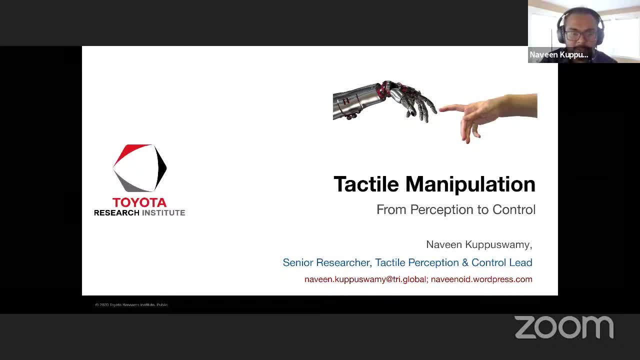 If I can. Oh, there we go. The participant view. Okay. So yeah, feel free to throw up your camera and do interrupt me whenever you want. So, as Russ mentioned, my name is Naveen Kupuswamy. I'm 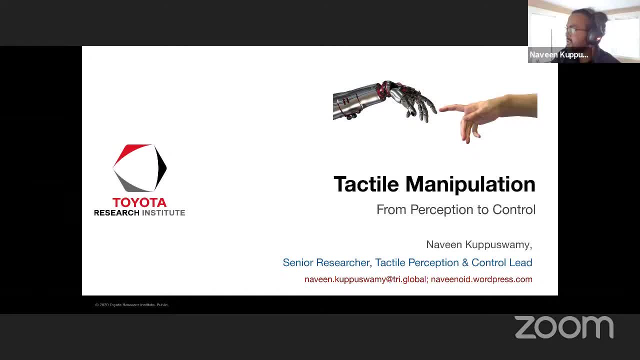 a researcher in the Toyota Research Institute, part of Russ's manipulation group. Before I even get into the talk, what I want to, at the outset, tell you is the aim of this talk for me is very simple. I want to tell you that I'm a researcher in the Toyota Research Institute. I'm a researcher. 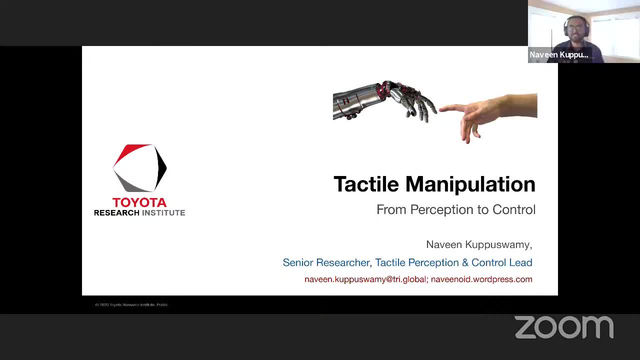 I want all of you to go home with just one single message in your heads: Why not incorporate a tactile sensor into your problems? So what that means, what all are the ways in which you can incorporate such a sensor that you're going to try and break down through this talk And right. 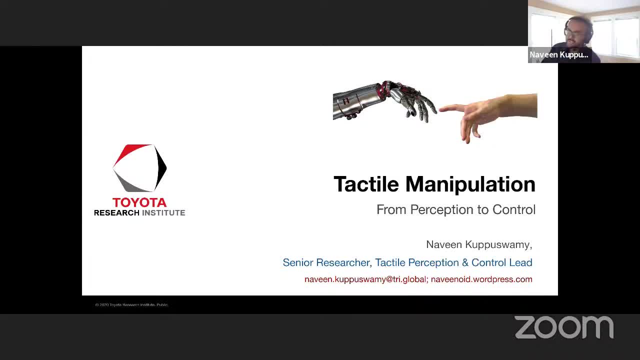 at the outset. I can already tell you there's some little biases which I will introduce throughout this talk. One, of course. I'm going to cite some examples which I personally like and I personally chose for didactic purposes, So it doesn't necessarily mean they are the best. 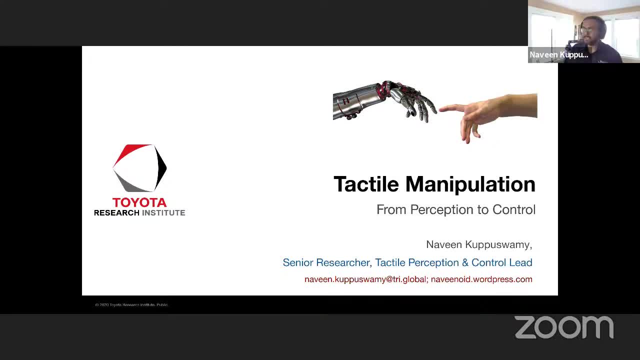 examples in literature. I've also kind of curtailed examples to fit our lecture duration so that we can actually dive into a couple of them. I will, of course, bring up some of my own examples, and I will often be citing some examples from the leading faculty at MIT, simply because I'm 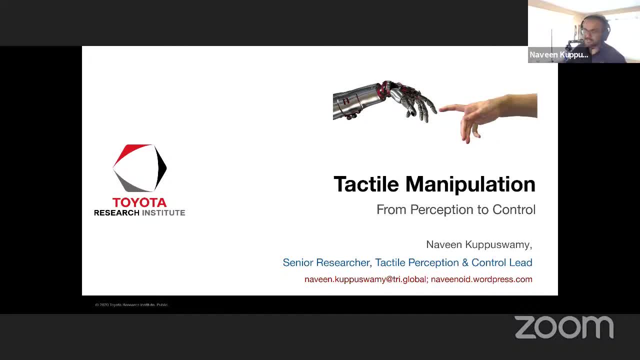 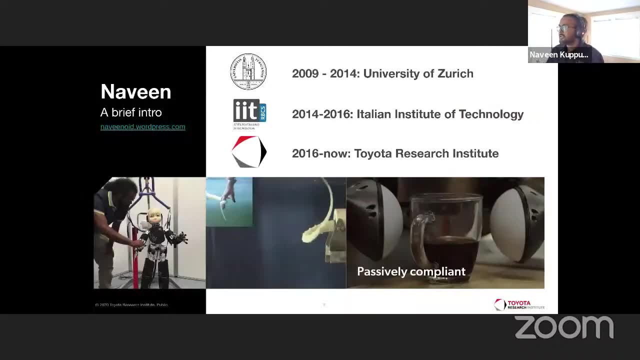 most familiar with a lot of their work And, as Russ said, they are just down the street from where I'm from, So I'm going to start by citing some examples from the leading faculty at MIT. So, based off of what's been presented throughout theEnimportant有沒有 and the 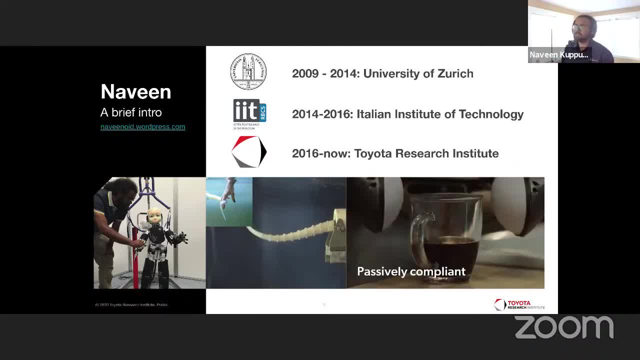 colleagues at MIT. you can see from the way I've talked about the level of interoperability that our offices are, although we're all sitting at home right now. So let's start forward for about a minute. see, right in the middle of your screen is this soft octopus gripper which has tendons going. 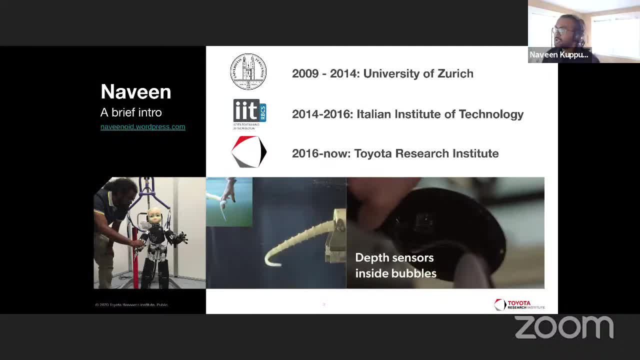 through this structure made of silicone and it's meant to be an underwater robot. I was a postdoc for a couple of years at the Italian Institute of Technology, where I worked on the iCub humanoid robot, which is this little guy you see on the left there, and lastly now at the Toyota Research. 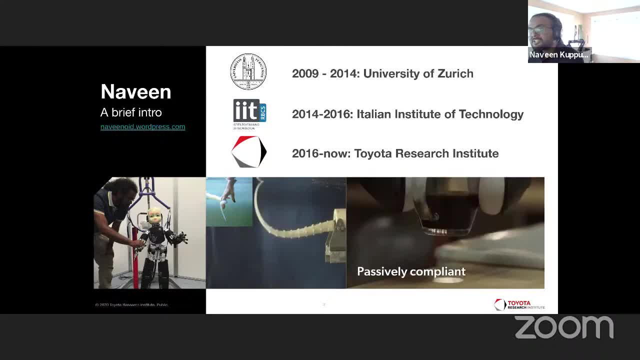 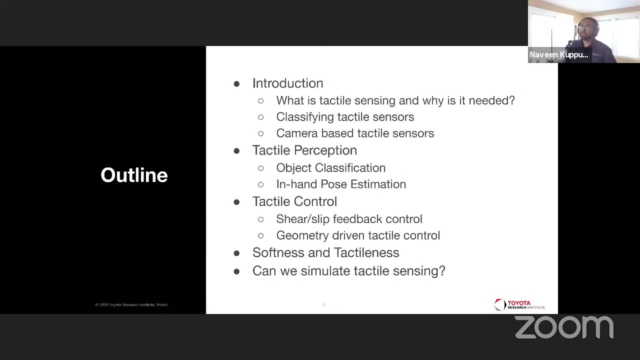 Institute, I have this incredible opportunity to work with some of the world's leading experts in several topics, but in particular, with some really solid experts in soft robotics and in designing and constructing complex soft tactile sensors, in this case called the soft bubble. So I wanted to quickly give you an outline of what we can expect from today's lecture and 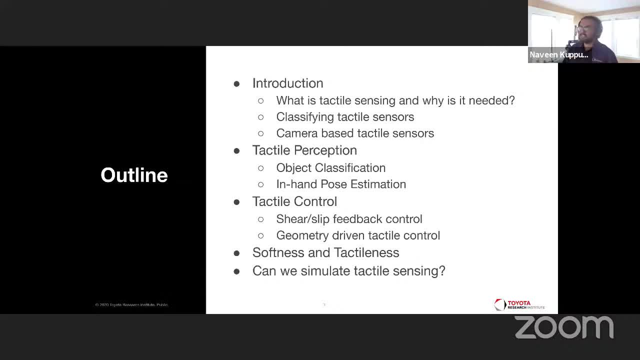 we'll dive deep into some examples. So the first part. let's break down this question which I personally find a lot of roboticists don't really quite grasp, which is what is tactile sensing and why is it needed? So it's not that they don't grasp it, they see parts of the puzzle and sometimes, looking at, 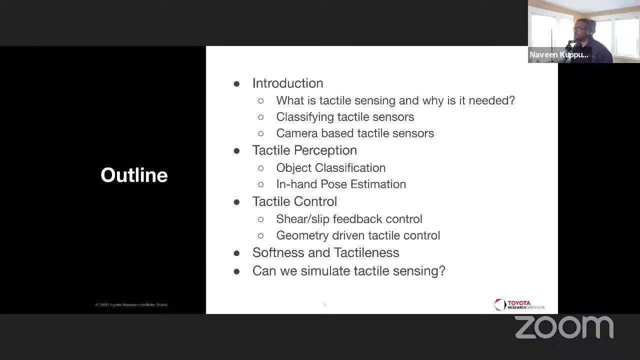 the whole really helps. Specifically I want to try and classify tactile sensors and today's lecture, for instance, comes purely from a bias that I carry as a control and control engineer, getting into robotics, which is I'm not really a sensor design person. so today's lecture will not get too deeply into the electronics of sensor design, into the transduction and how what. 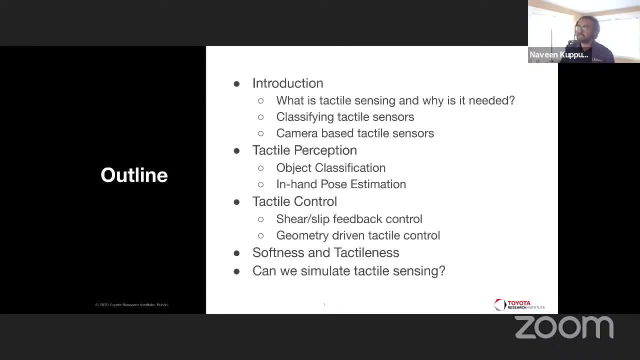 are the properties a tactile sensor can capture, etc. that that is not really what I'm going for here, and I will also reflect a distinct bias towards my favorite type of tactile sensor, which is the camera based tactile sensor right there, and we'll dive deep into that and what that entails for. 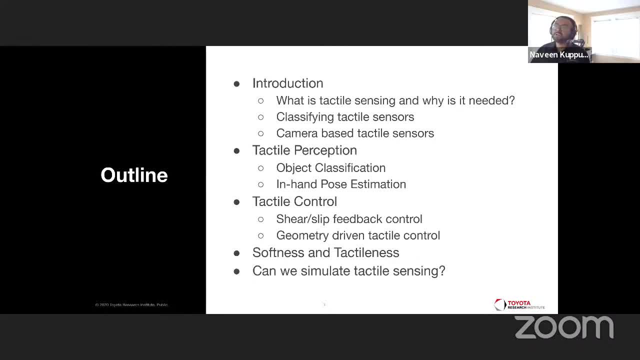 manipulation. Next, of course, I want to pick out two problems in tactile perception which I find really interesting, which I've also consumed some of my time in the recent years and I'm going to pick out a couple of examples in detail for doing some kind of tactile control and I want to throw into outlook. 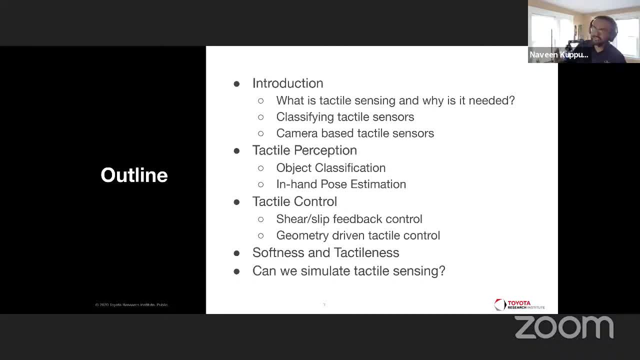 type questions, which is one: what does it mean to think about tactileness in a world where we have robots which are getting soft? and lastly, of course, the question which everybody who attends this lecture often poses: can we simulate this thing and can we stimulate it with drake for 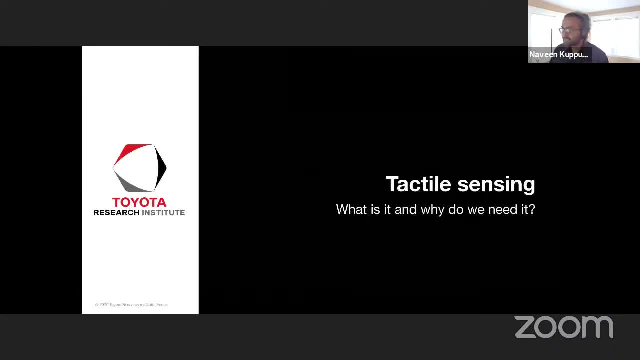 instance. so with that let's begin. so I can't quite see all your faces yet, but if someone feels like pitching in, let me ask you the question: what is a tactile sensor for you, and why do you think we need it? are there any? is there anybody who wants to throw up some guesses? 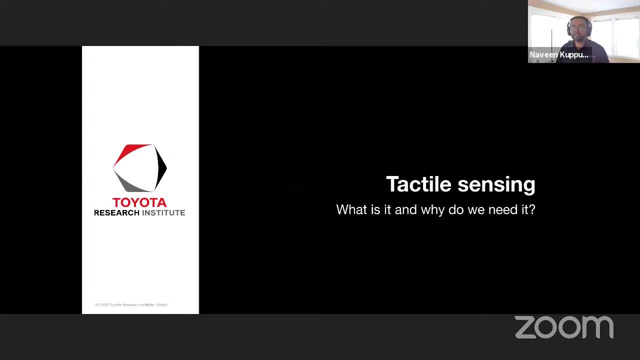 if not, I'm going to ask terry or meng to jump in. what is a tactile sensor for you? you can tell me whether I'm in contact or not. so some kind of sensation of your contact state. all right, maybe the texture and shape of your contact surface? excellent point. some aspect about 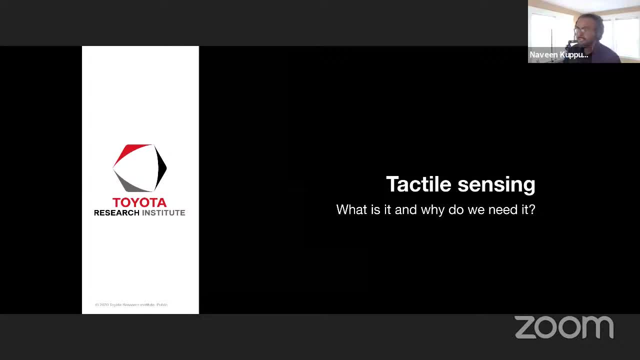 the, the geometric features of the surface or the object being grabbed, and what you can do with them, of course, is from these two responses, gives you one spectrum, which is sort of behavioral level decisions. if it is this texture, do that action. if it is, if you have made contact in this way, 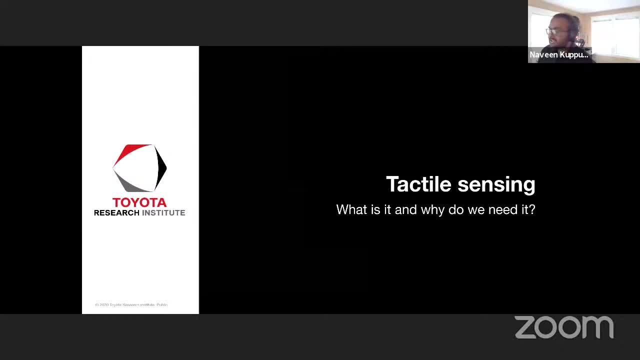 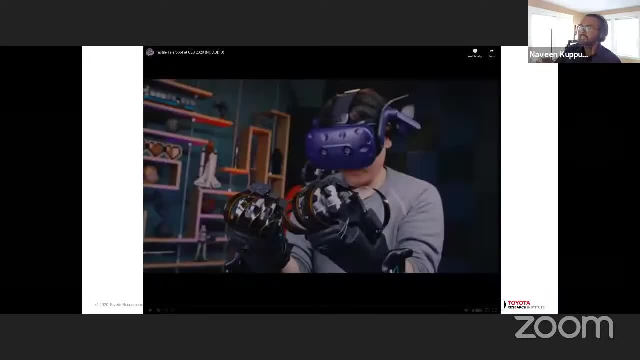 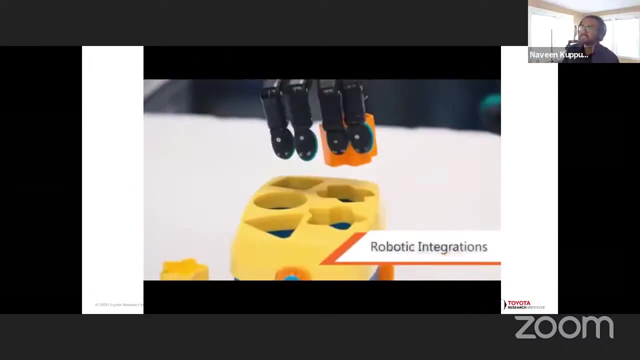 perform that action. so, as we tend to refer to that way of thinking it's, it's kind of, you can think of it as behavioral. but let's look at, before we get into anything, my favorite demo, and this is one of those demonstrations which, once you do it yourself, it really blows your mind. so this demonstration combines tactile sensing. 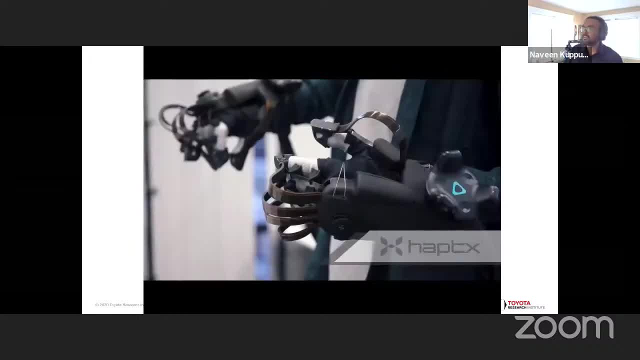 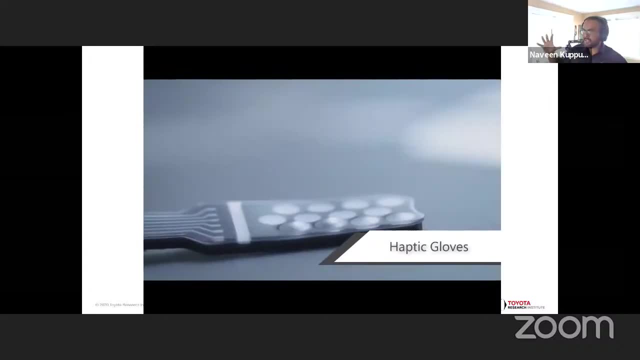 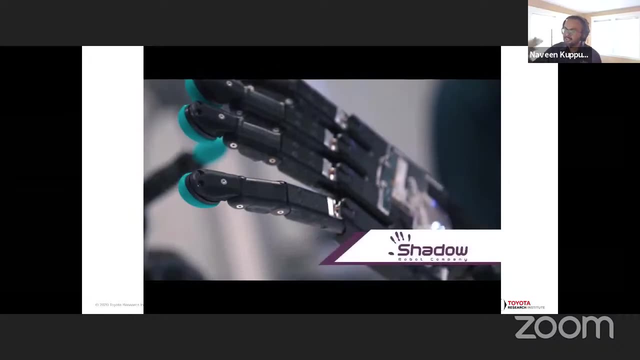 with a closely related area of haptics, and into this interactive demonstration, where people are having these haptic gloves, they're performing this complex teleoperation maneuver, with or without VR goggles, and you have the state-of-the-art dexterous robot hand built by the shadow robot hand company. 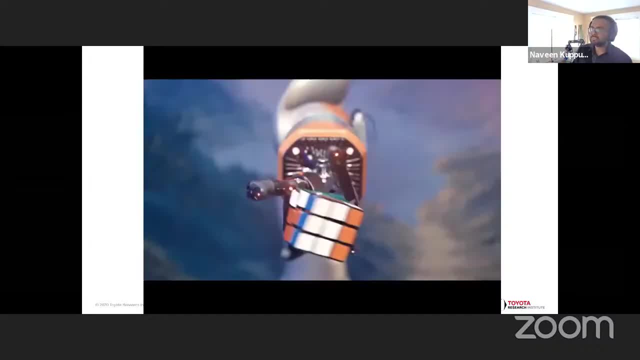 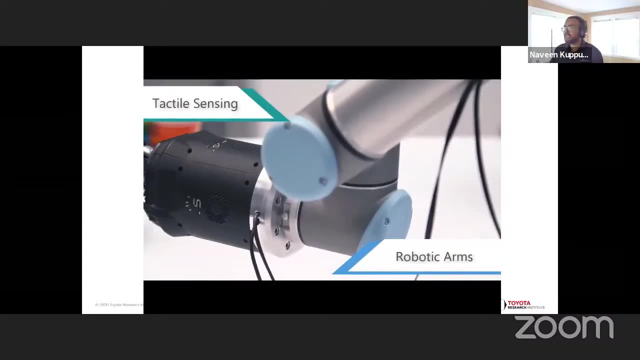 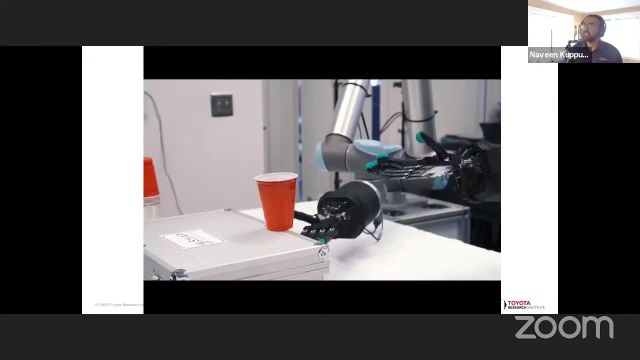 and a very interesting tactile sensor placed at the fingertips and, by the way, this hand is capable of pretty awesome actions. these sensors are from sin touch and through a combination of all these aspects, a user is able to experience what it feels to go perform a complex tactile manipulation. you 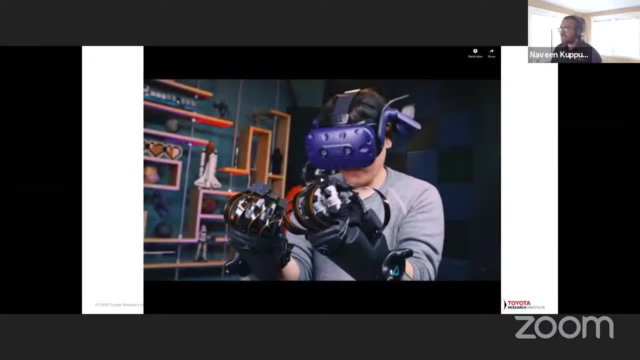 may have seen some version of these also being tested out in major demonstrations. you you had Jeff Bezos play with one of these and everybody blew up about those. in fact, my team even flew all the way out to California just to try out this demonstration, because it's a very visceral feeling of what does it feel for a robot? 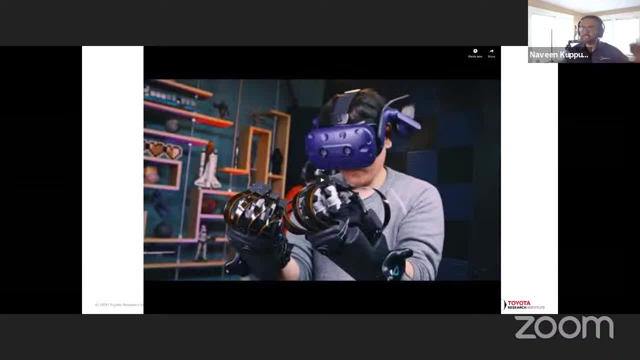 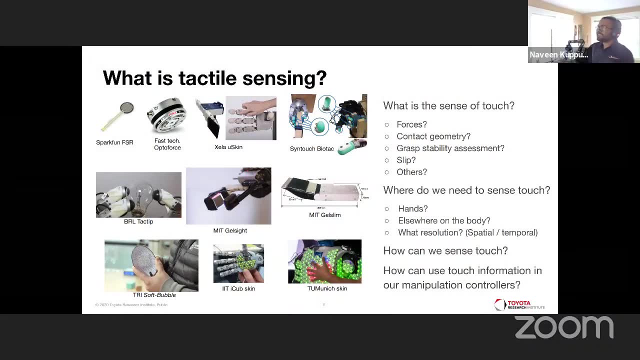 to touch something. you know exactly what it feels for you to touch, but what does it feel like for a robot to touch something? so now let's unpack this question now. what is the sense of touch? now, touch means so many different things. at the outset, I'm already going to tell you something. 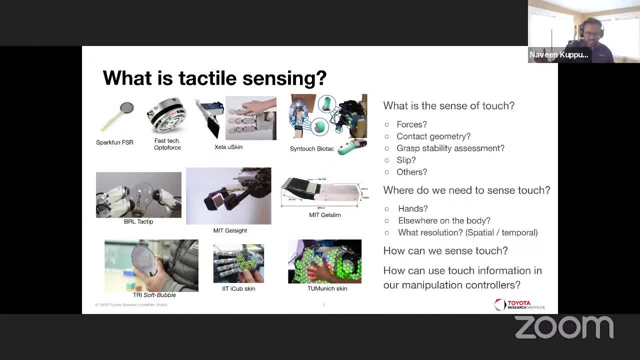 when we talk about cameras, for instance, in vision-based perception. it is a pretty huge field. there is a massive number of people working on vision-based perception, but what a camera is is a lot more straightforward. object of definition, for instance, a camera is some kind of sensor. 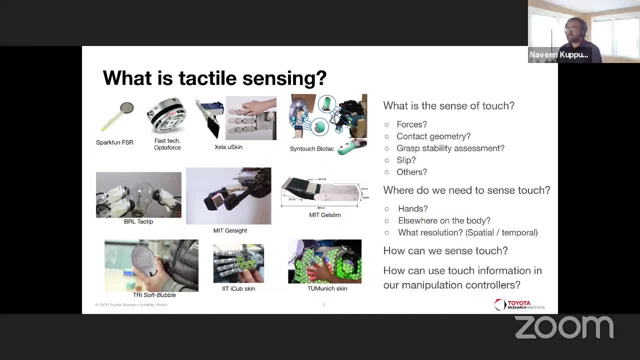 which is working on the electromagnetic spectrum and which is giving you information in some form which you can process and understand what's going on in the scene, whereas with the tactile sensor it's not even one single phenomenon. there's a whole multitude of phenomenon which are being captured. 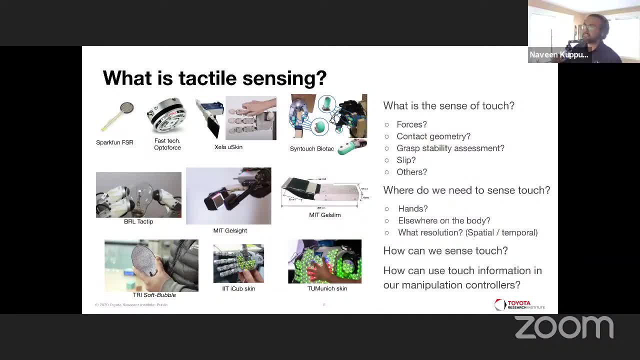 and therefore what a tactile sensor is, is so closely tied in with what is the transducer which is embedded inside this tactile sensor. so what is the modality which we capture? so I threw in a few examples. is a tactile sensor something that captures forces, something about geometry? it's 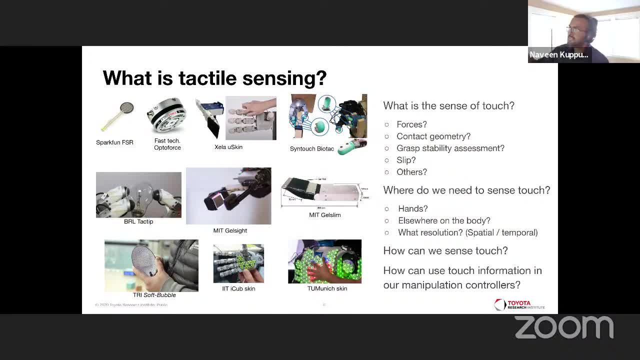 just like what Meng suggested is it's with the forces, we can already throw the question. does it just tell me on off that contact happened, like Terry suggested? is it something which can give me some sense of how stable is a grasp? is it something which can sense slip, which is some kind of relative motion? are the 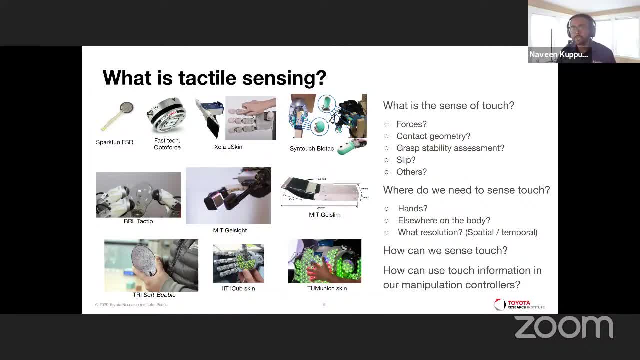 other phenomenon. maybe a tactile sensor can tell you the temperature of contact, maybe it can sense some other properties about the surface above and beyond a single time slapshot can yield you and intentionally I have thrown a multitude of of sensors out there and if you notice a little thing right on top left, 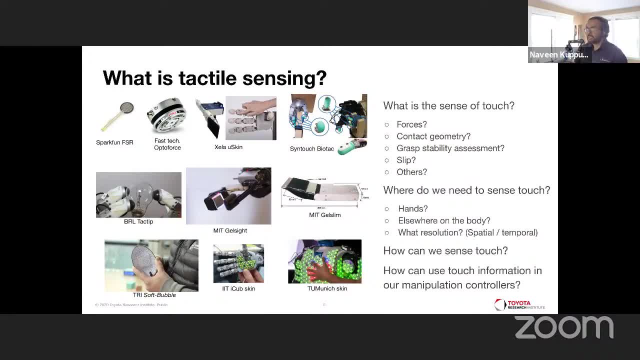 of the spectrum, I have something as simple as the humble FSR. a lot of hobby roboticists play with these four sensitive resistors of that form. all they are is a variable resistor where the more pressure I apply, through whatever electronics techniques, that pressure change is conveyed into. 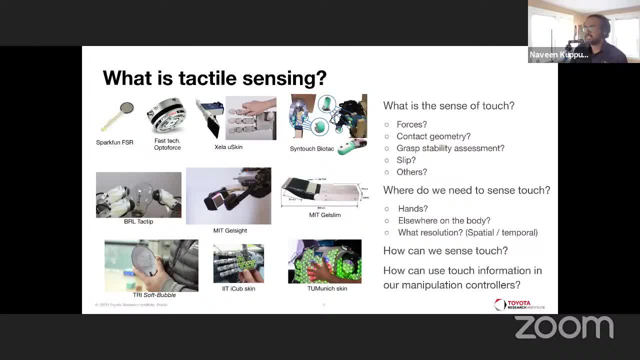 a voltage change or other forms of signals which can then be read out. so that's, I would say, one very simple kind of sensor in one end of the spectrum. next we have our our most well-known force torque sensors. you covered some aspects of force torque sensors in your previous lecture. you could say a force torque sensor is also a. 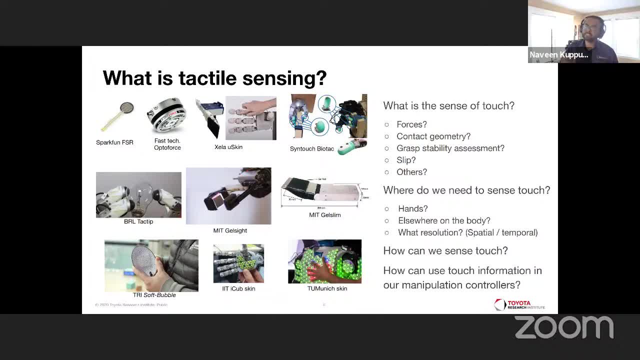 tactile sensor and we can talk a bit about where is it not a tactile sensor in terms of what are the limitations of force torque sensor for a complex tactile interaction. and then you have a bunch of examples, everything going from industry-grade products such as the zela u skin, the muskin, the sin touch, biotech, which was used in the demonstration. 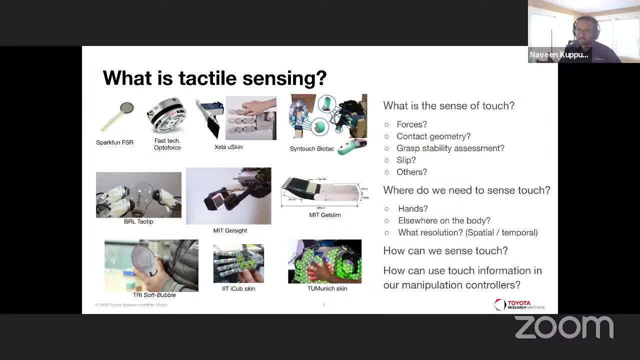 which you just saw, and then the brl, which is the Bristol robotics lab, stacktip and MIT's own gel site and gel slim, and then you have the soft bubble, the work which I am currently doing at TRI, and then comes the, the last two, which I want to throw. an extra question: where do you? 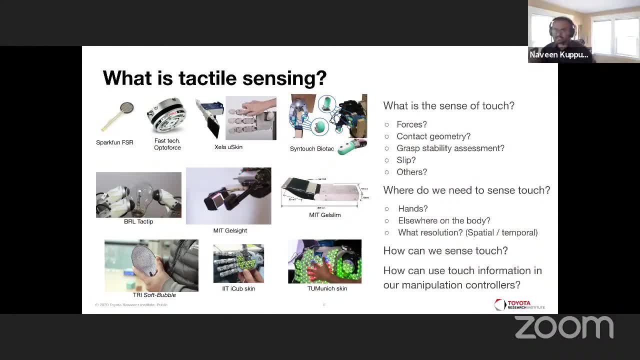 sense touch. do you want to sense touch on your hands, that is, your gripper of your robot? or perhaps do you want to sense touch everywhere, anywhere and everywhere on the body? and then also comes the question: what is the resolution with which we are talking about for this sense? 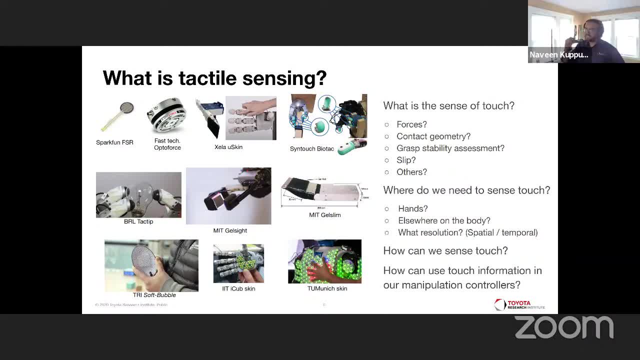 of touch, whether it's forces, geometry, slip, etc. there's a spatial resolution aspect, which is how finely it's distributed over the geometry of your robot itself or of your structure itself, and then what is the total resolution? how quickly is a tactile sensor able to tell you something happened? 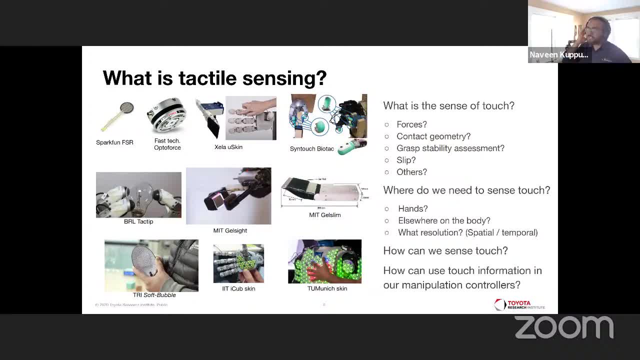 so some of these questions have direct analogies, of course, in the camera-based perception world, but nonetheless these are important questions to assess the different types of tactile sensors. so underlying all of these questions is, of course, the, the electronics transduction. a question which is: how can we sense touch? how are these phenomenon conveyed into some form of electronic signal which? 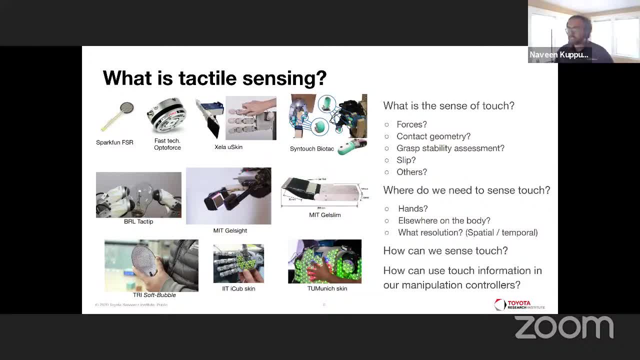 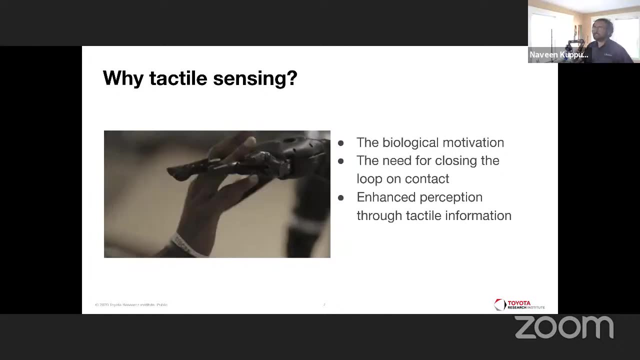 we can process and, as I said, we will not really get into that too much today. but my more interesting question is: how can we use this kind of touch information in our manipulation controllers? so, having said that, let's ask the question: why tactile sensing? and there are three ways in which I would like to. 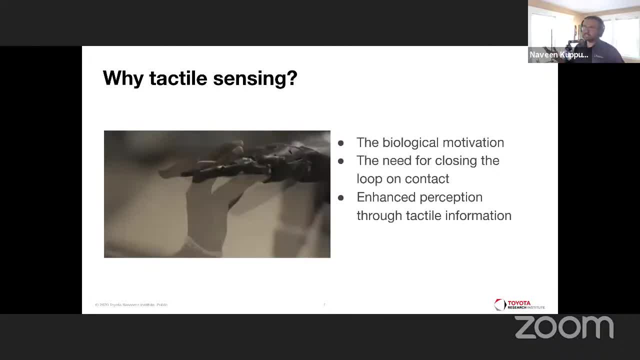 present the argument for why tactile sensing. the obvious case is there is a biological motivation. pretty much every living moving creature around us is able to sense some form of touch, is able to sense some form of contact, and especially if you take something as advanced as the human being. 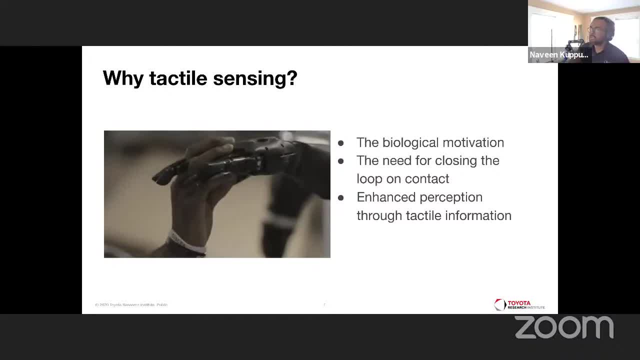 we sense a very powerful form of contact, so we'll understand that. next, there's, of course, the need for trying to close the loop on contact, and I'll explain a little bit about that statement. and lastly, perhaps our tactile information can give us an enhancement of the perception. information: 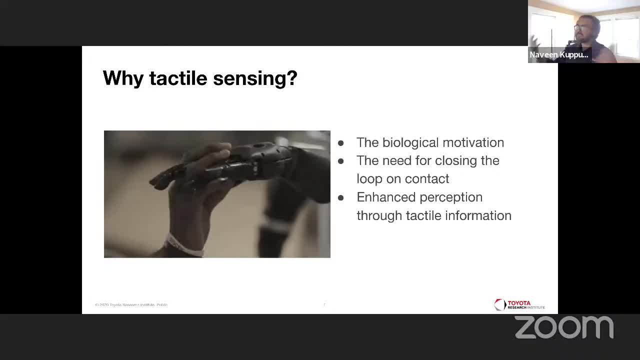 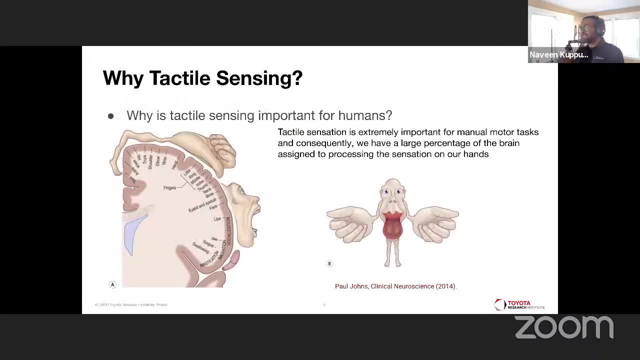 and keep in mind I'm saying you may use other forms of perception all the time, but tactile information can only enhance that perception. so let's start off with this creepy image here, which is from a well-known neuroscience text. I don't know if any of you have seen an image. 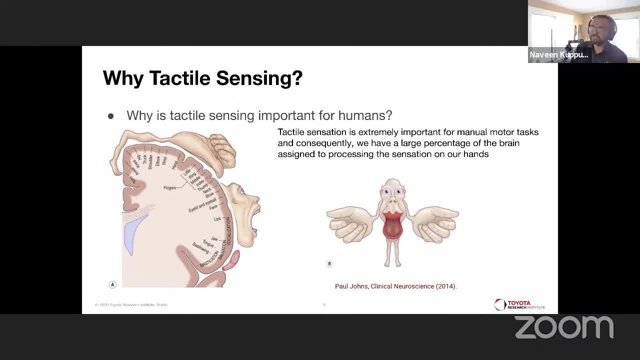 like this. what this image is doing is trying to represent the quantity of your brain matter which pertains to each of these organs, and that scaled image on the right is, in fact, literally showing how much of your brain matter is devoted to you understanding the sensations coming in from these parts of the body. note that this. 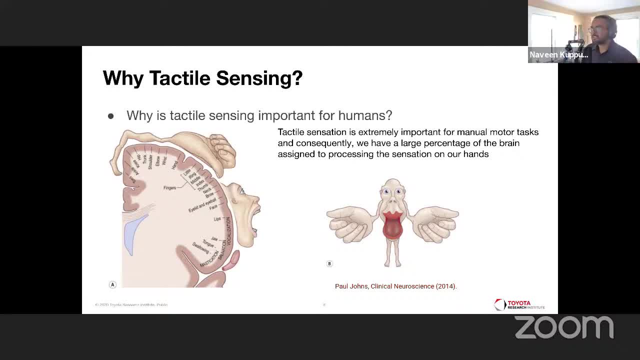 is not quite about the control. this is about processing the sensory information. so, as you can see, a huge part of our brain is somehow focusing on what our hands are feeling. there's, of course, your tongue and your lips, and your mouths too, because feeding ourselves is a 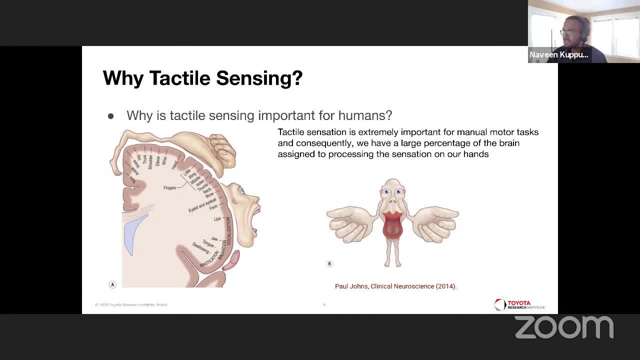 very important human activity, and vision is also an incredibly powerful and incredibly important human activity, but in a sense it intriguing that there's so much brain matter devoted towards tactile sensing, and I suspect, as do a lot of people, that it comes down to the fact that tactile sensation is a very complex 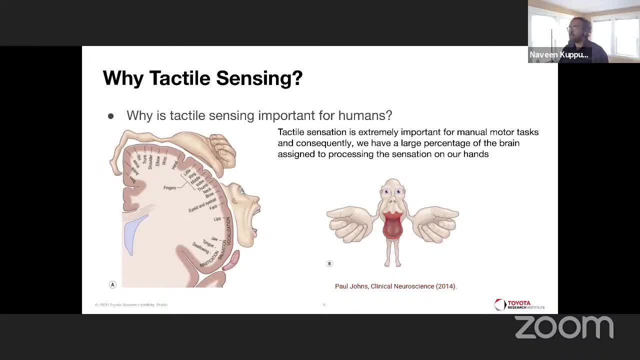 phenomenon which involves several possible modalities of sensations, and conveying all of that into meaningful information for control is really what all this brain matter is perhaps doing. And Naveen, the homunculus is just about the sensory cortex. yeah, and the 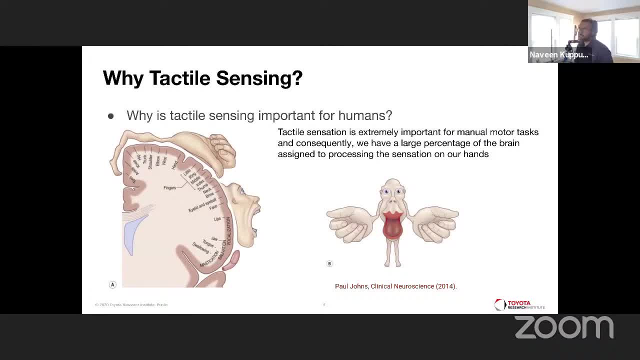 so the visual cortex is a whole? it's not. yeah, yeah, this is just sensory cortex and the visual cortex is massive by itself. yeah, Yes, yes, yes, not to not to say that vision is not as important. 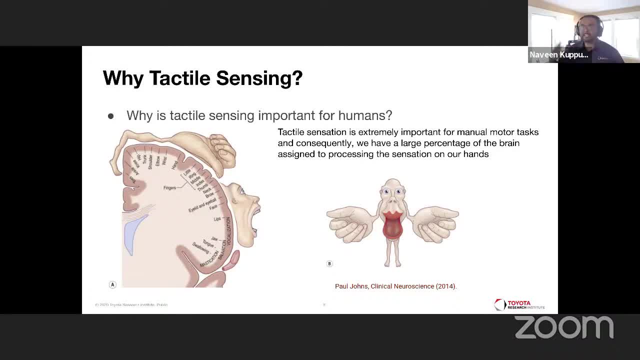 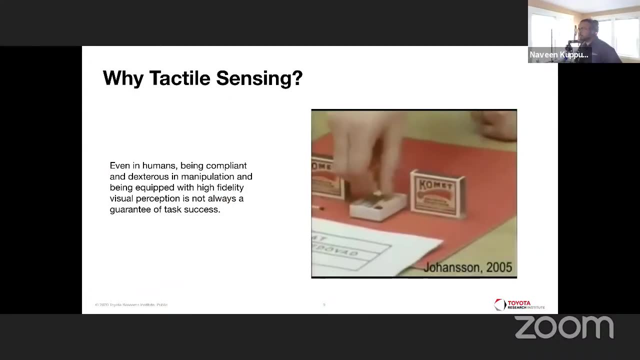 in fact, this is more about the understanding where your eyes are looking at, or something not so much about what eye is looking at. So yeah, but thank you for the clarification. So now here's a very interesting demonstration. This was from 2005,. this particular experiment. 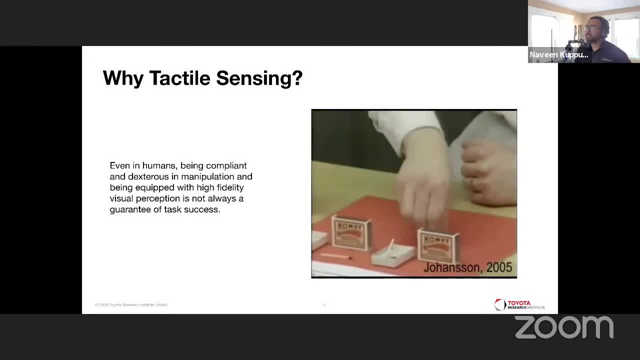 Now, right in our first lecture we had covered the topic of or. in Russ's first lecture he had spoken a bit about what's the advantage of having these soft, underactuated grippers In the human hands case. what if the fingers were soft and compliant? 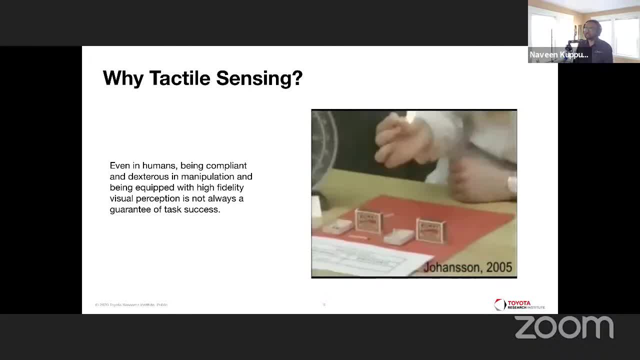 So in this case this person has been locally anesthetized in order to not convey any form of tactile sensation. The person evidently has some kind of nontypical sensation from the fingers. I'm not quite sure how they managed that, but essentially the challenge here is: the person can 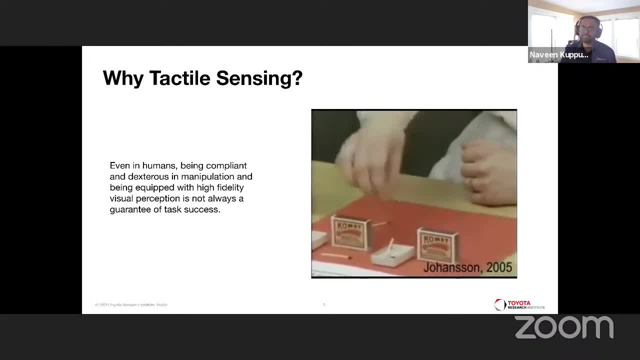 see, the person can control their hands. but the person cannot perceive tactile sensation, and they were asked to perform these kind of tasks. Now the person succeeds. this is clearly telling you that our vision is amazing. our brains are incredibly good at trying to adapt to a certain 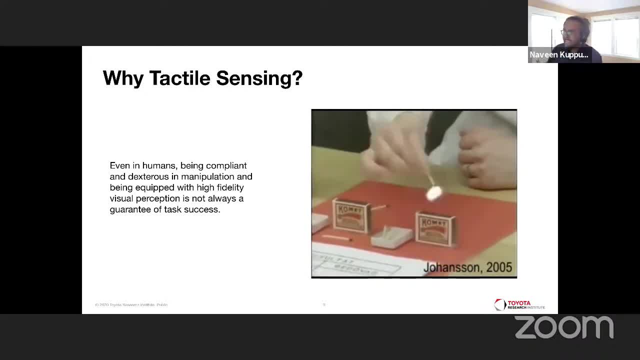 situation such as loss of the sensory sense of modality, and yet person fumbles like crazy in what was seemingly an effortless task for most of us. So just taking out a matchstick and lighting a little flame. Now, an equivalent analogy, I'm putting this: 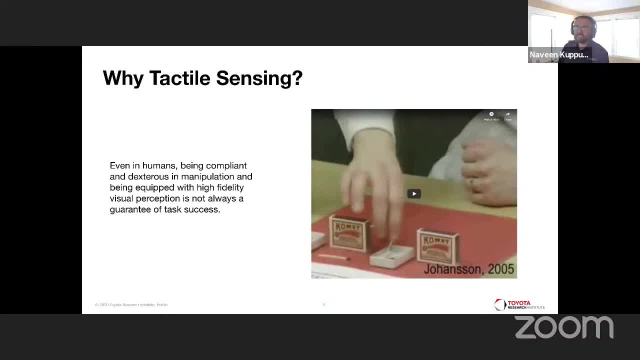 especially for all the people in countries which experience strong winters- is you go out in winter, you suddenly have your fingers frozen, stiff, and it becomes really hard to do otherwise seemingly mundane tasks with your fingers when you're outside without your gloves. So in other words, being compliant and dexterous in manipulation and being equipped with high 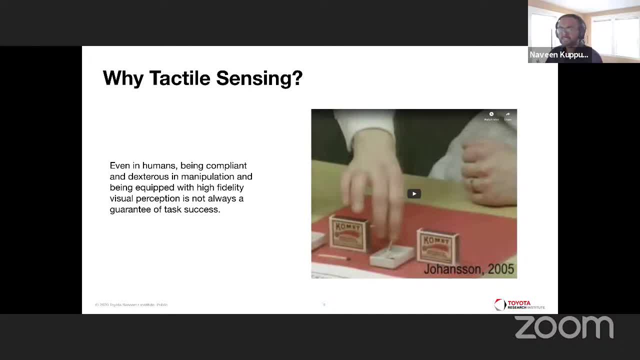 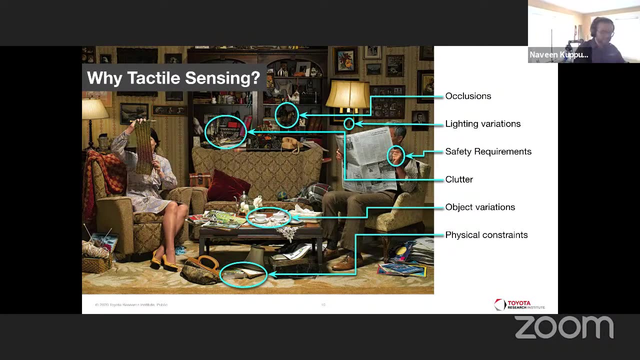 fidelity. visual perception is not always a guarantee of task success. So what is this sense of touch and why does it seemingly help us in this example? Now, let's now jump outside humans, because humans are, of course, a really complicated case, And let's just think purely from the perspective of a robot confronted with the 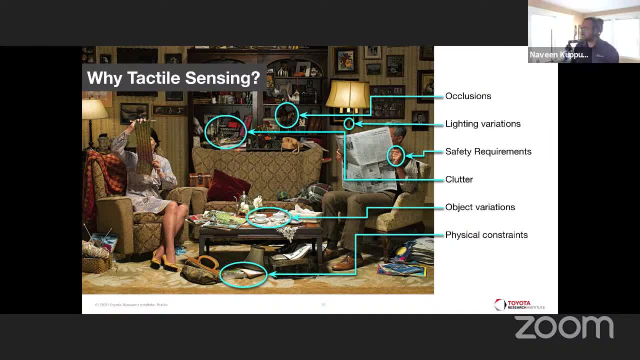 average home. So a lot of of us in the field of manipulation are interested in putting robots in our homes. So what are the typical situations in homes and why does that lead to confounding our sense of perception? So I have a list of issues here and I'll walk through them. Occlusion, which means you can't see a thing. 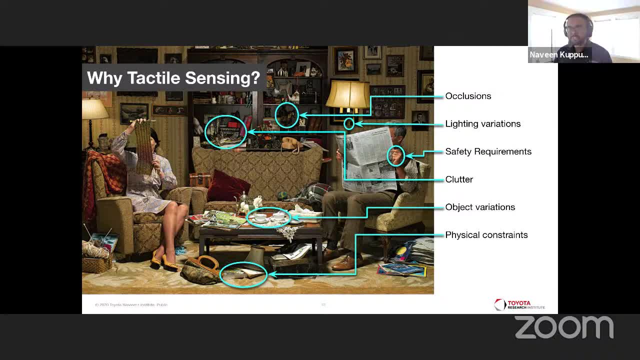 which is blocked by another thing. So if you were perhaps interested in spotting a very specific object and trying to perform some tricky manipulation with it, if you occlude yourself, you don't know what exists behind that. Similarly, there's lighting issues in our homes. We are not sitting in our labs with our perfect light sources and therefore lighting issues can tend to confound a vision based manipulation system. 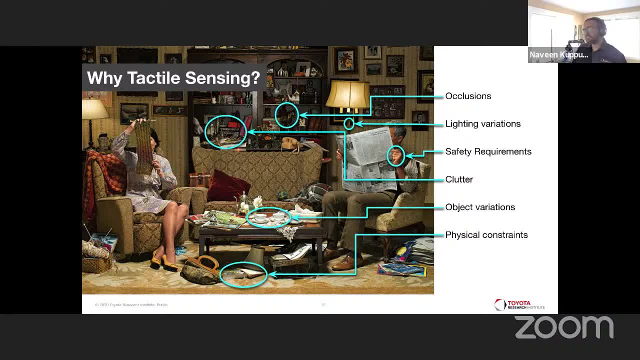 Safety requirements When you're working at homes. if there is a person near you, you better be careful in how you're behaving, Take care in order to not cause any harm, And perhaps looking to see if you touch something may not be the fastest way to respond if you touch something. 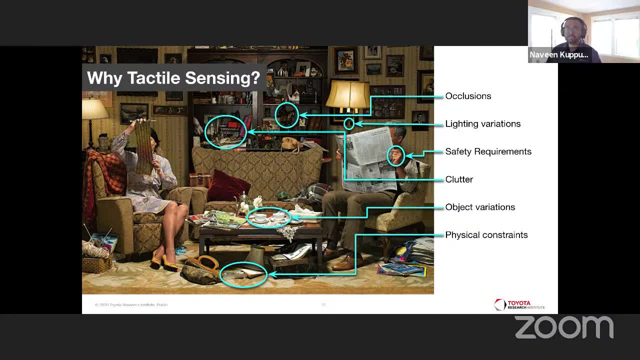 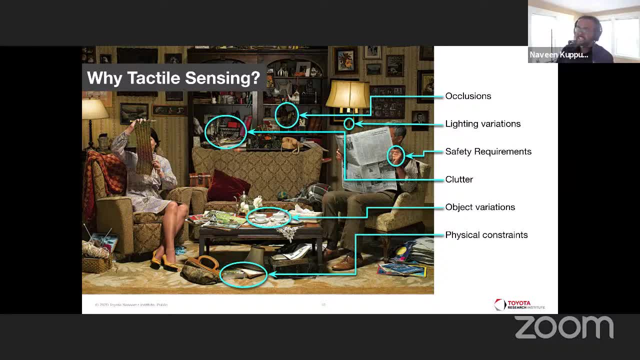 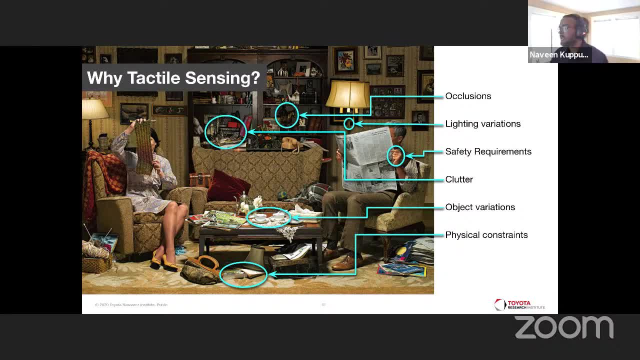 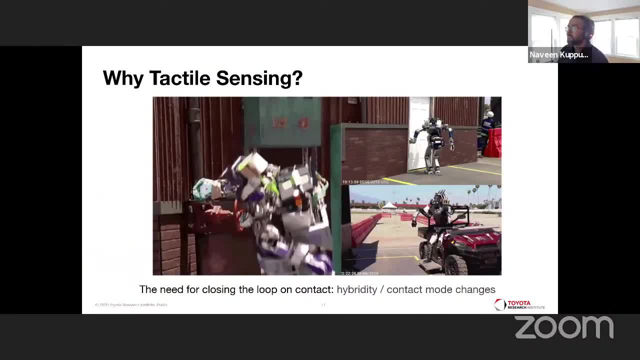 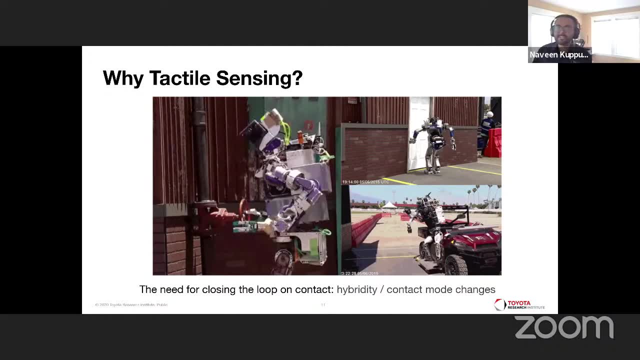 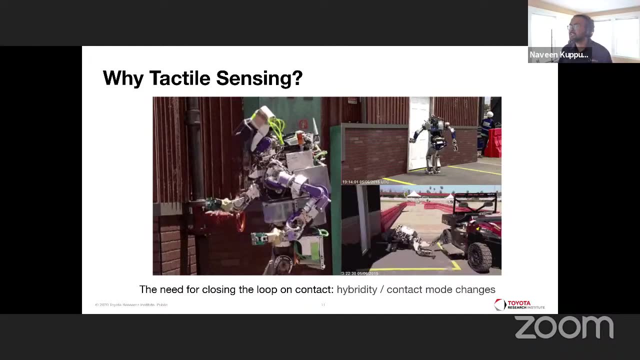 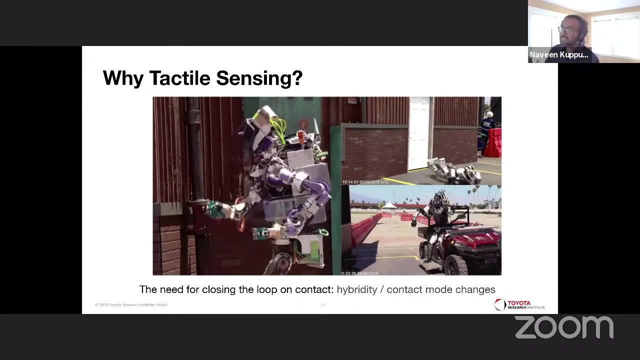 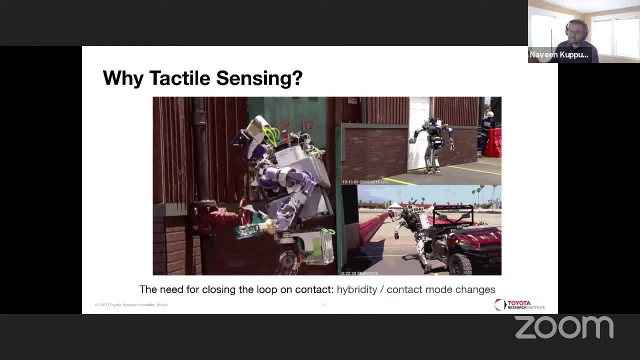 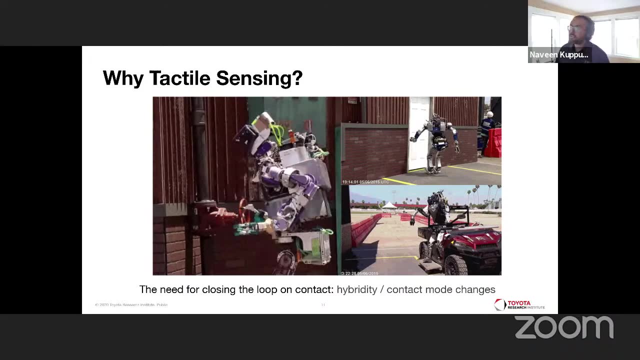 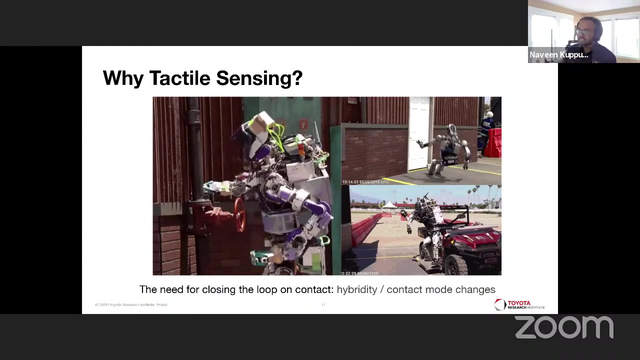 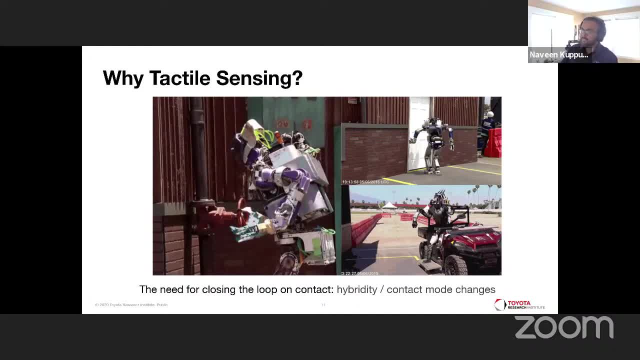 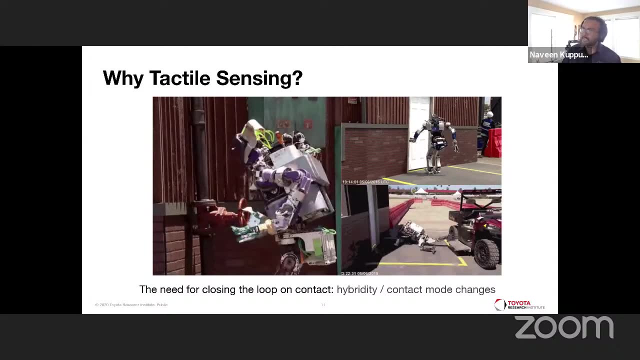 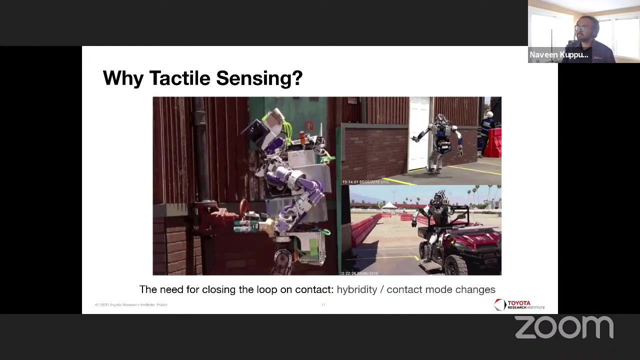 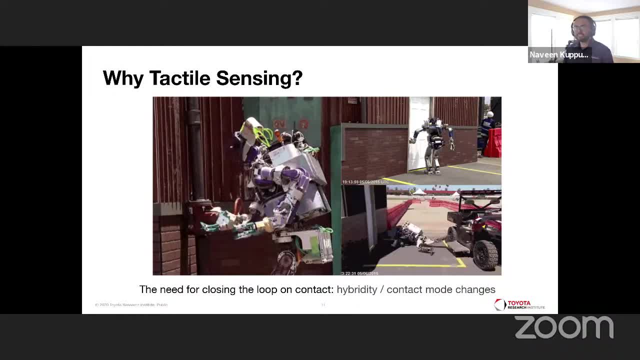 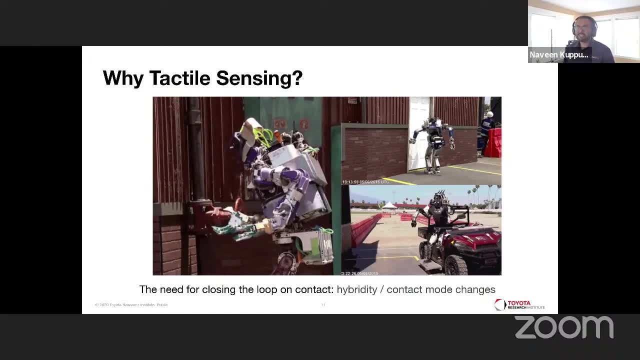 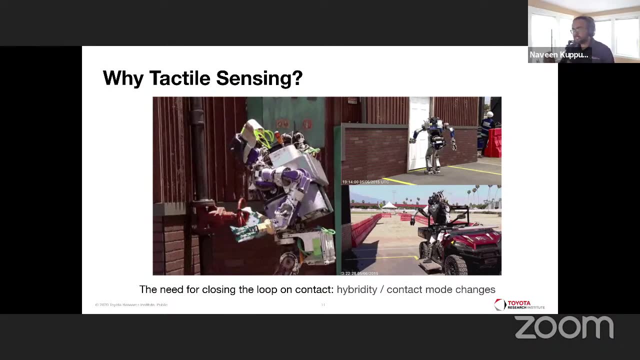 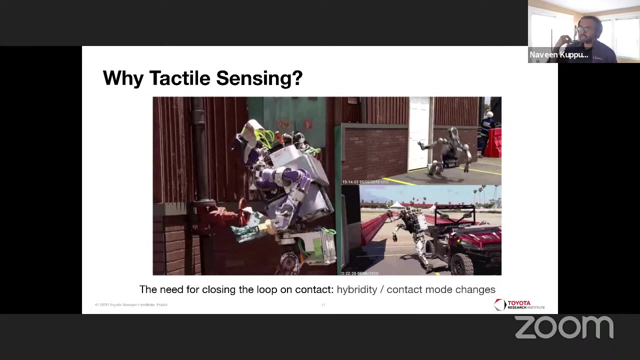 you're making these complex transition from having multiple parts of your body in contact- for instance, the robot's rear is on the seat, the feet are on the ground, but then you're suddenly trying to lift off and moving into a state where only the feet are in contact and not sensing. this transition between multiple locations of contact to a fewer set of contact locations often leads to your controller getting confounded and it then leads to predicting what the robot is doing. 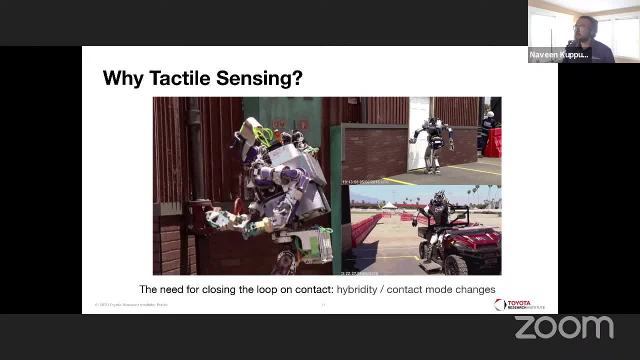 erroneous trajectories for tracking, or it leads to other kinds of complications where the robot then misperforms, malfunctions and leads to some kind of catastrophic conditions. So this is an obvious need for knowing that a contract transition happened. I want to think about now standing on my feet. I want to think about standing on my feet and being balanced. 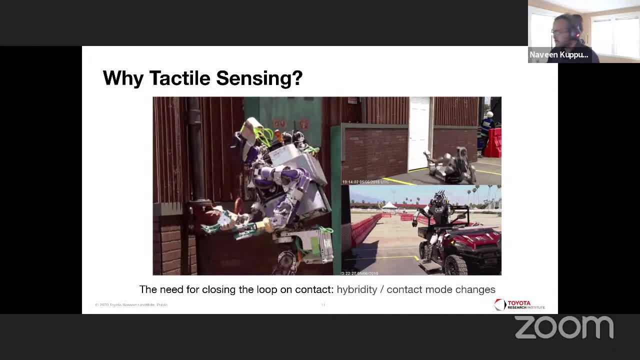 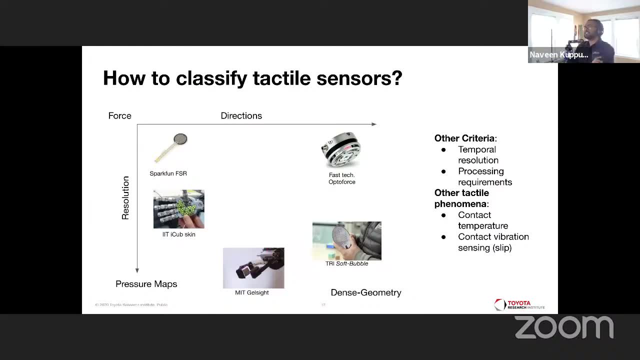 back there and then I can only move my hands and so on. So that's an obvious case for why tactile sensing makes sense. Now let's ask the question: how would you classify a tactile sensor? So I have thrown one form of classification. If you go, pull out the classic literature on tactile sensors. 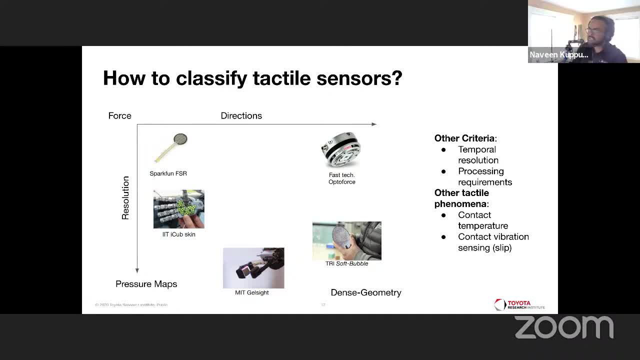 the main reviews. each of them talk about this classification in so many ways. You can talk about the classification in terms of the underlying technology. You can talk about the classification in terms of what are the actual modalities which are being sensed. but specifically, in manipulation, I want to 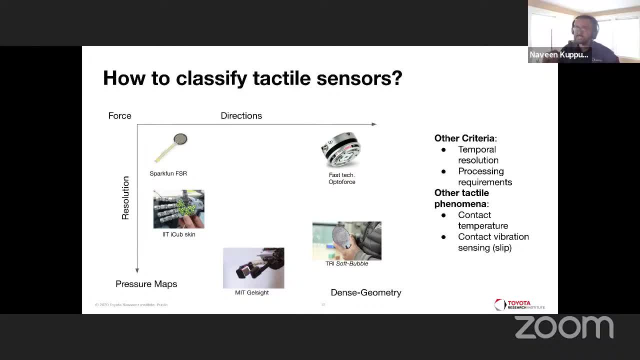 get your focus on this one spectrum which is, let's think, just about forces, the direction in which the force is sensed and the spatial resolution there, in particular, where we are sensing forces on some surface, on the robot, On the upper end of the spectrum, you 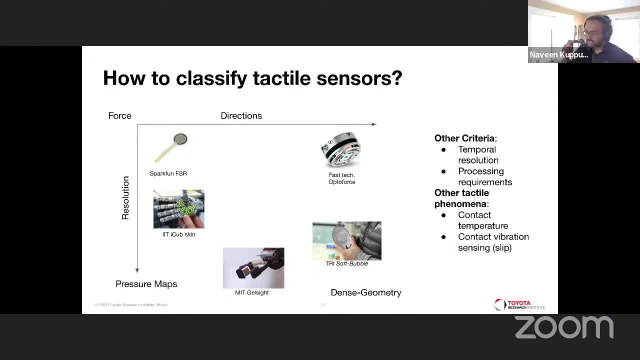 have these simple, humble FSRs, which are nice little pressure maps, as they're called. So you stick them on a surface surface. they capture the pressure with which external forces are being applied because an external body is in contact In the same axis. if you weren't changing the number of measurements, 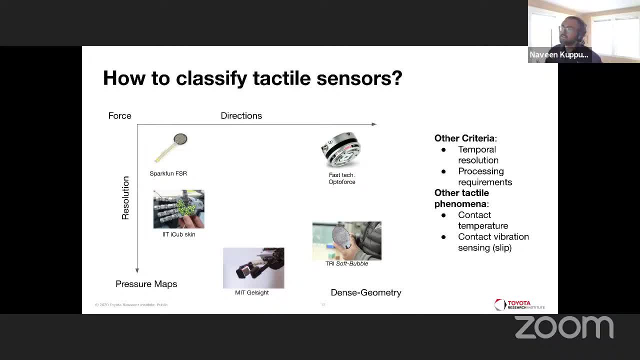 from a single point. you have our force torque sensor, which is able to sense all the way up to six different axes of forces and torques. So that's XYZ forces and torques in three different directions, And yet it's sensing all of those aspects from a single reference body. So we are 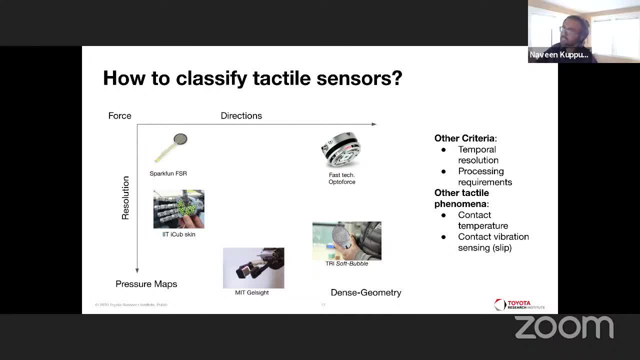 trying to sense what is the net external force or torque, as applied on the single body, in this case the sensor's body. Now, if you move lower on the scale- by the way, I'm not sure if you can see my pointer- Let me throw up my pointer. I think now it should be visible. Yeah, Okay, So on this end, 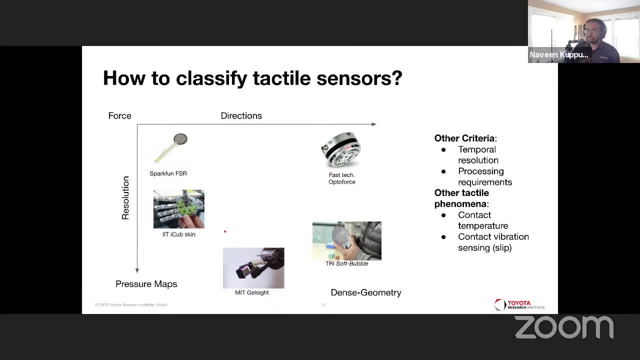 of the scale. you have something like this Dense pressure maps distributed all over the surface, like in the iCub skin, And on the bottom end of the scale you have the ability to sense at a very high spatial resolution, as well as in 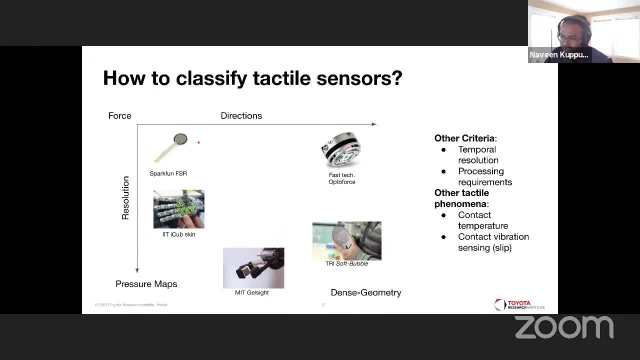 multiple directions of applied force, not just the normal direction, like these, which is through these so-called dense geometry sensors, which is what I would talk a little bit more about in a second. But just to be clear, we have other criteria. We have other criteria with which we can think about these sensors. One is, of course, the 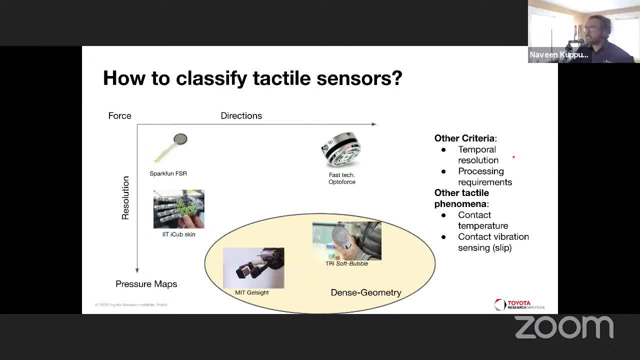 temporal resolution. so how frequently we are able to get updates the processor requirements for these sensors. So cameras, of course, come as a neat package, technology which give you this little cable by which they stream out information in the form of frames or whatever. Now, tactile sensors. 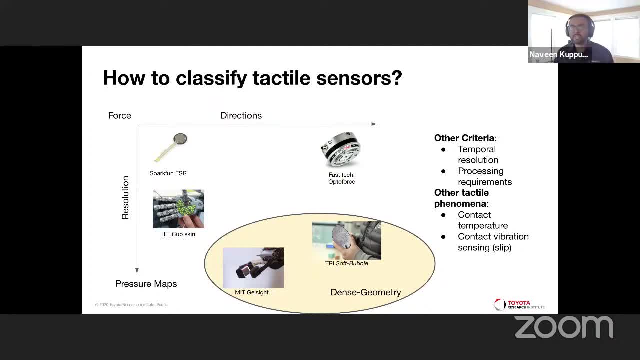 may or may not come with the associated processing embedded inside the packaging of the sensor itself. So sometimes you may have to do a lot of the processing to understand the processing of the sensor itself. So sometimes you may have to do a lot of the processing to understand the. 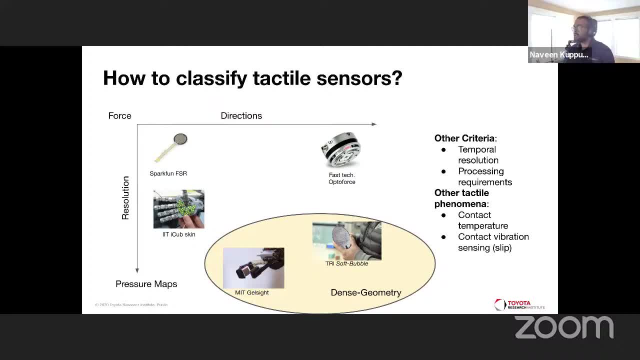 processing of the sensor itself. So sometimes you may have to do a lot of the processing to understand what happened from raw voltages or whatever. So that is another way to think about tactile sensors. And, as I mentioned before, there are other phenomenon which I'm not covering in this form of 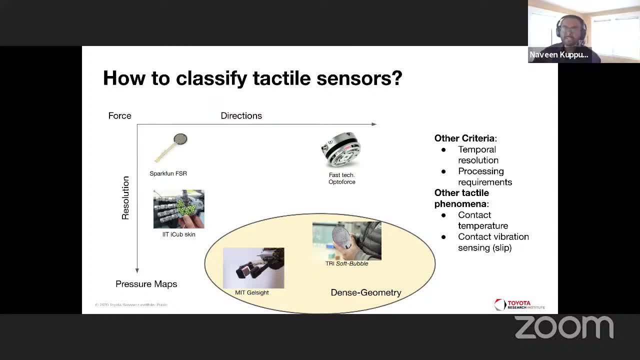 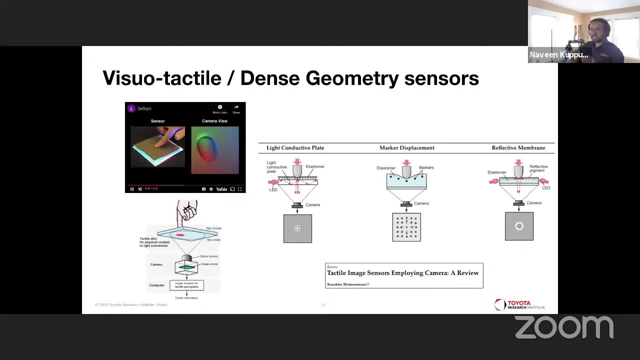 classification, for instance contact, temperature, contact, vibration sensing, which is also related to sensing slip. So those are things not present in this 2D plot right here. So let's talk very briefly about these visual, tactile or dense geometry sensors. So let's talk very briefly about these visual, tactile or dense geometry sensors, which now, indeed, is my favorite. 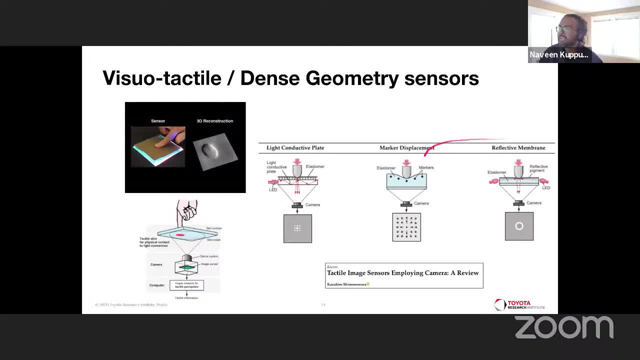 class of sensor. The video playing up there is the MIT GEL site, which came from Ted Adelson's lab, and it represents one of the classic examples of this new archetype of sensor. So the essence of this is well captured by this image right here. 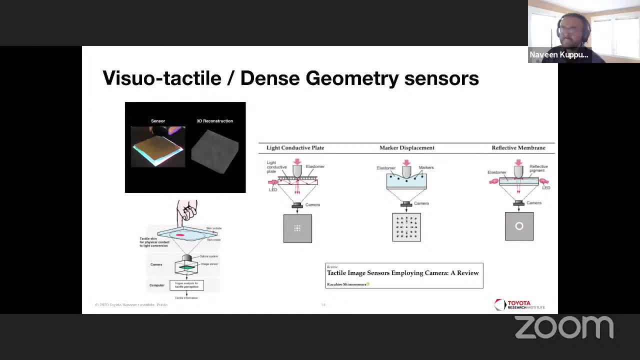 There is some form of external contact. Your robot surface is embedded with some kind of skin. So the essence of this is well captured by this image right here. There is some form of external contact. Your robot surface is embedded with some kind of skin. 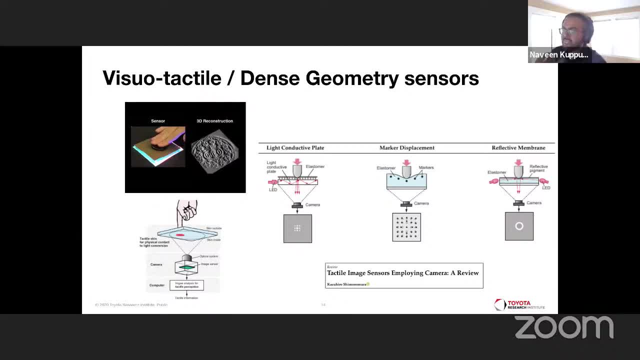 The inner surface of skin when it deforms, is being observed by this optical system with an imaging sensor. and then you have your image processing work sitting in a computer giving you tactile information. So the slight distinction is unlike an FT sensor or 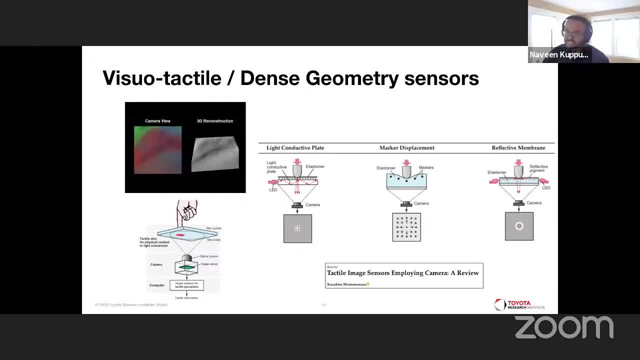 a pressure map type sensor. there is still quite some processing happening on your solution outside the sensor itself, But the really interesting aspect is, as it's said here- with a little typo, by the way- the image analysis part is completely vision-based processing, And that is something which we now have a better and better sense of. 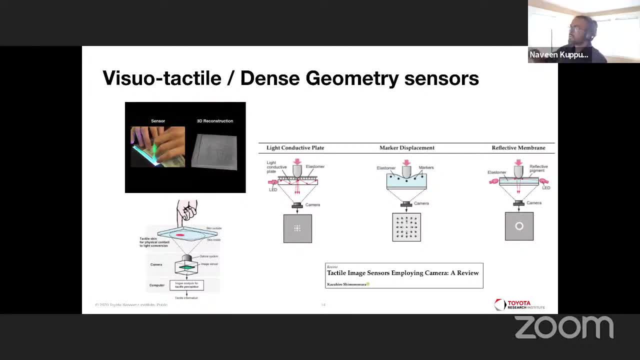 how to perform this kind of image-based understanding. Now, there are three broad techniques, as listed in this review, for performing this kind of an action. So there's even a fourth, which I'll talk about in a sec. So either you have a light conductive plate, 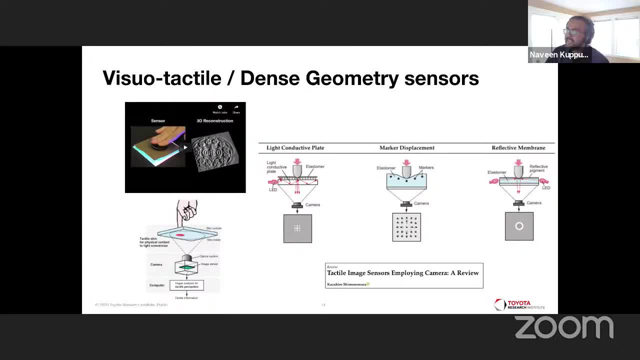 which is you have an internal light source- in this case this little LED, and a reflective surface which is facing inwards on an elastomer medium, which is a medium which can be deformed And once external contact happens on it, light gets deflected and you're literally looking at. 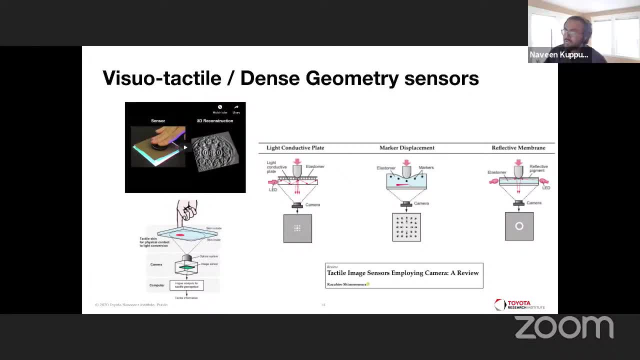 the deflected beams of light. The other form is: perhaps you don't care about deflecting light itself, You simply embed the surface with these kind of markers and you're looking at marker motion. and later in this talk we'll dig into what does it mean to observe motion of markers? And lastly, 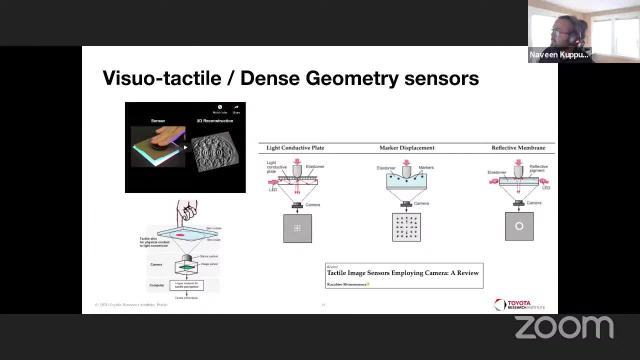 a variant of this format is to instead have this kind of reflective pigment which directly captures what happens when an external surface suddenly changes the patterns of reflection. Now, this is to say these are vision-based sensors which are not active, So they're not projecting. 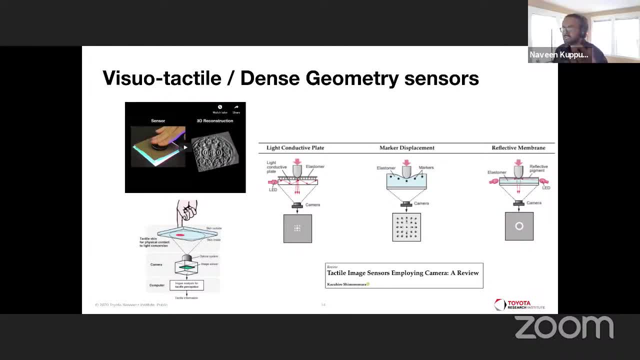 any form of patterns or et cetera. And now, of course, as you may have covered in your class on doing computer science, they're not going to be able to capture the image, but they're going to be pose estimation. they are these so-called depth sensors, sensors like the time-of-flight sensors. 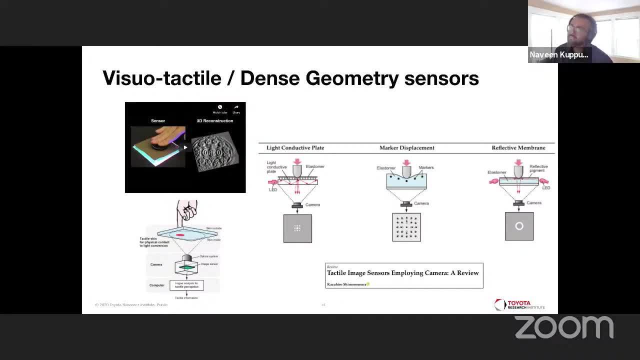 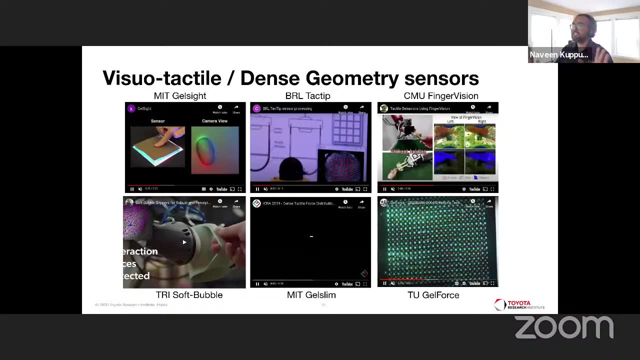 which can even directly measure the distance to a surface, And if you can embed one set sensor into this packaging, you also have a more direct form of measuring the distances. So here's a quick view of all of these key different types, in a way, And I've listed the 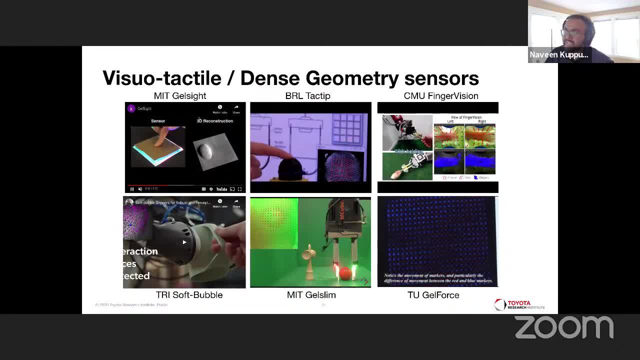 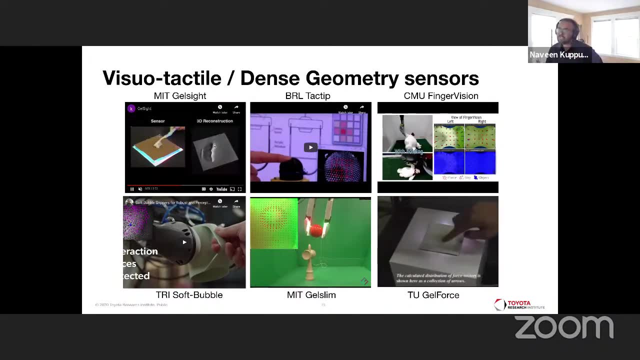 names of each of these sensors, Let's talk a bit about them. So there's the MIT gel site which has this reflective surface and it's stuck on top of this elastomer And you can see what the nature of contact is doing to the visual images coming out of the sensor. And by cleverly, 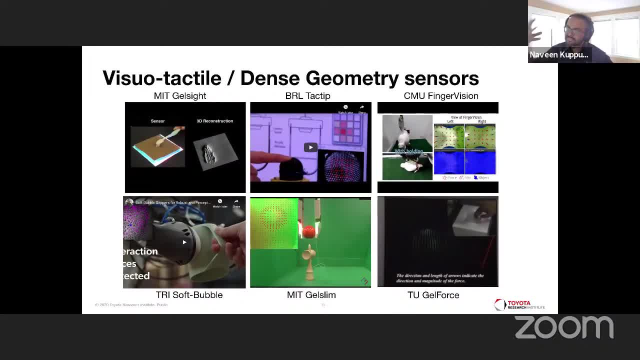 arranging light sources. you can also convert this kind of depression directly into a tactile depth map and it's capable of very high resolutions of sensing. A related sensor is the Bristol Robotics TACTIP. Here, instead of having it as a surface. 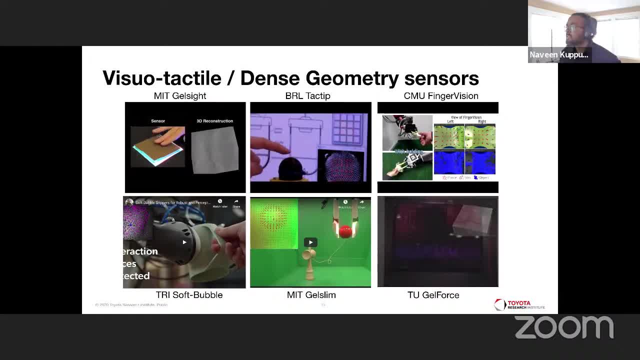 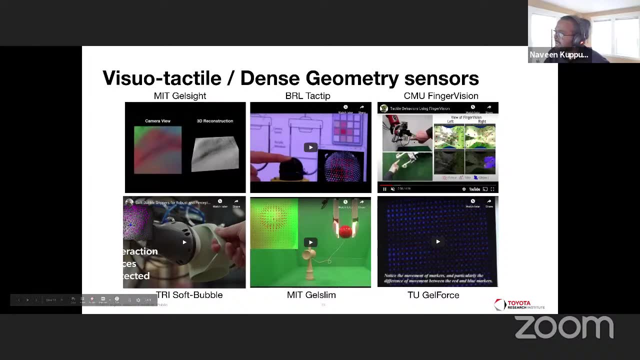 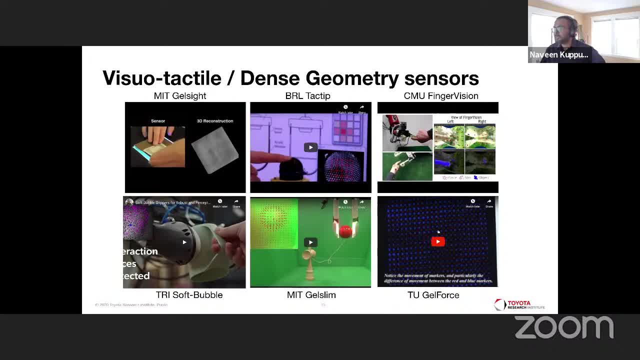 of these markers which are then captured, And then you can see the motion of these markers which are then captured. And then you can see the motion of these markers which are then captured, captured with some kind of vision-based techniques to process. 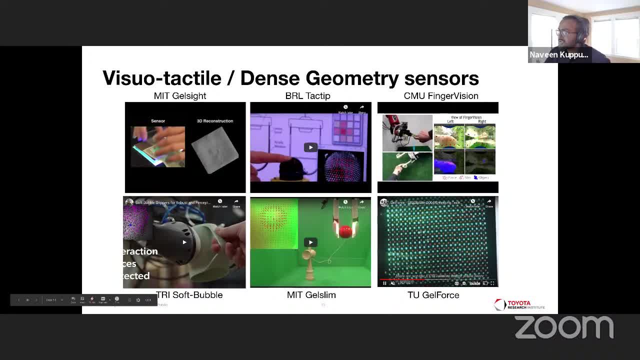 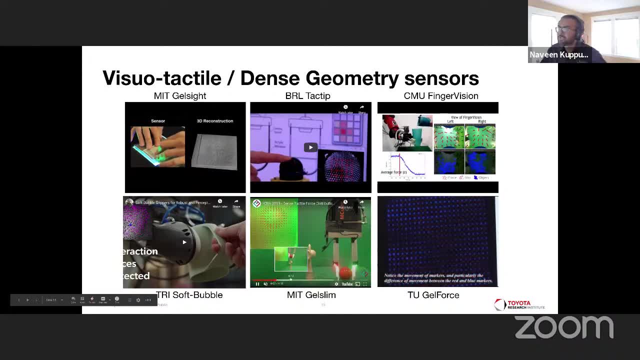 A couple of other examples: the Tokyo University GelForce is one of them. The MIT GelSlim, which is a closely related cousin to the GelSight and which also uses similar methods to understand both the depth as well as how external forces 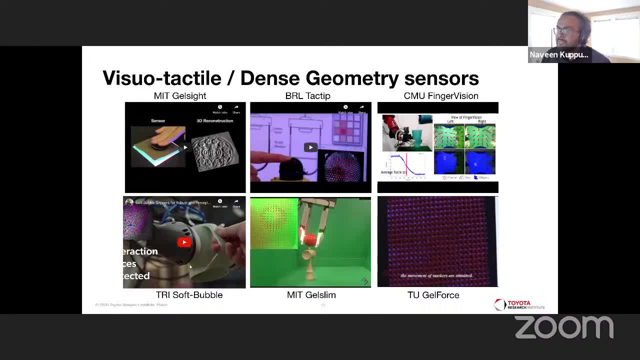 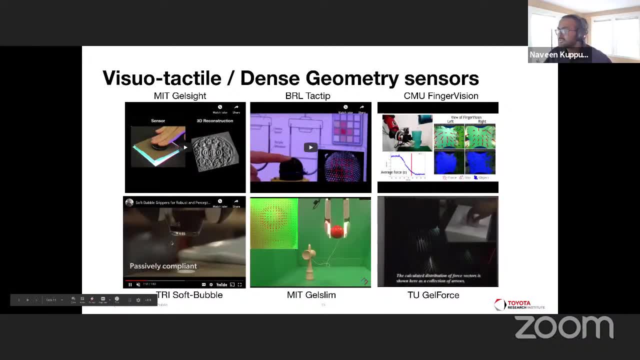 are influencing the tactile impressions And, of course, lastly, the TRI's soft bubble sensor, which I will talk a bit about towards the end of this talk. So if you had ended this talk by asking me what is your favorite sensor? 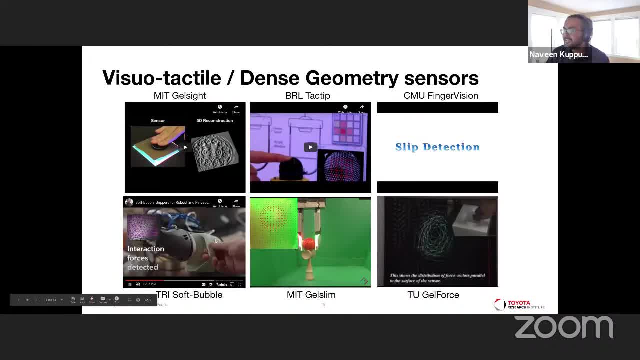 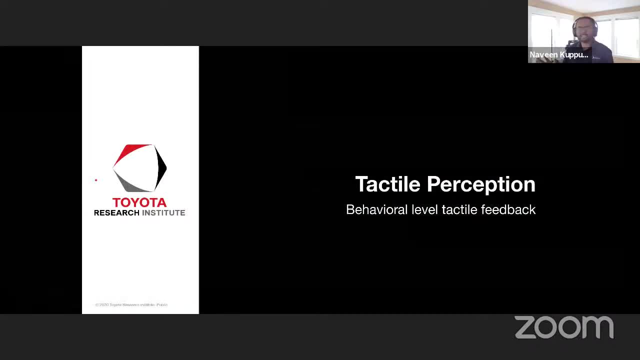 It's one of these. So there you go. That's my naked bias on display. So now, moving on, let's talk a bit about tactile perception. But actually I would like to quickly ask: are there any questions at this point? 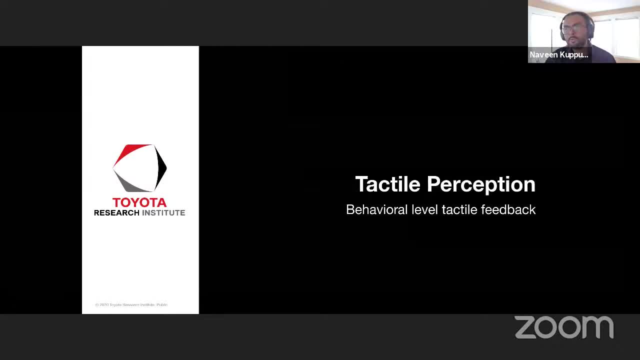 No, I'm only seeing four faces because I still haven't mastered zoom. Oh there, I see more faces. All right, All right, I am assuming I'm seeing a lot of understanding and comprehension in your faces, So I'm going to proceed at this point. 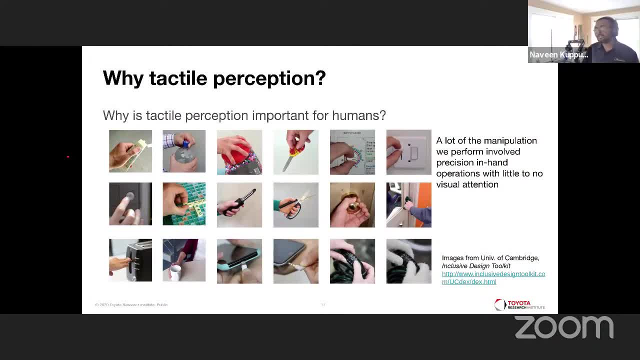 So why is tactile perception important? And I'm drawing the slight difference between perception and just tactile feedback control for a specific reason. So a lot of manipulation we perform involves precision in hand operations or with little to no visual attention. And take a number of these objects and a number of these tasks which you're used to. 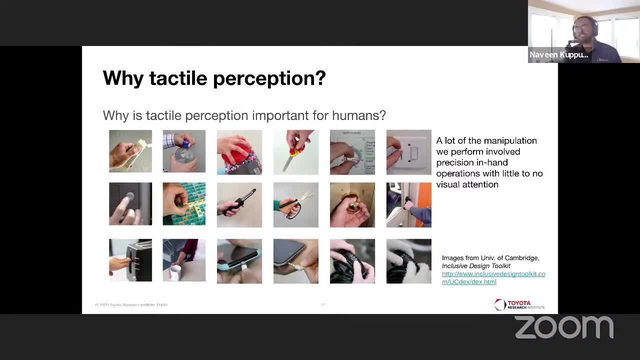 performing all the time and perhaps recall how much of these tasks involve you actually looking at your hands and trying to see what exactly you're doing. And it turns out a lot of these tasks beyond the most basic visual cues. you're capable quite well of performing them with just a sense of touch alone. 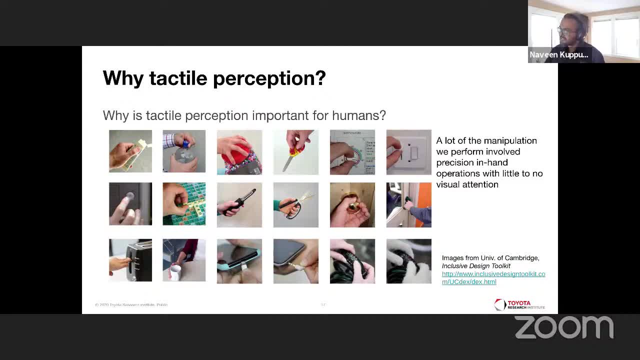 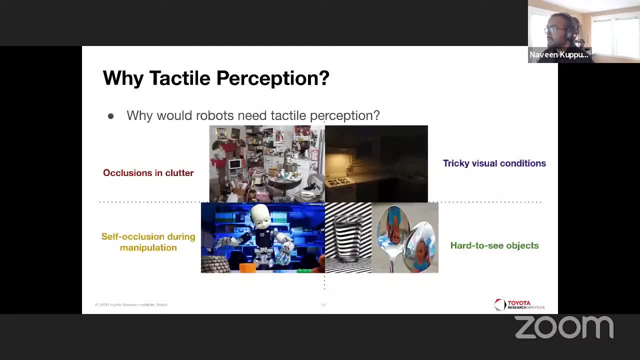 So not paying attention is also fine, because your tactile system is paying all the attention required to perform a lot of these tasks. Now let's go back to the robot case, And this ties in very closely to the image I showed before. There are four problems I'm throwing out right here which specifically call to attention why we need tactile perception above and beyond just camera-based perception. 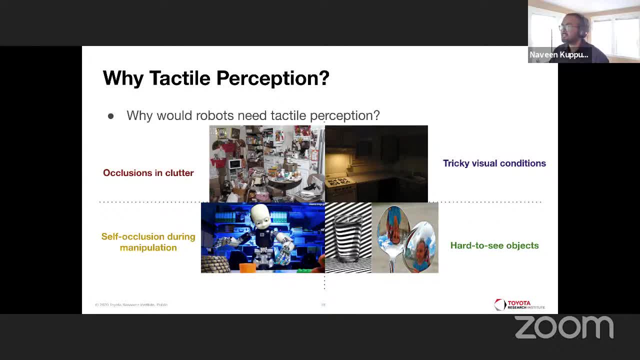 So occlusions. take that lovely home right there, And after a few months of COVID I'm not sure how many of our homes look like that, but I have a strong suspicion it's quite a few. Then you have tricky visual conditions. 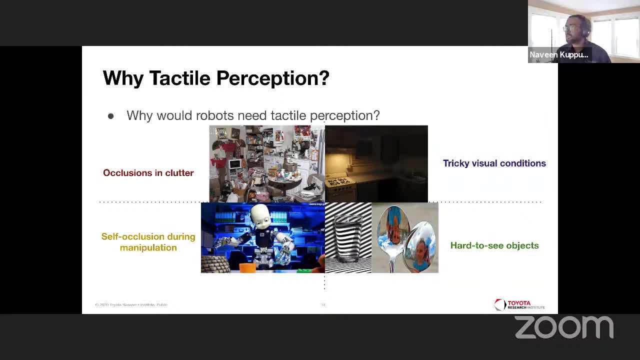 Of course you cannot guarantee perfect. I mean, we have lighting sources in our homes and quite often you're asked to manipulate without having sufficient lights to see what's going on. On the bottom right you have this very interesting category: hard to see objects. 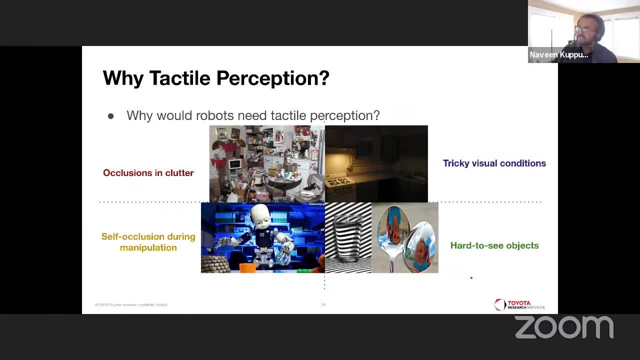 You can throw in a lot of processing to understand these objects, for instance with these specular reflections or with which are transparent. But a lot of times perhaps you don't need to pay that much visual attention because you all know your eyes can lie. 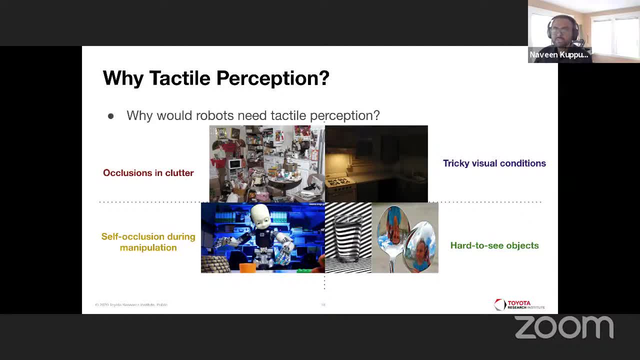 On the other hand, you can just go touch the thing And perhaps Understand what you're sensing right there. And lastly, any robot is susceptible to self occlusion, because once you actually go reach out and make contact with this object, you're starting to instantly block external perception from even getting a clear view of this object. 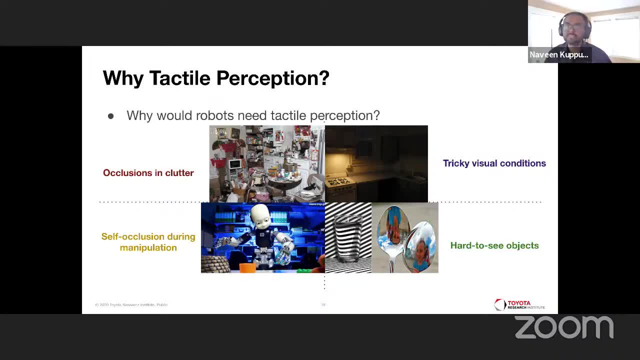 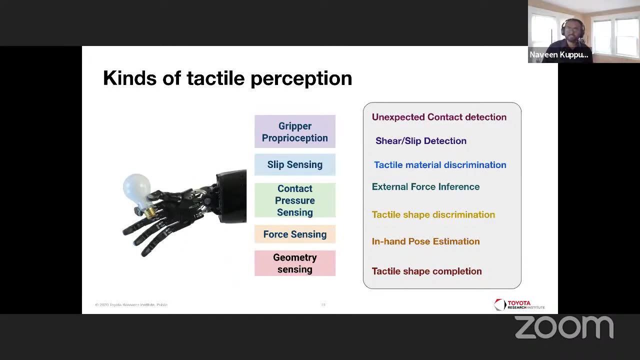 So, especially in the case of these dexterous grippers, with these multi-doff fingers, you quite often tend to occlude yourself. Now, moving on, I threw out a set of tactile perception problems and I would like to just kind of walk through some of these different problems. 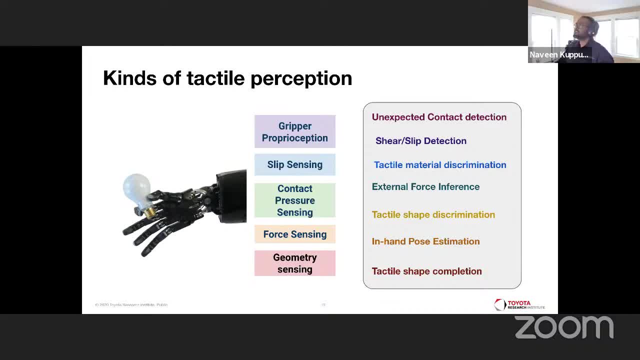 And this set here you can think of as your set of skills which you can embed in your own robots if you had the right form of tactile sensation. So let's walk through this list. So let's start with unexpected contact detection. This ties in exactly with the DRC example which I presented earlier. 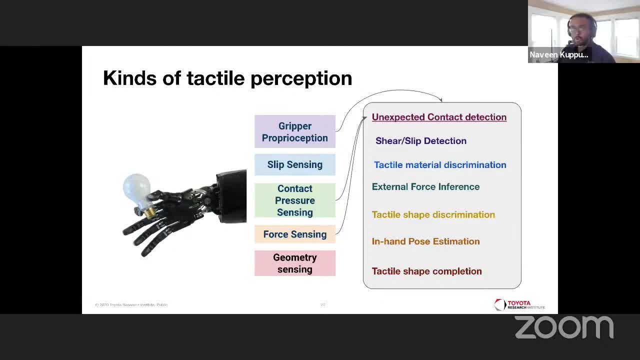 There is a sudden contact, which you didn't expect, either on your robot or on the object which you're trying to manipulate, And you would like to detect that something happened and therefore perform some fast activity to respond. Just a moment here. There we go. 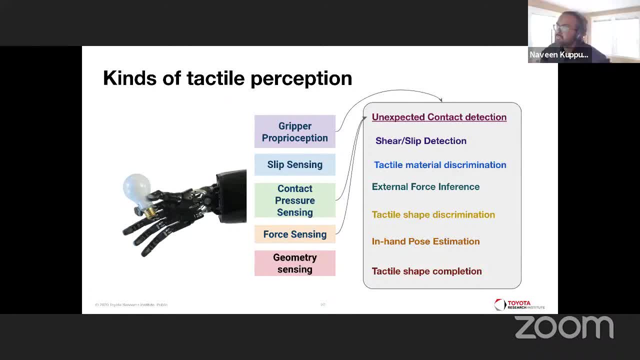 So And The The three ways which, in general, you can try and compute this is to directly sense forces, to sense contact pressures, and the gripper proprioception is, of course, trying to understand where your finger is in space or where the fingers are relative to the gripper itself. and all these kinds of information combined 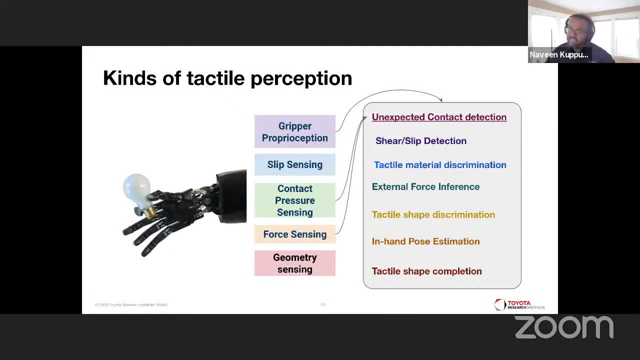 Now why I pick out these are because a lot of times these kinds of sensory perception tend to be really fast and when you want to detect an unexpected contact, you want to react really quickly, And this is when i think it would be particularly helpful to have the finger in space, or the fingers are more likely to be a bit faster if you try to do this. 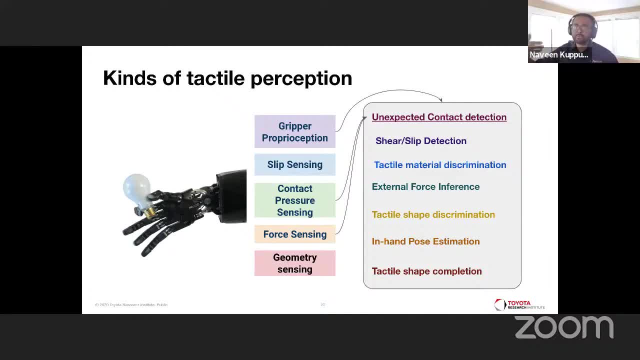 So you'd like some form of sensory processing where you are able to very quickly glean what has happened to your robot because of external contact, and you perhaps don't really want to sit and number crunch your way towards understanding that contact happen or not. you want to instantly know that contact happened to my robot. 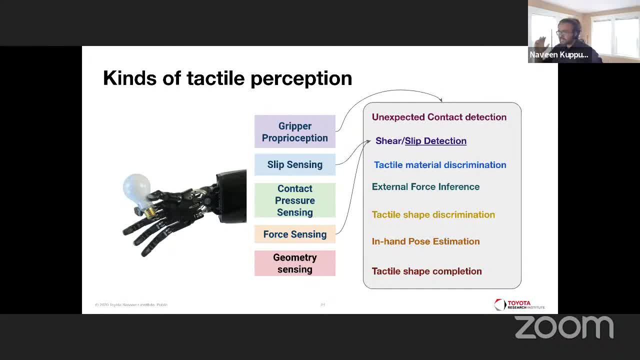 The next question here is to detect slip or shear. Specifically, you would like to understand if the object is slipping from your hands or if you're having your hand mounted on a surface. The surface itself is slipping away, and that is a more permisory distance metric than you might expect. 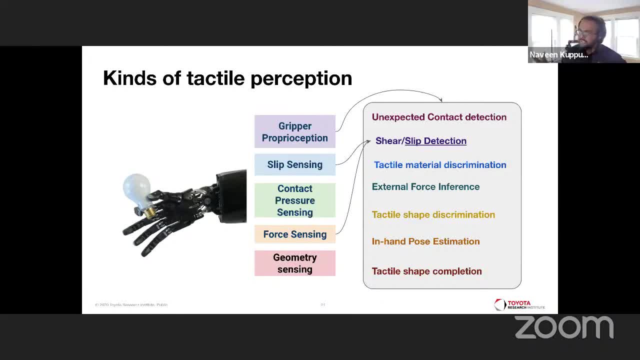 itself is slipping away due to whatever reason, And shear is a phenomenon which happens on your way to a slip, where the object itself is subjected to these tangential forces And you would often use some kind of force sensing. You may have dedicated hardwares. 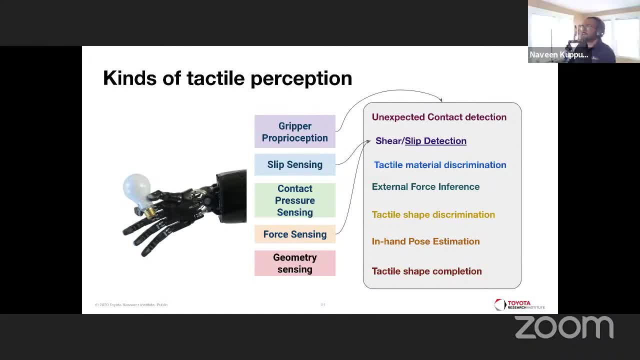 Can you hear me? Sorry, It was all good. Yeah, And you may need dedicated hardware to perform this kind of slip sensing in order to understand this. The next problem: this goes back pretty much exactly to something Meng mentioned, which is performing some kind of tactile material. 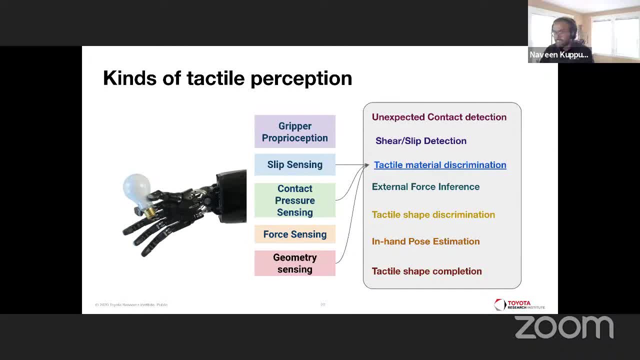 discrimination. Now, this could be useful for a number of high level skills, Like I put my hand into a bag and I'd like to know: am I touching a piece of plastic, Am I touching a piece of wood Or I'm touching an unknown surface? 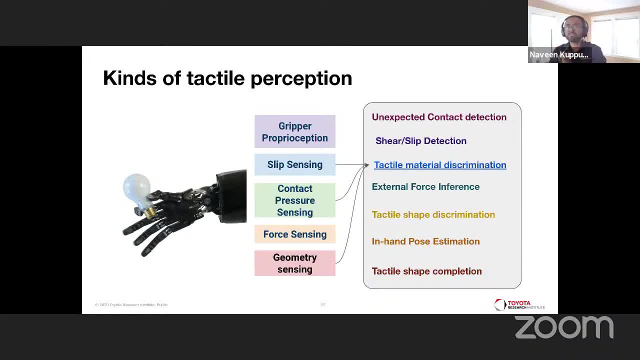 as my robot is regressing. Perhaps knowing what kind of surface it is will quickly help me decide how much weight I can put on my hands. So often this kind of material discrimination can be dealt with classical classification techniques, as we know, in perception. 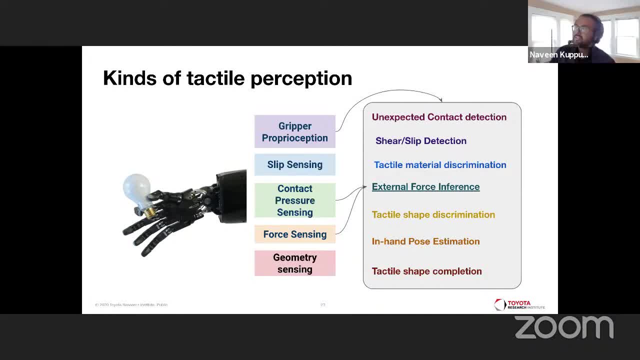 External force inference is a more expanded version of unexpected contact detection. Perhaps you want to not just say that there's an external force. Perhaps you want to actually look at what is the direction of this external force and try to cope with that direction change. 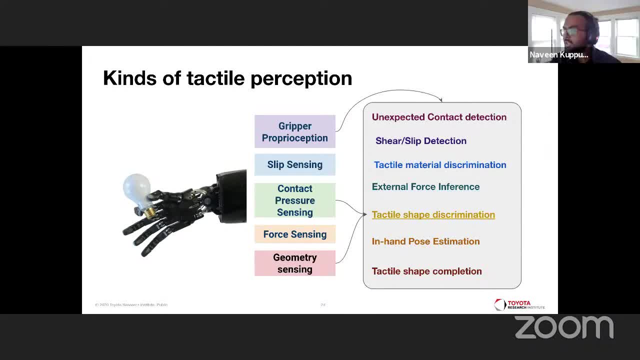 Next comes the next problem. OK, So I'm going to talk a little bit more about this problem. So I'm going to talk a little bit more about this problem: shape discrimination and the problem which I'm going to heavily focus on for the next phase of this class. 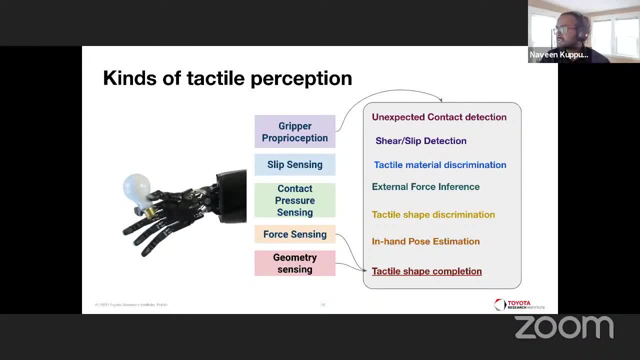 which is in-hand, pose estimation And, lastly, you can even perhaps touch an object and infer a lot more about the shape of this object through this tactile shape completion, style problems. So, for today's focus, these are the different problems which we will talk about. 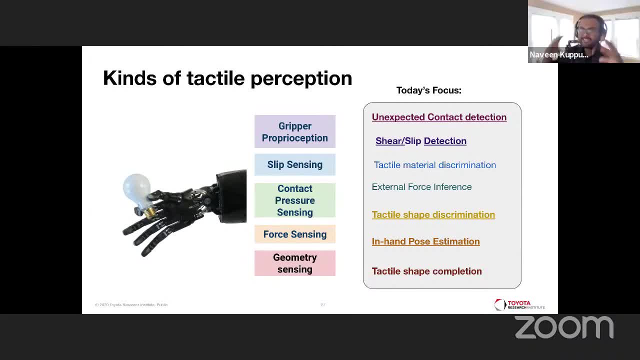 For me always it means number crunching to understand something about the state of the robot and the world, And some of these I'll talk in terms of perhaps performing some direct feedback and helping you cope with something unexpected when it happens to your robot. 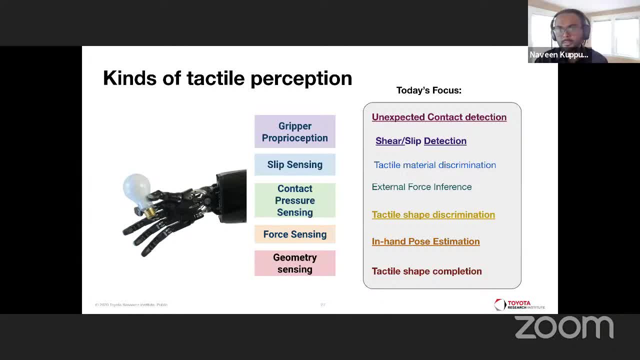 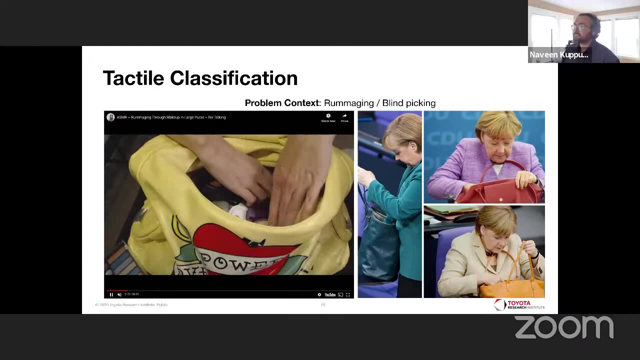 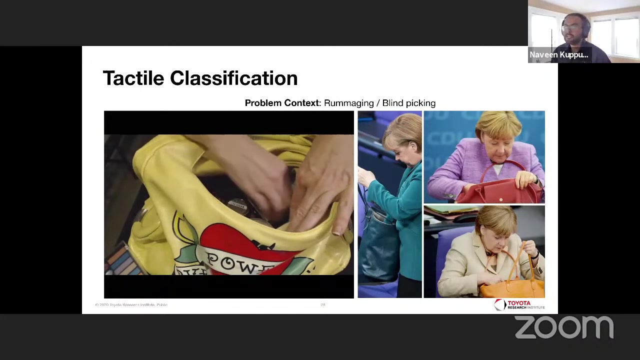 Any question at this point, As I am flipping through your faces, I do see plenty of comprehension. I hope So. I will. I will proceed. So let's take the tactile classification problem. So a number of you understand this context. We have our favorite chancellor rummaging through her handbag. 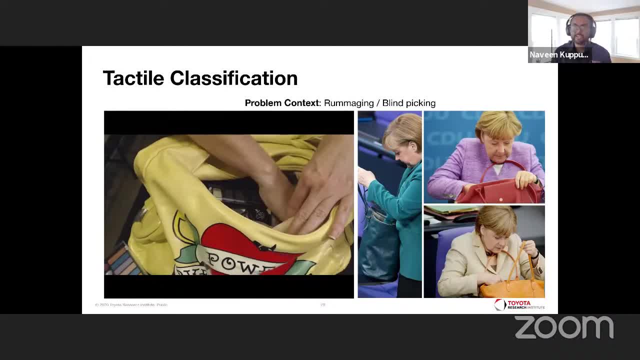 What if we want to perform something like blind picking? You want to stick your hand into an enclosed surface, pick out a single object. Now, you don't necessarily need to know what that shape of this object is, but perhaps you just want to know. 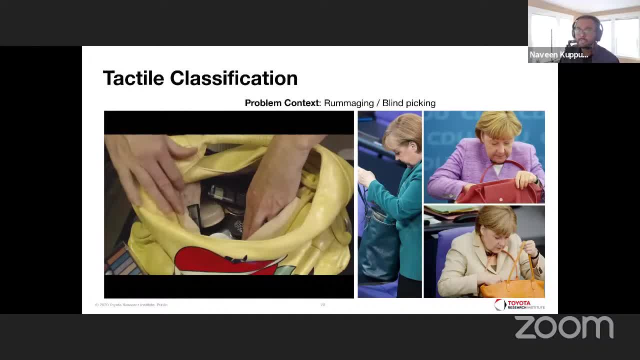 there are different classes of objects, And I want to- just, I want to just stick my hand in and pull it out. Now, why can't you do this as an image-based or a vision-based classification problem? This is an enclosed surface. 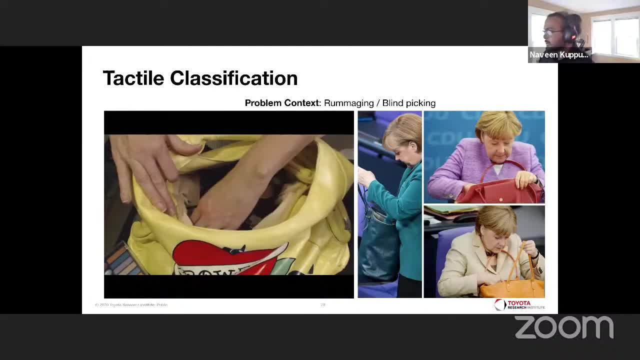 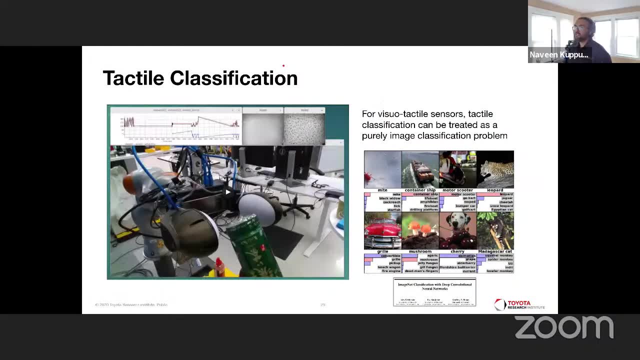 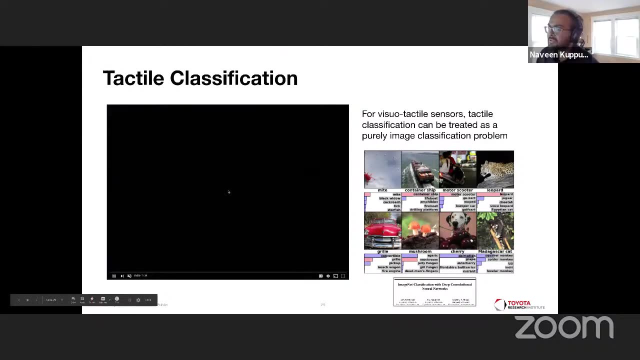 It's kind of hard to actually pick out what is it that you're dealing with. So in this problem perhaps comes a really important aspect for a vision-based tactile sensor, If you want to understand what it looks like to actually make contact with this object. 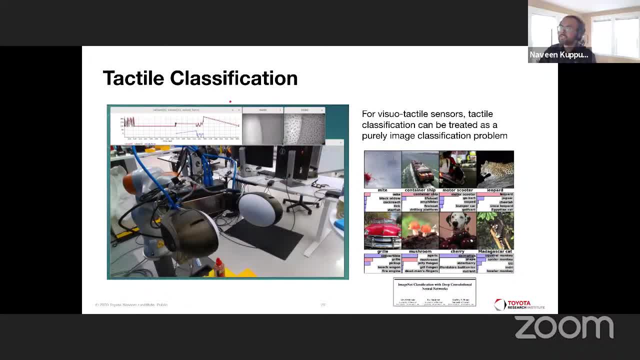 So take, for instance, the TRI soft bubble gripper. here I'm introducing a number of objects And you see on the top right there the tactile impression created by these objects. So this is the view from the cameras embedded in these kind of tactile sensors. 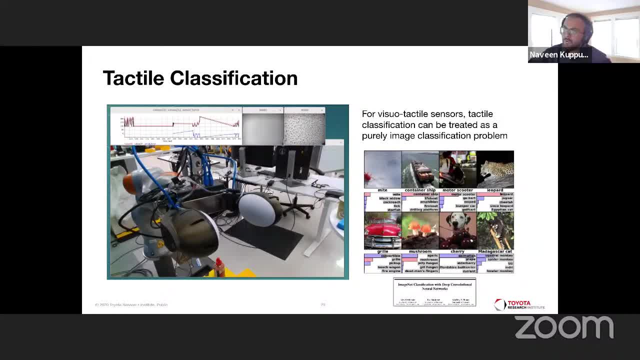 And the instant I am telling you that, this is a view from the cameras of making contact with these objects and these object categories are known. perhaps we can treat it purely as an image classification problem, And that is a problem which we understand pretty well in the world of VR. 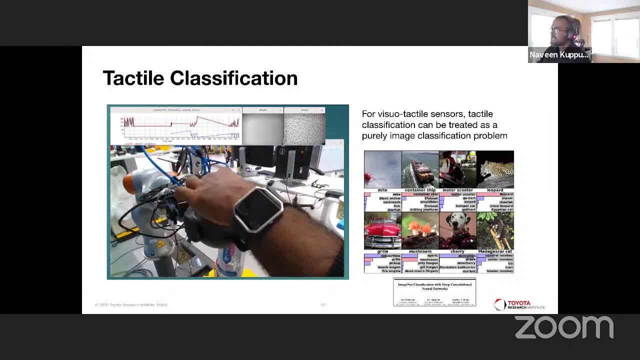 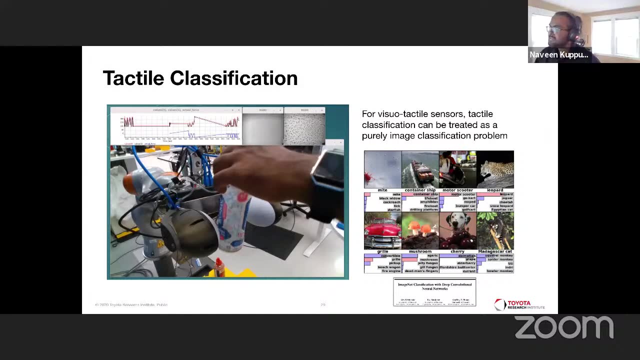 It's a problem of camera-based perception. So these images, of course, are from a well-known image classification work which is known as the AlexNet, And we have these different classes of images And from the pixel information. we would like to know what is the class of this object. 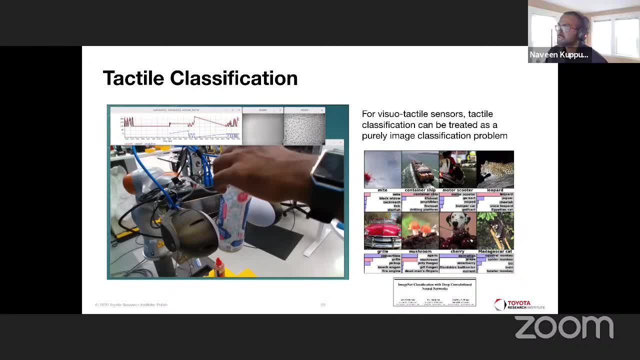 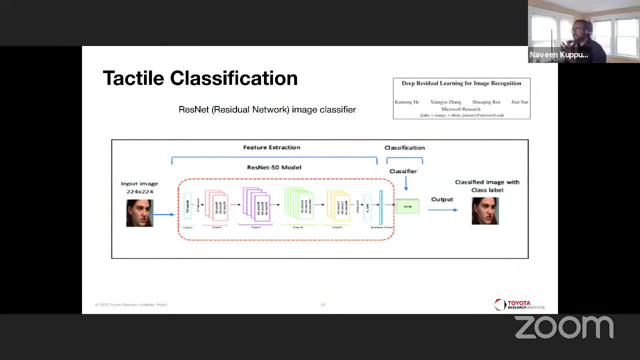 either as a probability or you just want to say this is the class that I directly infer just from the pixel information. So let's take one. Let's take one of these networks which is pretty well known for how well it has performed on some benchmark data sets. 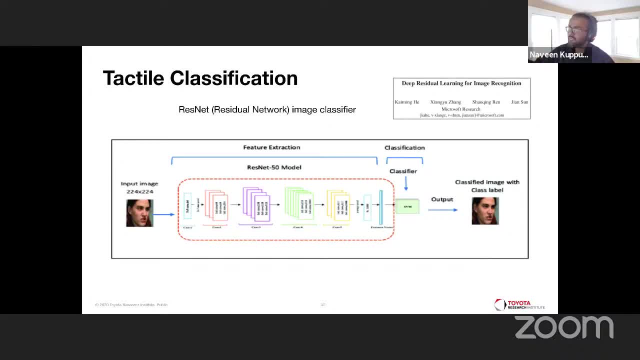 It's known as the ResNet or the Residual Network Image Classifier. For more information, I recommend you dig into the actual source paper. But suffice to say we are using a convolutional neural network And in this particular instance, what I'm illustrating 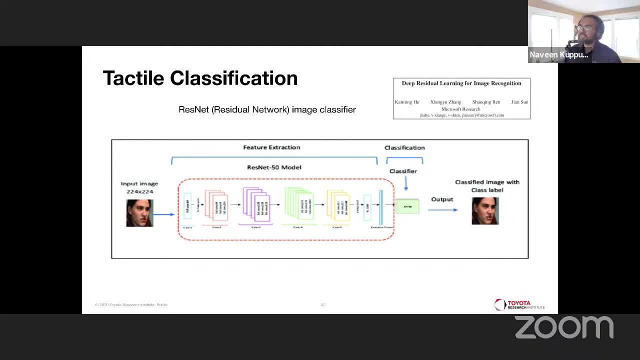 is the so-called ResNet-50 model, So with the 50. refers to the number of hidden layers that are present in the image. the number of hidden layers that are present in the image and the number of hidden layers that are present in the image, we can. 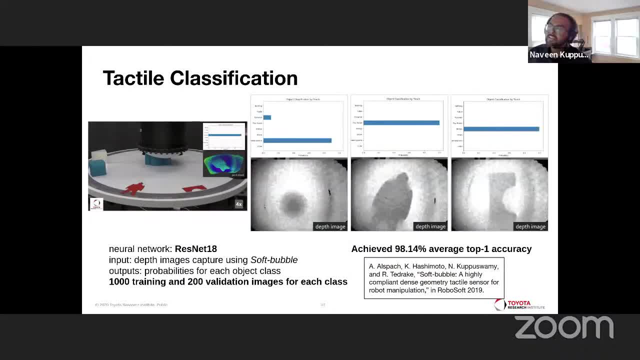 use the ResNet problem and the actual classification part really comes out with a class probability and a label for the class. So in the case of tactile images, if you had classes and if you had images, sufficient amount of training information, you can treat it exactly as a ResNet problem. 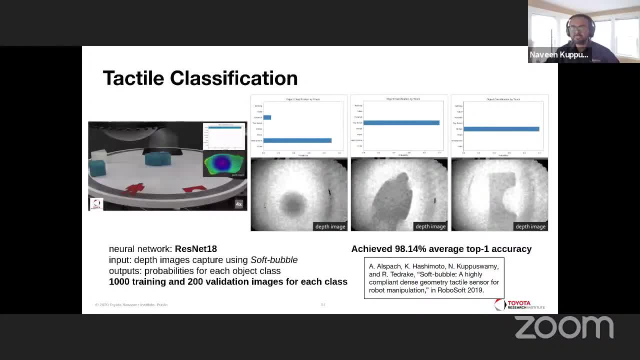 So this is the kind of classification I just picked our work simply because I have nice gifs to show you what's going on. Now, the key interesting aspect which you have to keep in mind is: why is it hard to perform tactile classification as opposed to camera-based classification? 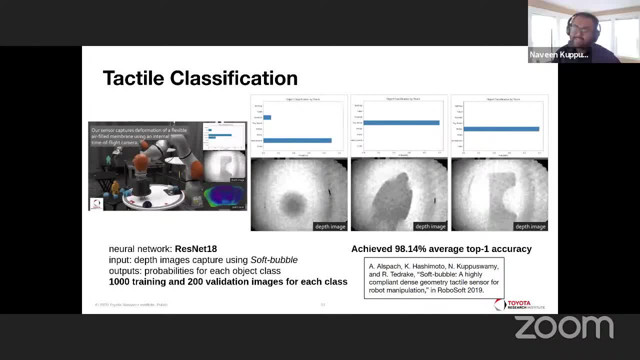 And the answer is quite simple. In a camera-based world, it isn't quite as expensive to obtain labeled images. You can stick a camera on a scene, You can move around with your camera, You can sit there annotating these images or farm it out to the cloud or get an outsource. 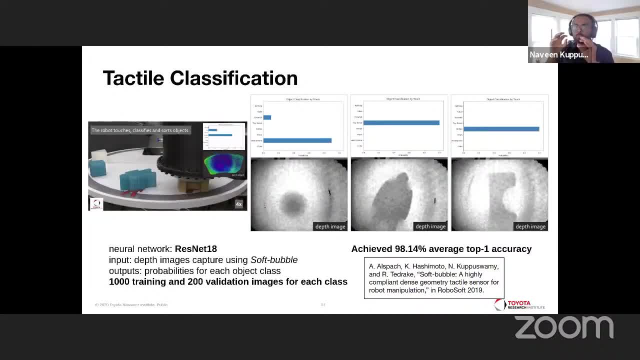 that information to a company to sit and draw or mark out what are the objects you see in a scene, Whereas in a tactile case you actually have to go reach out and touch the object, and repeatedly touch the object to get a sense of what all are the possible ways in which this object can. 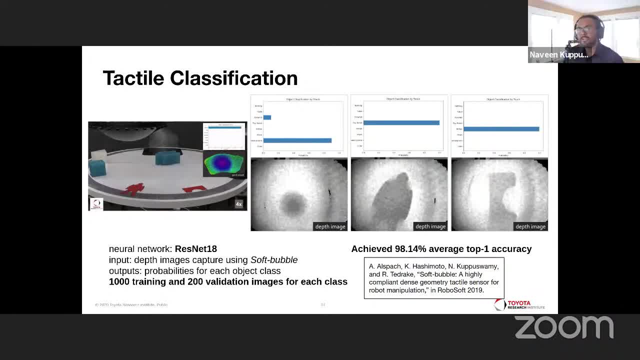 be touched, to obtain your corpus of images, to train your network. Now, what does this entail? Anything which is making contact is slowly degrading or abrading. You're literally reducing the lifetime of your sensor with every single contact you make. So, in other words, tactile classification. 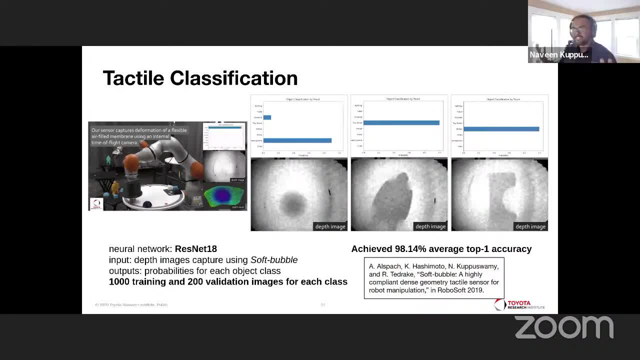 starts becoming challenging from the perspective of. it's not that easy to suddenly obtain a corpus of tens of thousands of images, because for each of those tens of thousands of images you should have made tens of thousands of contacts. So this is quite the same as saying a robot should. 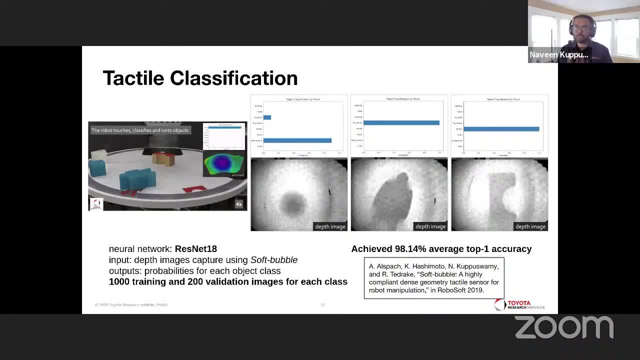 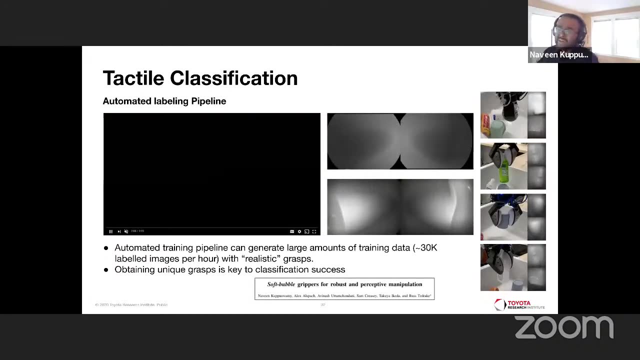 sit there playing with objects repeatedly in order to get a sense of what all one single object means. So this is usually the tricky nature of performing some kind of tactile classification, which is how do you give it enough training information in an effective way? Now, one part of this problem we tackled at TRI. 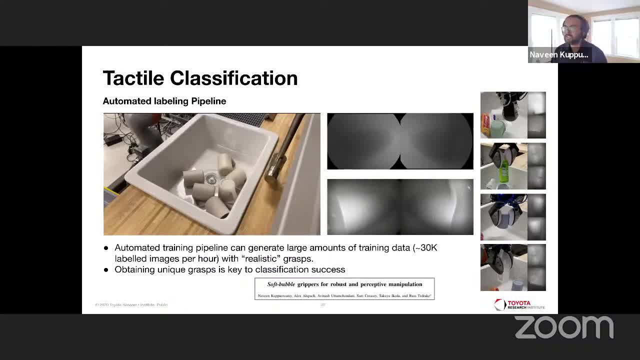 was to simply perform some kind of automated labeling. In this particular instance, what you're seeing is the scene in front of the robot filled with a single class. In this particular instance, the class is called Mug. Now, I mentioned two factors. 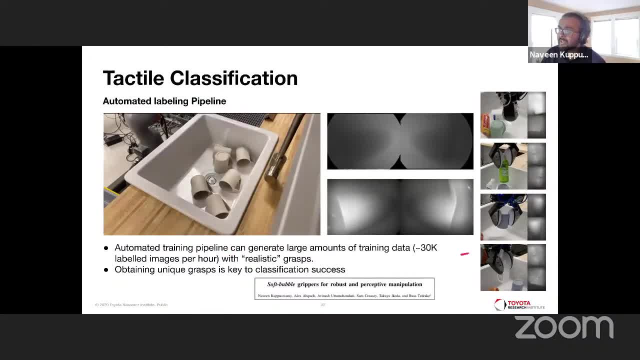 Here. one is the amount of training data you can create inside an hour, which is usually a determinant of how well a classifier works. And the second aspect here is also a key aspect to think about when it comes to making tactile contact. The uniqueness of a grasp is key to classification success. 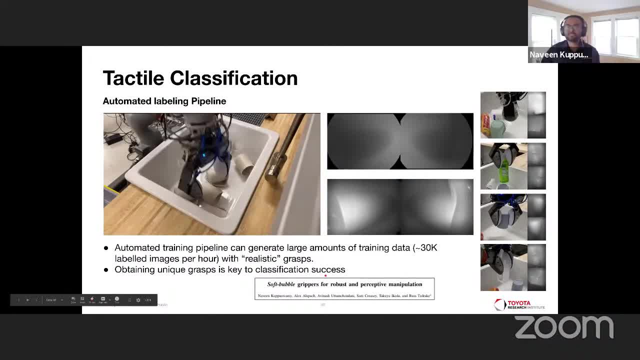 So it's not the number of training images per se. You could have tens of thousands of images of dogs in a scene and train a network to classify if an image contains a dog, But in the case of what is a mug, you perhaps need to capture every possible instance. 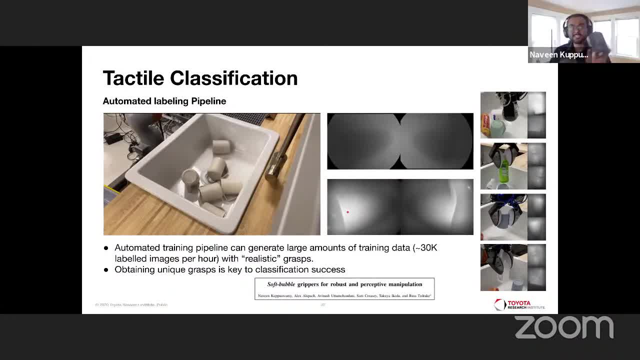 of a mug being held in your hand. Now I have a coffee mug in my hand. There's a lot of possible ways in which you can grasp this possible mug, So quite often this also tends to be a determinant of your success when 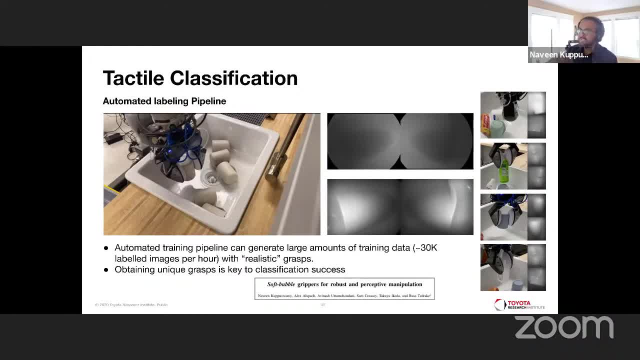 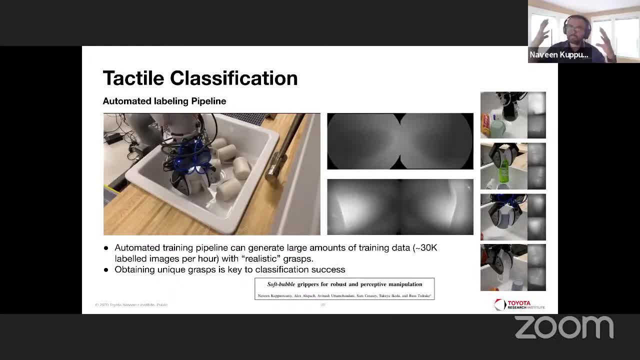 There's a lot of data. There's no one short answer. The answer is perhaps something in between: Find a more data efficient way to perform your machine learning. Perhaps you need to find a more efficient way in which you can make contact And, of course, make your sensor itself way more robust. 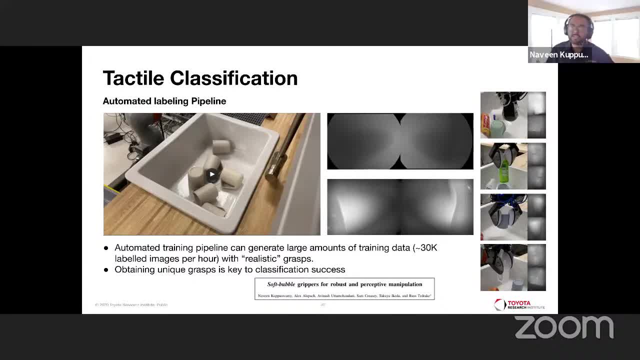 that it doesn't even matter if I were to make tens of thousands of hours of contact And perhaps that sensor is sitting out in your lab sitting and sensing And you can transfer that learning to another tactile sensor which is deployed in the field. 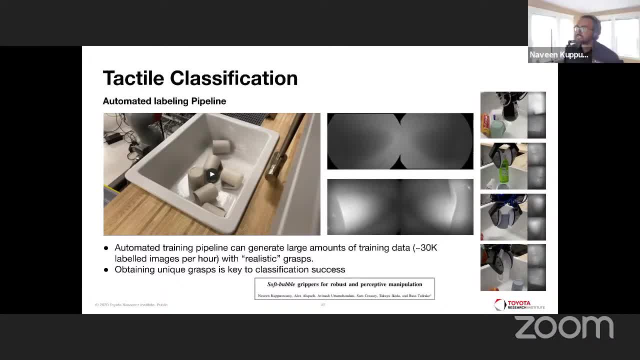 And this transfer learning aspect is also a challenging question when it comes to tactile sensors, Because it's not always the same for two different sensors to sense the same phenomenon and give you the exact same outputs. There may be minor differences between each sensor due to the nature of the contacts. 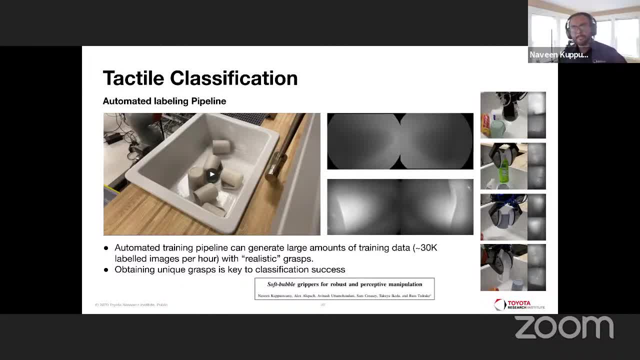 Yeah, I've got a question about that exactly. Go ahead. So any two cameras have different distortion models And that doesn't seem to have impaired the ability to see And that doesn't seem to have the capability of image classification tasks from being able to do what they need to do. 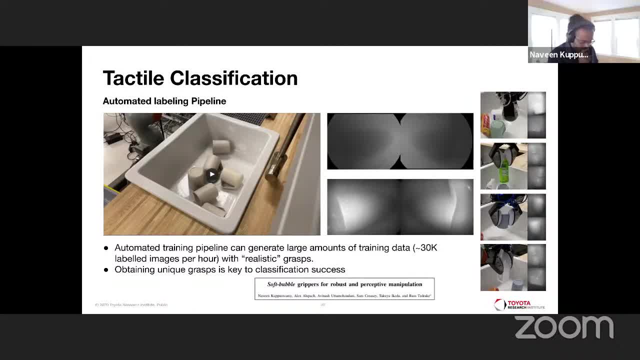 How much does it really matter that your sensor is degrading or changing over time as you do these tests? Isn't that like? I guess? what I'm leading to is: is it sufficient for one research lab to generate a corpus that another research lab can then? 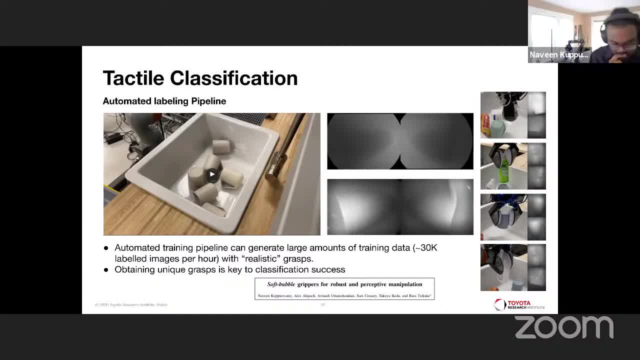 use on their sensor? Is there enough, You know, at least within the same class of sensors, gel sites or something like that along those lines, to be able to deal with the fact that, yes, while we've only, you know, the image net that you then 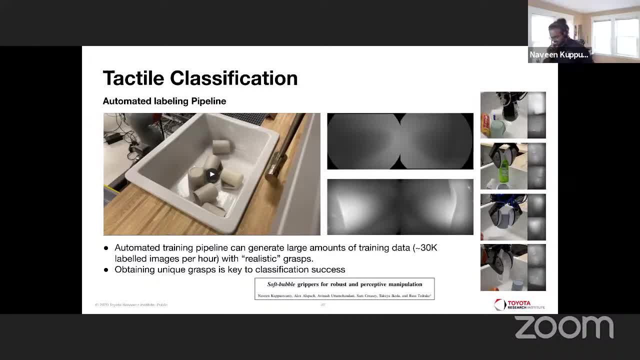 fine tune on your specific sensor or something? is that in the realm of practicality? So there's an excellent question And I'd like to unpack it in two possible ways. So you hit the nail on one hand, You hit the nail on two hands. 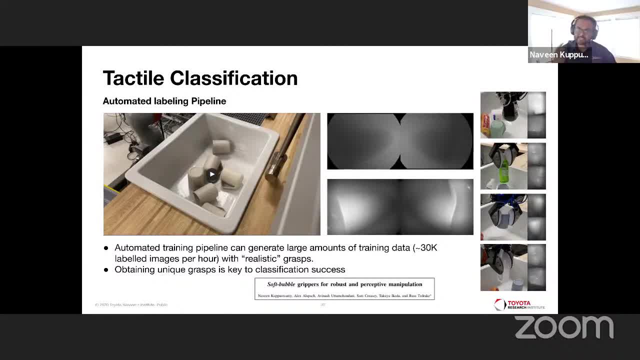 You hit the nail on the other hand. You hit the nail on the other hand, And it depends on the object that you're getting. But you can also have an example of what can be done where, where you can go, and then you can actually start working out. 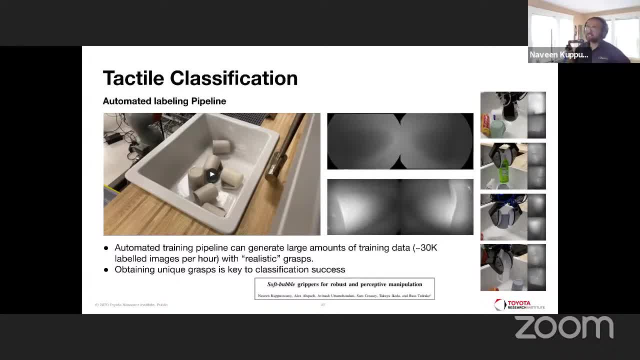 what you're trying to do with your sensor, and then you can think about how to deal with the worst object that you're thinking about. And so one way that we can仰- And I'm going to leave it a few minutes here, because I do want to take it a little deeper- 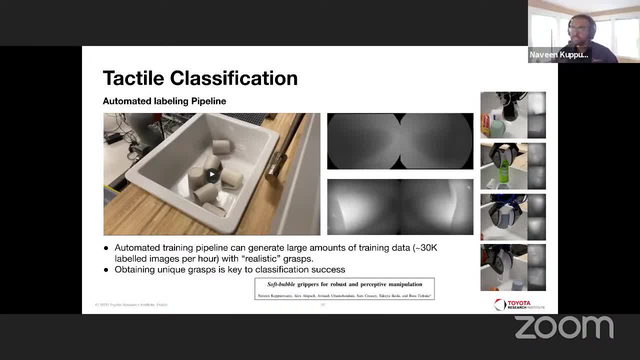 And I want to start with what's going on with the sensor, A couple of things that we think about. So we've got this. this is an example of it. This is something that I have done: how your sensor is making contact with this particular object. now, when it comes to generalizing, 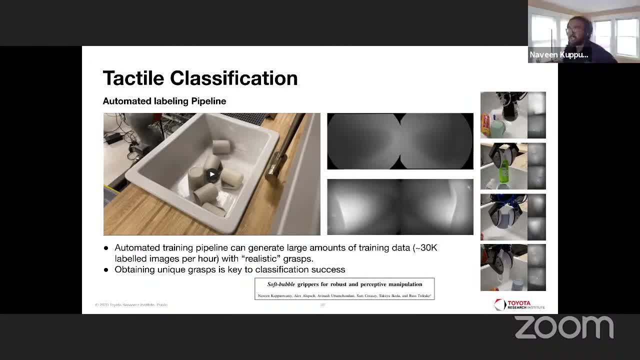 across sensors. that's a way harder question, simply because what each sensor senses is so unique to the physics of how the sensor itself has been built. and i'm specifically talking about how, how compliant the sensor is, how much of the surface the sensor is measuring. what is the 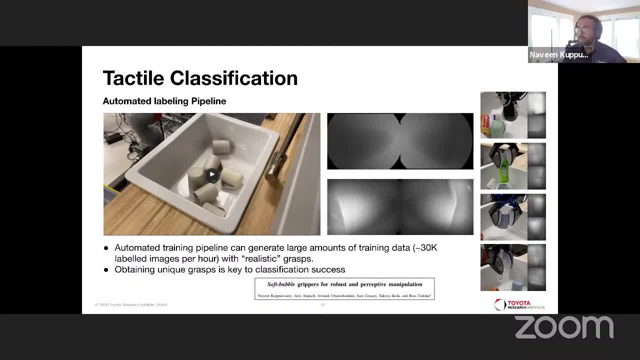 resolution of the surface geometry that you're sampling. all it comes down to really saying is: can there be some way of understanding that a grasp at this point of the mug is almost the same as a grasp at this point of the mug in terms of telling that it's a mug? now you know for a fact. 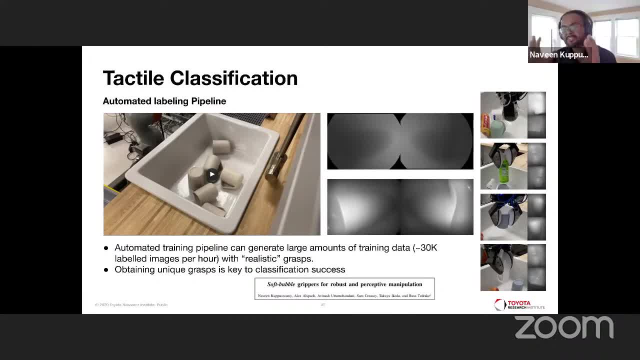 that from your own sensation. if i were to give you something vaguely cylindrical, something made of ceramic, you'd probably just guess it's a mug, until i gave you extra information to tell you that it's a mug, and all of us have fumbled around in the dark to know that we can confound ourselves. 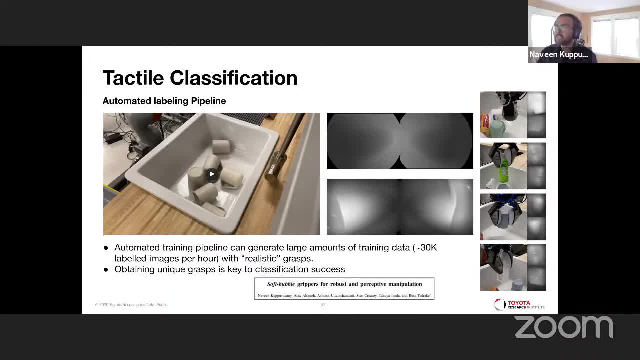 sometimes with tactics sensation, so you do need a huge corpus. so the unfortunate answer for your question is: there's no straightforward way and indeed it's an open research topic. and how do we find a data efficient way to train on these kind of tactile sensors? does it answer your question but does not answer. 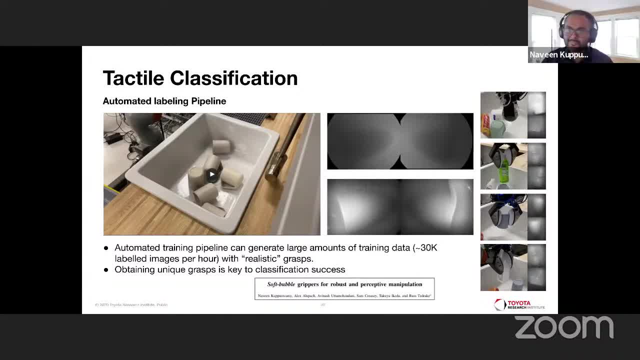 kind of um it's, it's more. you know, in some senses, image net broke up wide open, people doing tons of things, and with, with, and, and. it is that all it would take is take, you know, all the different types of sensors out there. you know, have have had 10 different research labs. each of them generate a hundred thousand images. 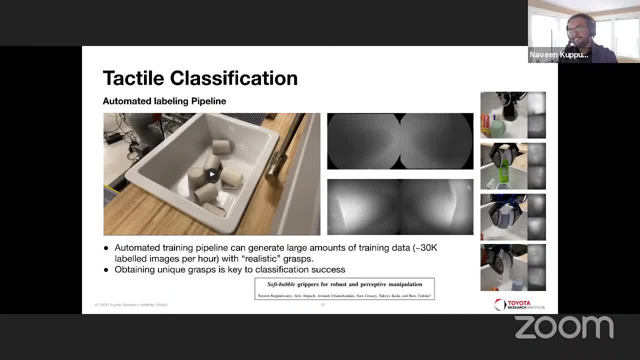 with their and and put it all into one data set and turn the deep learning crank is, is, is that? is that in the realm of practicality, not nothing is a practical? i do think that is in the realm of practicality. um, i mean, the same example could also be turned around and saying: a single robot as it keeps performing tasks. 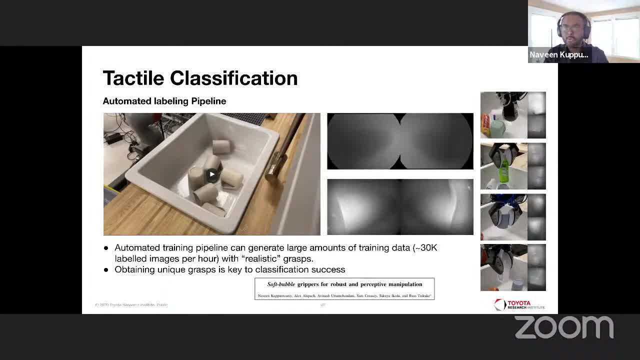 encountering new objects, can it add it to its corpus of known objects? so perform some kind of lifelong learning. so either learn from other agents or learn from your own experience and grow your corpus. now the second aspect is literally, uh, something we tackle, so i don't see why not the 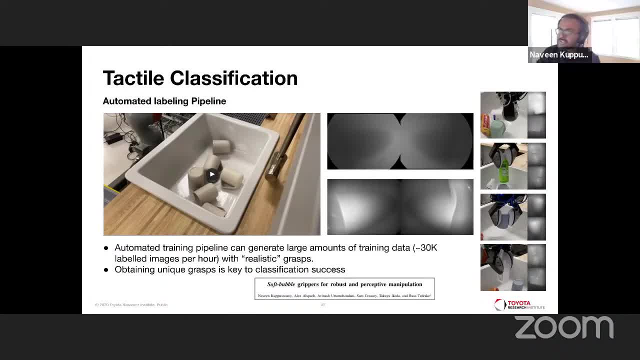 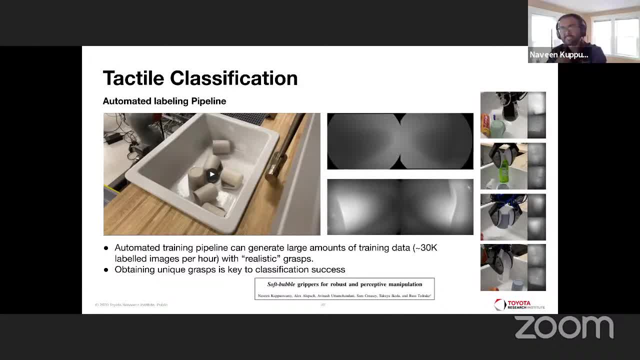 find the minimal number of parameters which define the way one sensor behaves, uh, and figure out why each tactile sensor of a same instance is slightly different. but i do agree what you said is totally within the realm of possibility, uh, but the more we investigate a data efficient learning strategy, 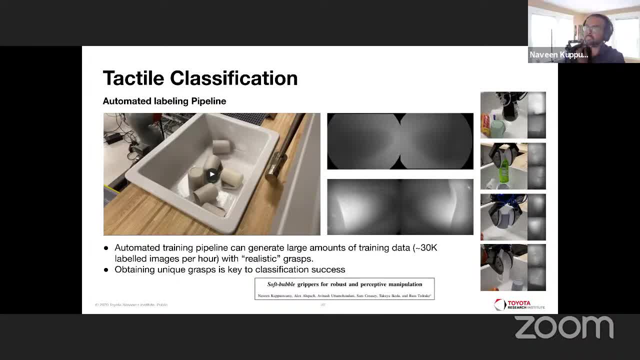 the better off we are because, at the end of the day, every sensor which makes contact abrades degrades, and that is something which a camera-based uh uh thinking does not really entail, you don't? you don't lose off lifetime of your camera every time you turn it on, in quite the same way as a. 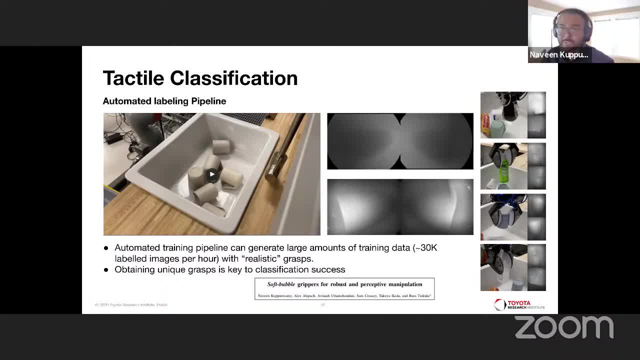 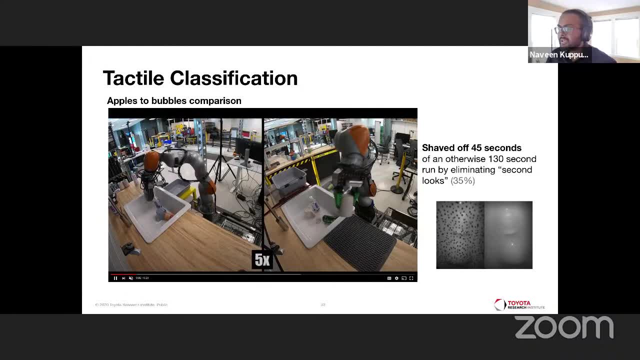 tactile sensor. so that's really my point, but good question anyway. so yeah, there's somebody else. perhaps just some loud muting. so this is uh, incidentally, the result of performing that kind of uh training by letting our robot self-explore and learn objects. uh, we would joke and call this the apples to bubbles. 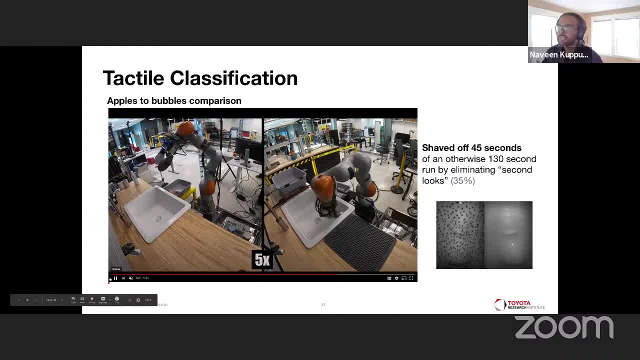 comparison because, uh, you have this scene which, uh- let's restart the video as i talk, you had the scene which, uh comprised of objects which need to end up in the dishwasher, such as mugs, and objects which need to be thrown away, such as trash in the form of these pet bottles, and so on, and really, 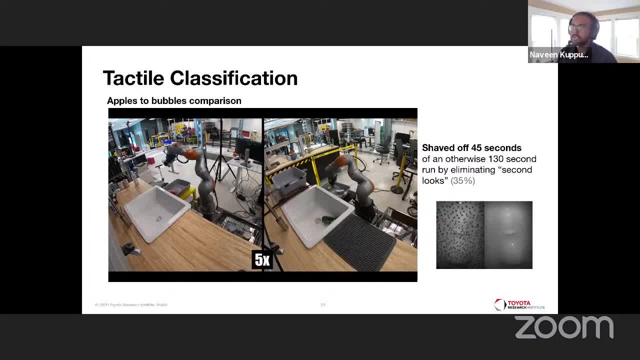 could we train the robot to simply from a single touch, or learn to understand what the robot is doing? what is it that is being touched now? uh, in this particular instance, i don't want to say this is true for all time- if you were to use tactile sensation and perform this classification, uh, end. 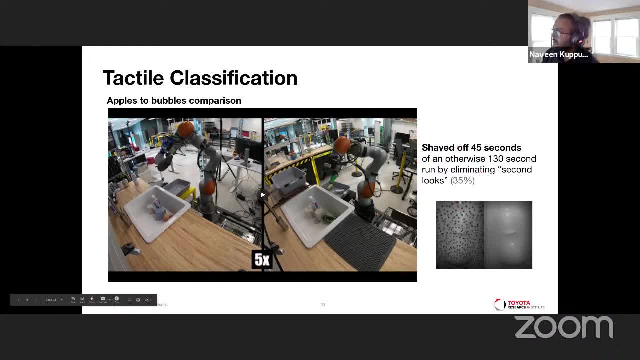 to end, we do achieve some uh gains. in this case, uh, a 45 second shaving off the total time. now what that means? in the view on the right, you had the robot. pick out an object and if it is sure what it is, from camera-based techniques, go deposit it in the dishwasher. now keep watching the. 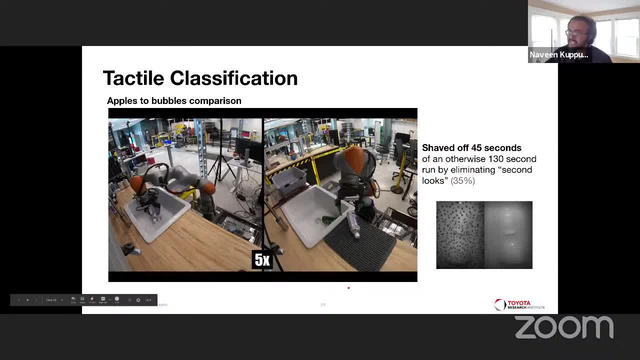 scene. on the right you see the object robot pick out an object and singulate it to let camera-based techniques tell better if it's trash or not. and part of that is because when you're going in grabbing an object you tend to occlude the scene and telling what's in a scene when you're partially 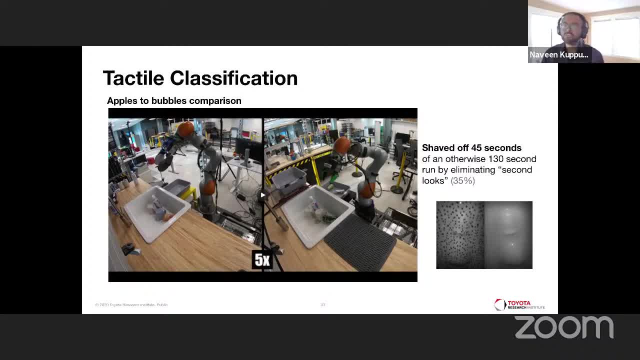 occluding is a lot harder, whereas with the tactile sensor you're not really going to occlude your own tactile sensor. that's, in a way, the beauty of tactile sensation, which is, if you're occluding, you're touching something else, and if you want to tell what you're touching, you're literally touching. 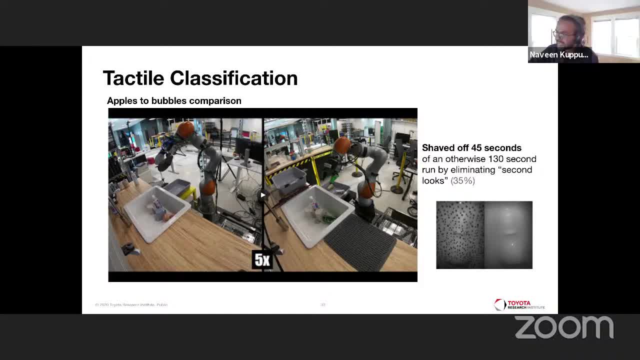 the thing you're touching and if you want to tell what you're touching, you're literally touching the thing, so you don't have the question of occluding your tactile images. uh, really, and that leads to some speed up. are we clear on classification before i move on? i think you made a super good. 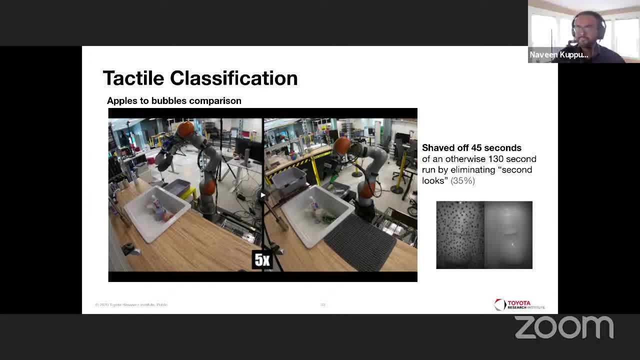 point in in the middle- there i want to make sure it lands- which is that you're getting a very different view of an object when you're touching. it's a much more local view right than uh, than the more global view that you'd get from a camera looking at it from away. so, like your example with 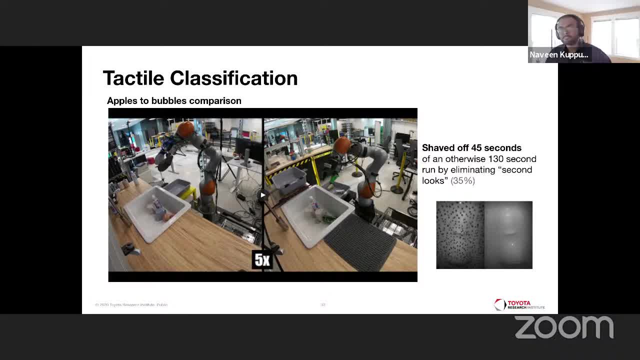 the whole mug. i think was perfect, right. so the fact that you're just seeing the curvature and you're asking yourself: can you identify the whole mug, it seems like a very different problem than seeing it from a distance and getting a more global perspective. so you like end up having to. 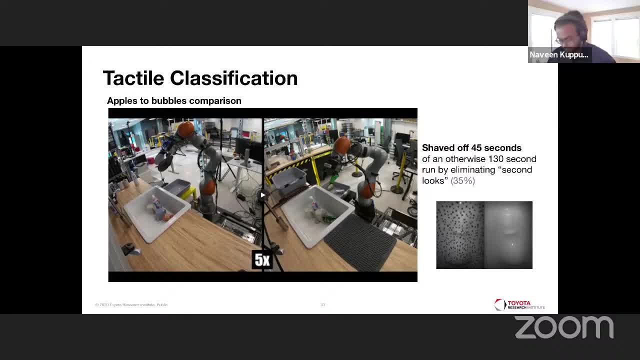 think about texture of the mugs and are being the important cues instead of, like you know, it's got a handle right, so it's super interesting to think about. there's also a question from and it's. it's a great point and, yeah, go ahead, terry. 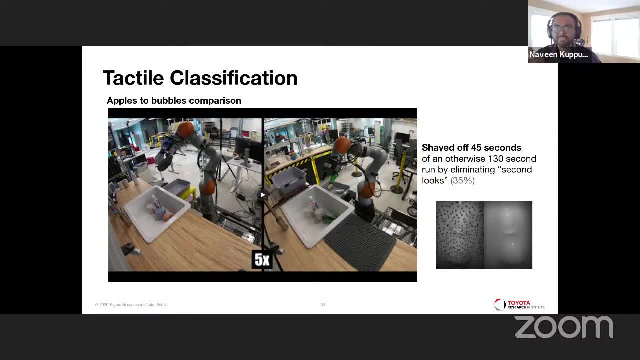 oh, i was just going to say sorry, somebody spoke. does the model work with tactile sensor images? that's? that's a great point and we'll briefly talk about it towards the the last part of this talk. can you have a known model for what a tactile sensor can? 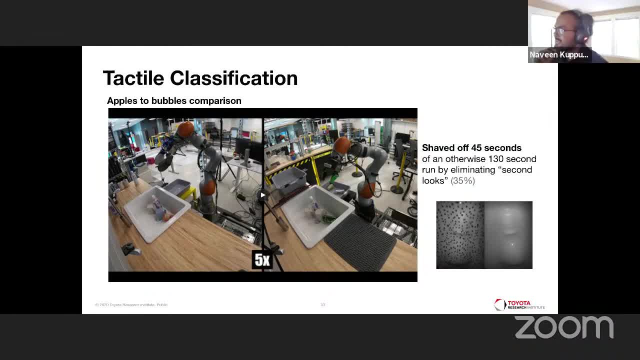 actually perceive. so is there a, is there a sensor independent way of saying what is a tactile sensation you expect from this particular object, or even a tactile sensation you expect from a sensor dependent way? and that expectation is a hard problem until you fully understand the physics of the tactile sensation itself. now i also want to emphasize, in this particular mug example. 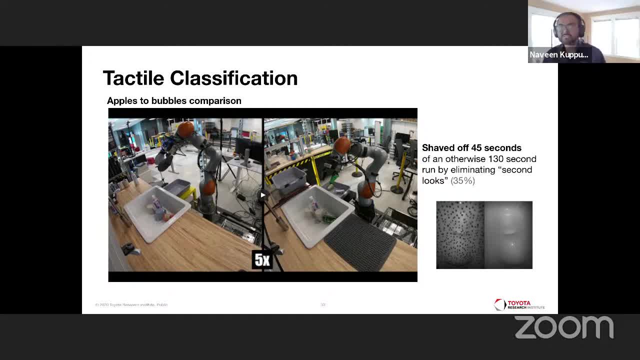 what we tend to think of as visual features in a camera based world are quite different from what are interesting features in a tactile world. so, uh, something which is uh, which has confounded us in camera based perception, is this perfectly blank, featureless surface like a big 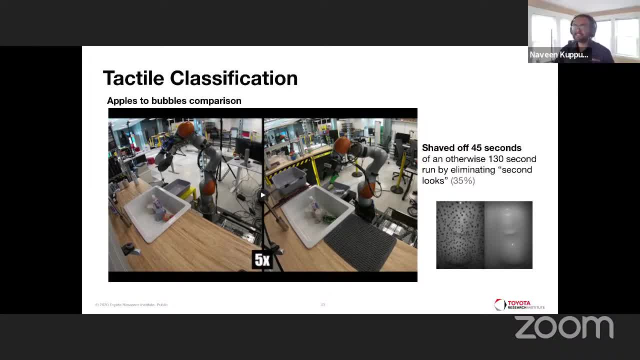 white wall, now an equivalent in the world of tactile, is a perfectly uniform material. it doesn't even matter what shape it is, if it has no features, as long as it's uniform and it's curvature, exactly like the surface of this mug. so for a tactile sensor, this mug surface is highly 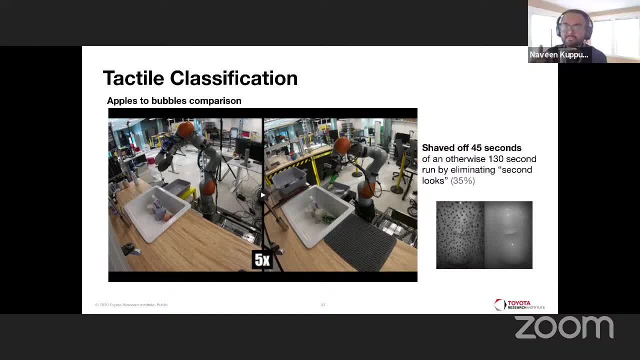 confounding. it's not easy to understand. how is this surface different from this surface? different from this surface? there may be microscopic differences, but do we really want to process information at that level of spatial scale? these are challenging questions when it comes to classification and a lot of these questions also. 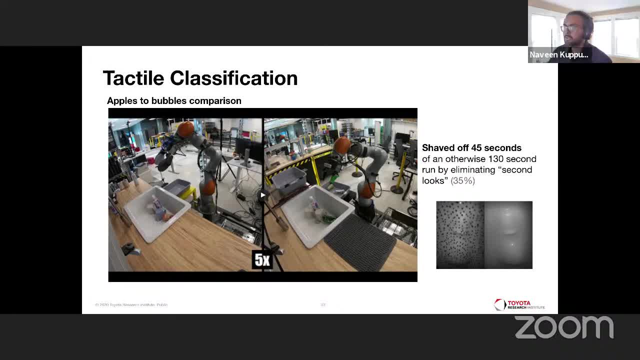 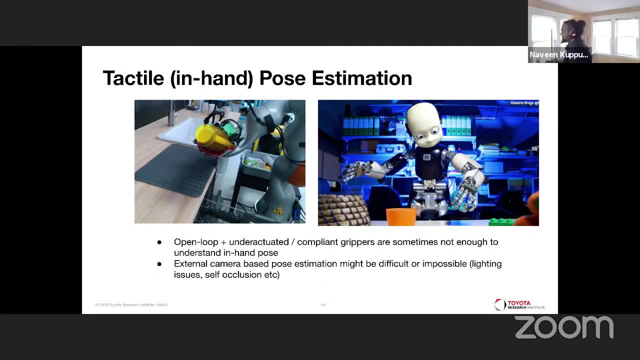 quite nicely tie into our next problem, which i'm going to talk about now, which is in-hand post estimation. so why do we need to perform tactile post estimation now? you had, i think, two lectures on the topic of post estimation using camera based techniques, specifically using uh. 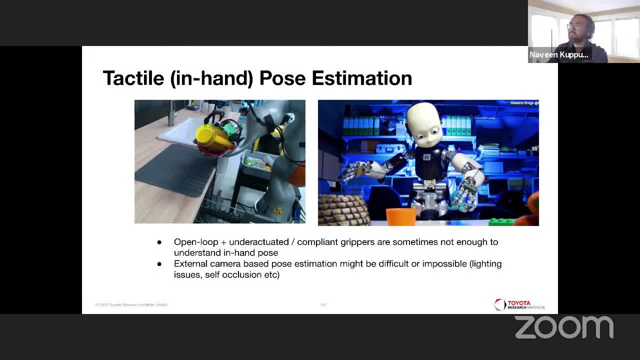 these depth sensors or of different formats. so you know that camera based perception can work or may have issues in working under some specific considerations, but why do you even want to think about this in-hand post estimation problem? and that's what i want to talk about. so the first: 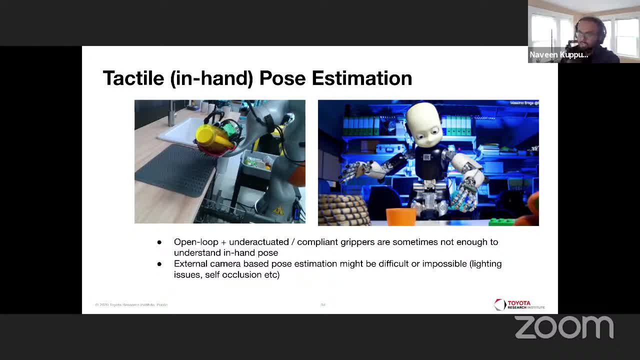 thing is, uh, right at the beginning, as i mentioned before again, uh, we know that we can be kind of open loopy with a sufficiently compliant gripper. we have all seen these beautiful videos of robots rummaging through piles of stuff and picking a thing and placing it elsewhere without really 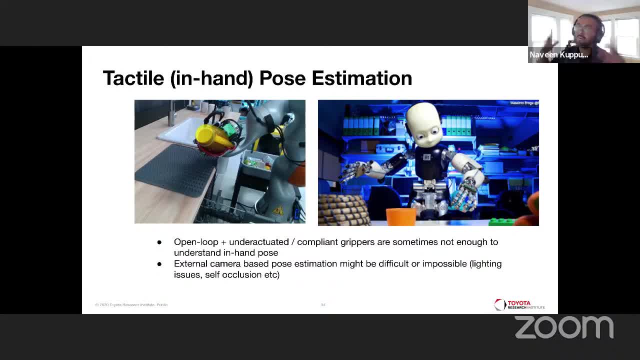 reasoning about what they touch as long as they know that they are holding something in a loose sense. so sometimes that is not enough to tell you how you're holding an object. on the image on the left you have an interesting comparison. so what you had was the robot reaching in into the clutter. this is the 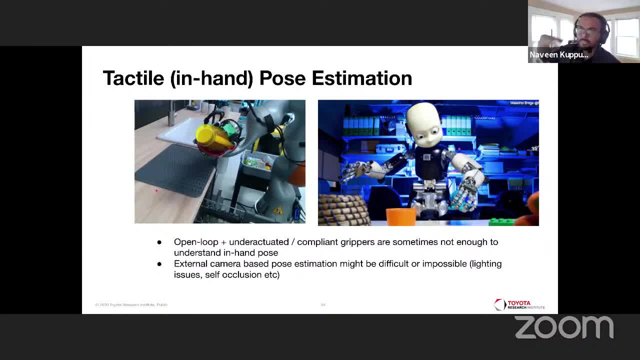 robot at tri, for instance, grabbing a mug with some hypothesis about what was the pose of the mug coming in from the cameras and the robot then picks up this mug and on the camera frame we are now trying to compare the difference between the expected mug pose, which is in the translucent, shaded color. 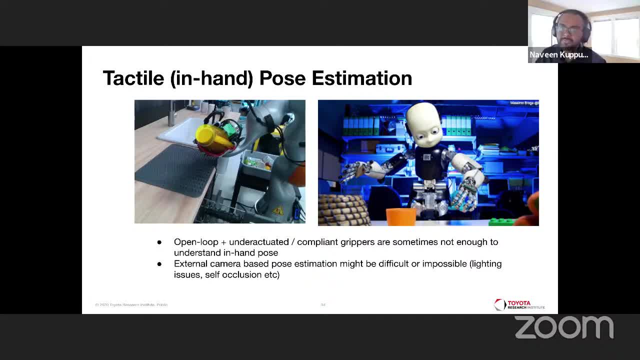 and the actual mug pose, which is in the colored image in the form of red. now it looks subtle, but that's a pretty important distinction for an object such as a ceramic mug. why is that the case? so, first and foremost, why did this difference even happen? now, the difference happens, obviously. 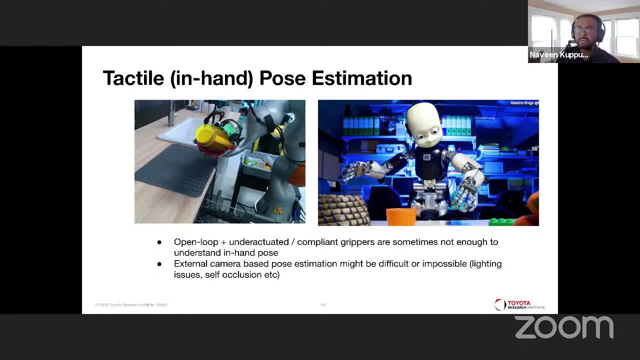 because contact is a complicated phenomenon, especially when you're contacting with two surfaces, such as a gripper. a lot of things happen in the small few milliseconds as you're starting to make contact, which push an object away from where you expect it to be and it ends up at some other location. 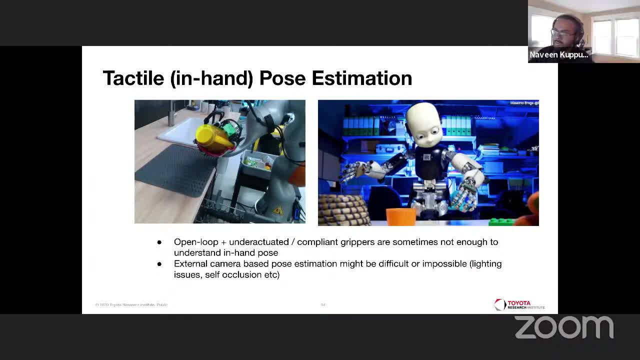 in space, which is really where this problem comes from. but second, this small distinction really starts affecting us if you want to perform some precision action after you grasp an object- and that's an important point- if you were to simply pick an object and place it, you perhaps 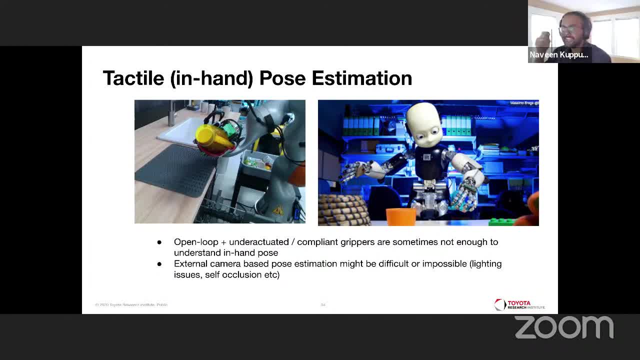 don't need enhanced pose estimation, only if you really need to understand how you want to place it. perhaps the object is fragile, like a mug. it needs to be placed in a specific way. it cannot just be dropped. perhaps the object has very specific requirements based on what it's containing. for instance, maybe it's a coffee filled. 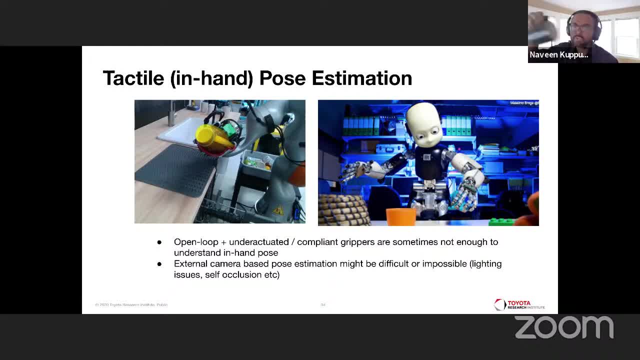 mug. i want to hold it always with the top upright. i don't want to just let or move it all the way around when i'm grabbing it, so i want to keep a track of is it pointed upright. so these are all tricky questions and, of course, not to mention our favorite example. 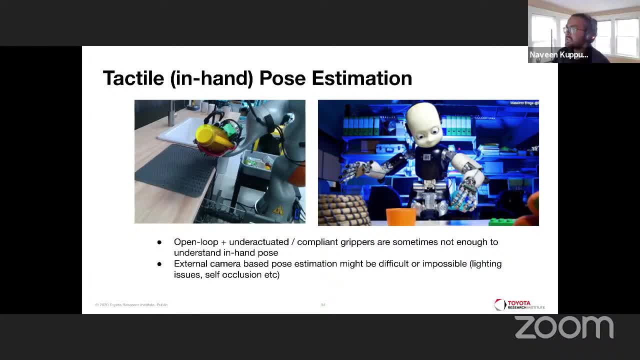 as i listed before, self occlusion and camera based problems may also fall into this realm. you can keep looking at your hands with your eyesight, but quite often your hands would cover your eyesight, making it an extra hard post estimation problem, as you might know from your. 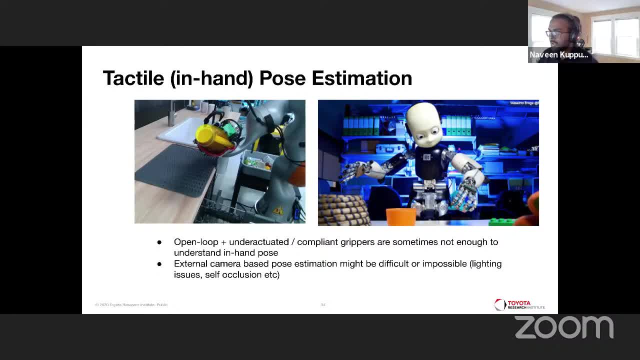 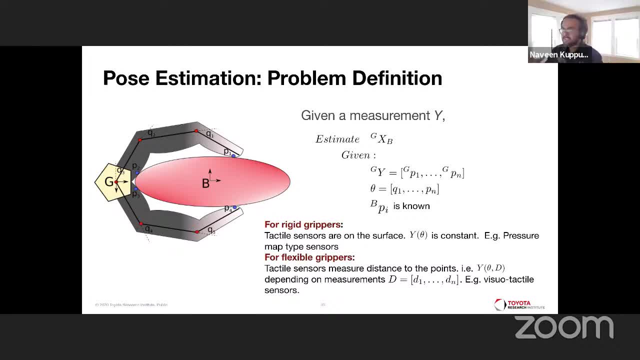 work and post estimation earlier in this lecture. so let's study this problem definition. we have this gripper. i just drew this fictitious gripper holding this object b. the gripper has an associated reference frame g and we have this measurement set y. now what this? 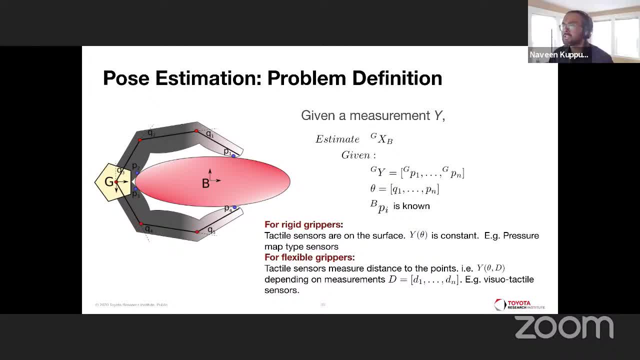 y is. let us say, we have a perfect knowledge of the kinematics of the gripper and somehow some kind of tactile sensation is giving you, let's say, just on off, measurements, and it's able to tell you what each of these points are, the points being p1, p2, p3, p4, where contact is happening between 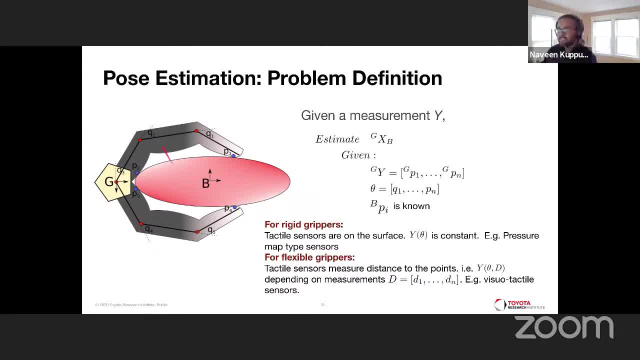 this surface and this surface- let's now consider it's a rigid case. the fingers don't comply, the object is rigid, so they are discrete contact points here which we are dealing with now, in these discrete contact points. if i were to know the location of each of these points- p1, p2, p3, p4- in the reference frame g, you have this nice neat. 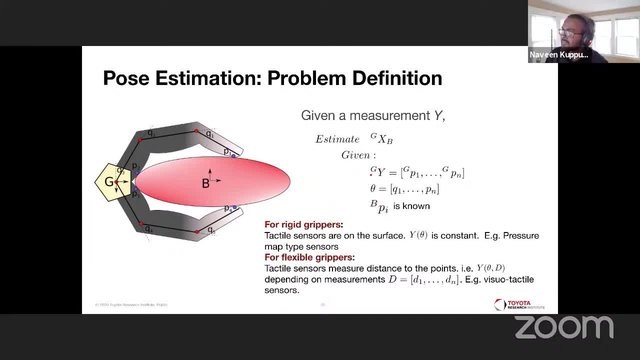 measurement set gy uh. the qualifier for this measurement set, of course, comes through these observations, which are the kinematics of the robot coming in through the encoders, kinematics of the gripper. so the set q1 and so on. i think that's a typo. that should be qn. 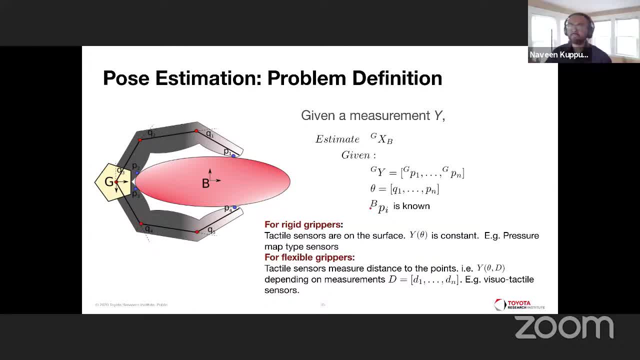 here. and let us say we know the object model. we are not talking about trying to guess the pose of a completely unknown object. we somehow know what is the complete set of points in the object reference frame, which is every possible point on the shape of this, on the surface of this object. 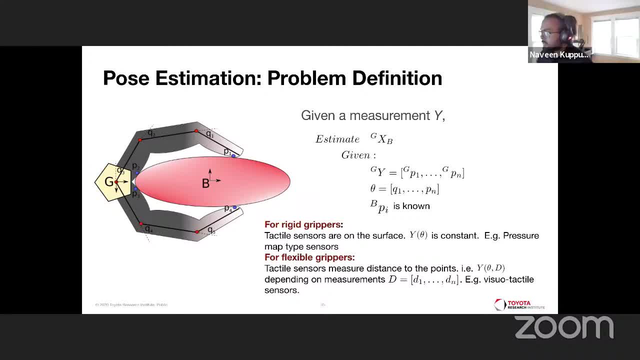 and surface is an important aspect. so for a rigid gripper you can say: the tactile sensors on the surface are the contact points, and y of theta is a constant. in other words it doesn't quite depend on how much pressure you're applying on the contact. the set of contact points are the same. 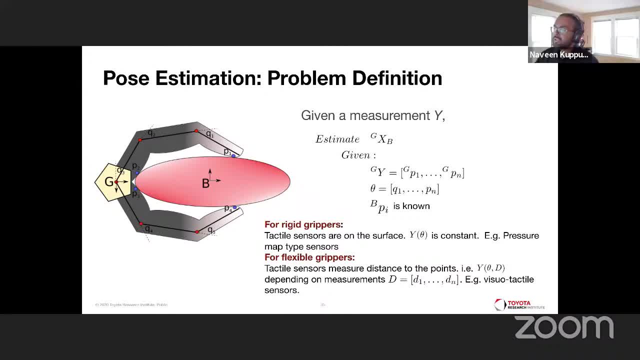 regardless how much pressure you push in into each of the contacts. so we'll talk a little bit about flexible grippers later, but suffice to say you have a contact surface, not discrete contact points. but you could also sample on that surface and obtain a similar set of measurement points. now 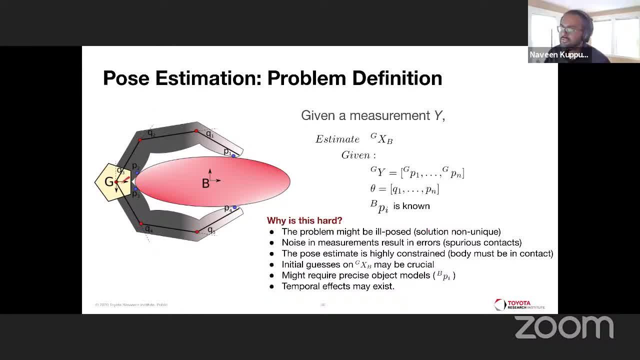 we can ask the question: estimate g x b, which is the pose of this object in my reference frame g? now we can ask the question: what makes this problem particularly hard? so, first and foremost, it's an ill-posed problem by its nature. there is a non-unique solution. if i simply gave you. 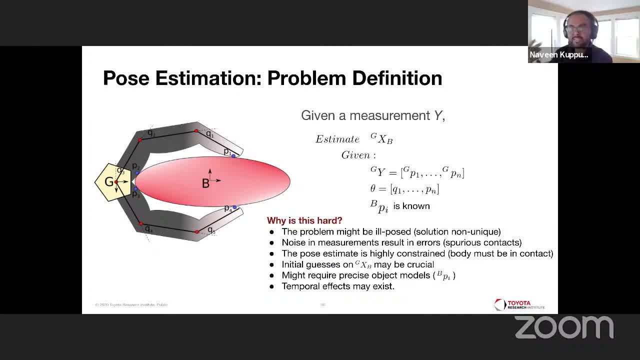 these given parameters and asked you to estimate gxp, there could be several possible poses of this object which satisfy this set of measurements. noise, of course, can heavily affect us, because our notion of where these points are comes entirely from the idea that a tactile sensor has said what the points are: p1, p2, p3, p4, perhaps a neighboring? 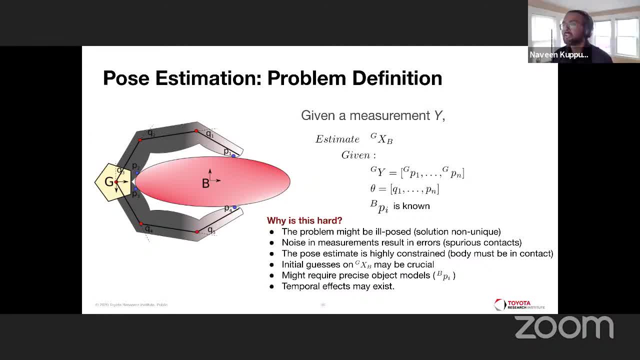 tactile sensor fired when it shouldn't have fired because of sensor noise, then our sense of the set of measurements y would change and that can confound us. second, the pose estimate is highly constrained and this is an important point. we are not talking about an object in 3d space. 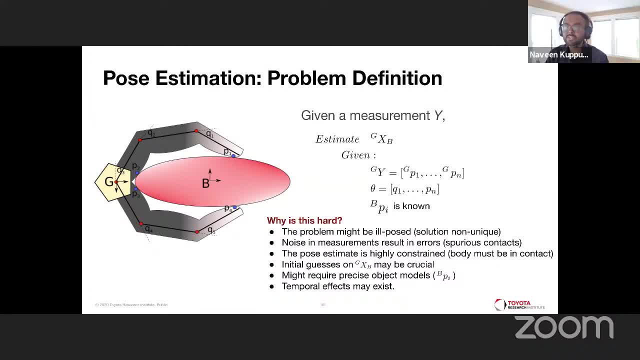 with nothing around it. the robot is in your gripper. so, in other words, the robot cannot be inside your gripper and cannot be away from your gripper. it is in contact, it's touching a gripper, and that's a hard fact that you know. so we should uh think about how that that constraint affects. 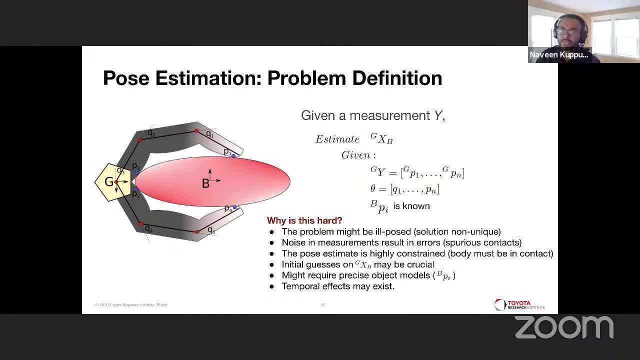 our pose estimate. the initial guess may be crucial- and this is something we already know of in other kinds of post estimation problems- and it might require a pretty precise object model. how much of the object knowledge do you need to know? that is the set bpi. so how much, at what resolution, do you need to know the object itself? 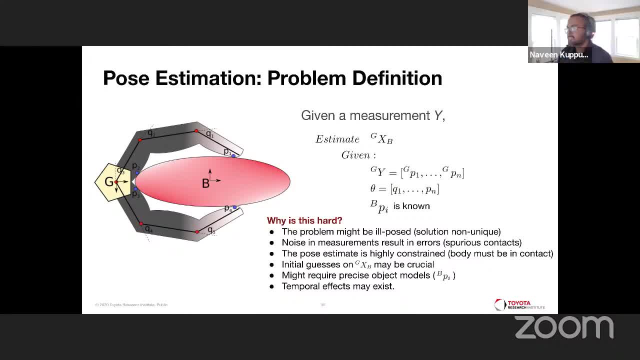 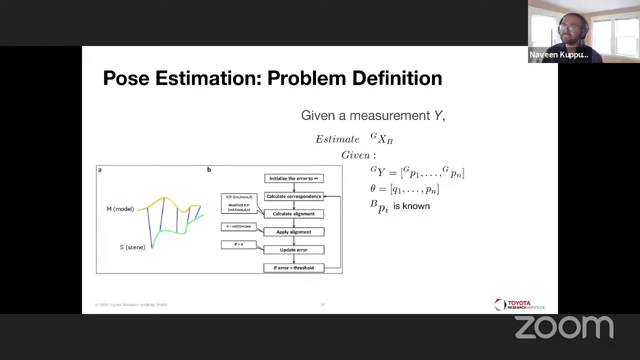 in order to perform this action and, of course, with a tactile sensor, like any other sensor, there may be temporal effects. so this is related to the noise question in, as i mentioned earlier. so if you simply look at this problem definition, you notice that by structure it's very similar to. 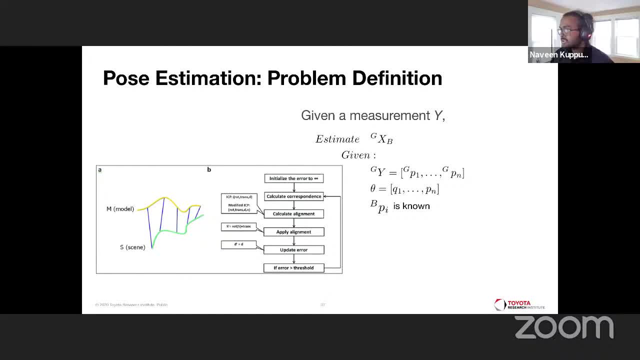 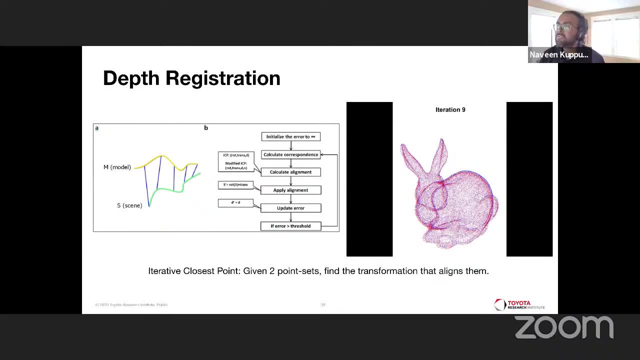 another problem which you have studied, which is, of course, uh, depth registration. so you have a model, you have a set of measurements and you're asked to find the transform between your scene and your model, or the other way, depending on how you post the question. so all of you know the 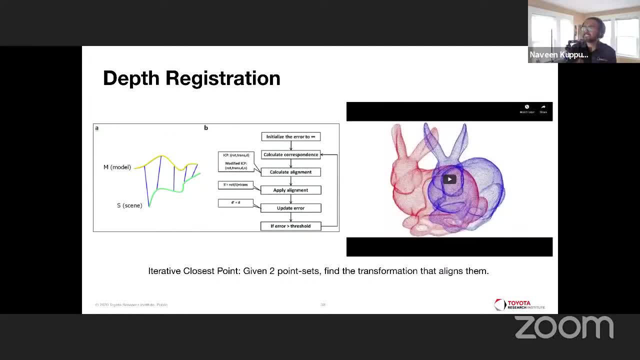 stanford bunny, and russ mentioned that you have even done that as an exercise. so uh, it's. it's not too hard for me to explain what is it that we are trying to do. so the flowchart on the left is, of course, the steps of the well-known icp, or the iterative closest point, uh, algorithm. so which? 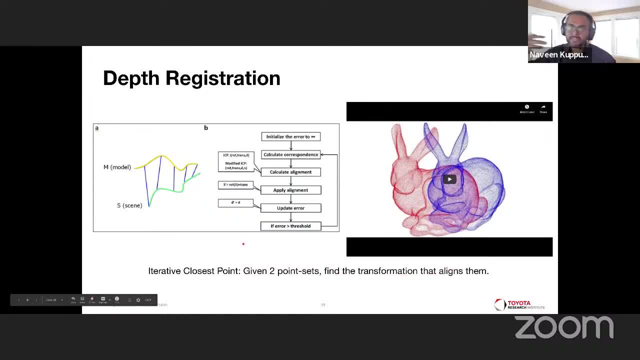 is called the linear distribution model and it's used to find the transformation that aligns them. in the simplest form, it's an iterative process of taking your set of points and finding, uh, the pose such that the distance to the nearest point on the model are minimized and you shake up the little. 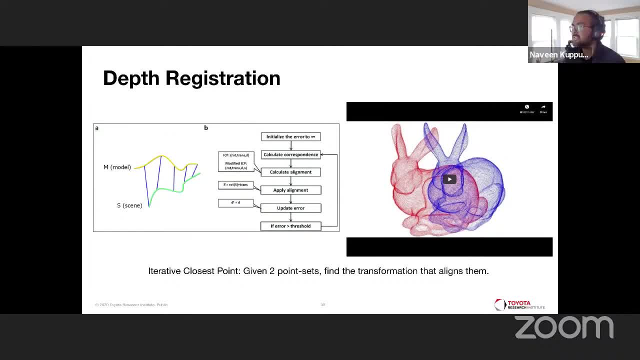 bag of points, uh, and you repeat the process. shake up the bag of points, repeat the process until you're satisfied that you hit the goal now. uh, in the case of these kind of dense jumping points. uh, in the case of these kind of dense jumping. uh, in the case of these kind of dense jumping. 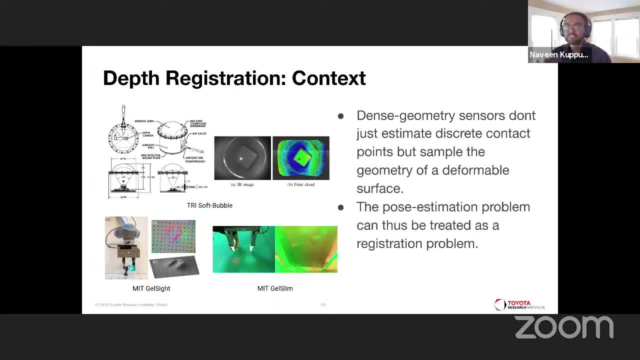 tactile sensors And, by the way, I should mention this, I will interchangeably keep using the terms camera-based tactile sensor, visual tactile sensor, dense geometry sensor all to mean the same thing: The camera inside a soft structure which is going to go make contact with the 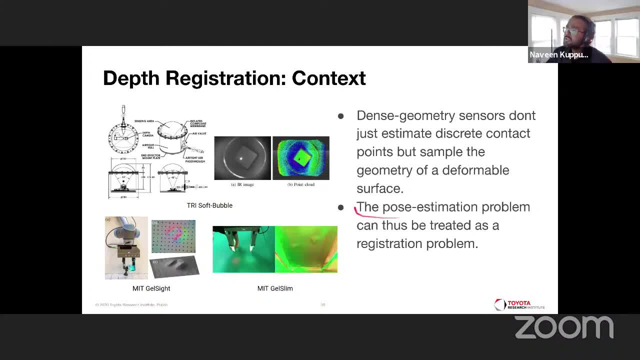 surface. So dense geometry sensors don't just estimate discrete contact points but sample the geometry of a deformable surface, So the whole sensor surface deforms and you sample that structure in discrete locations. but the sensor itself makes contact continuously with this object And the pose estimation problem can thus be treated as a registration problem. 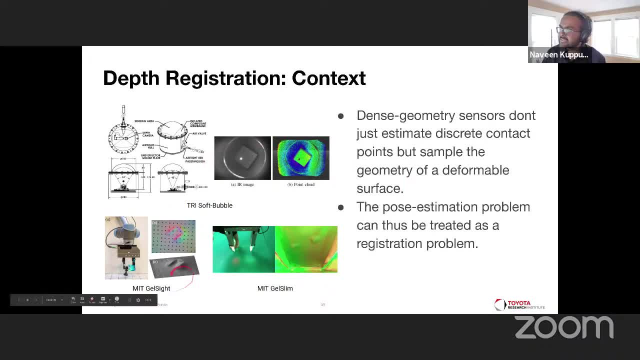 And I have illustrated the depth maps coming from each of these sensors here, just for you to visualize what it looks like for a sensor to actually go touch an object and obtain a depth map. Now, this was one example of us performing this kind of depth registration using an early 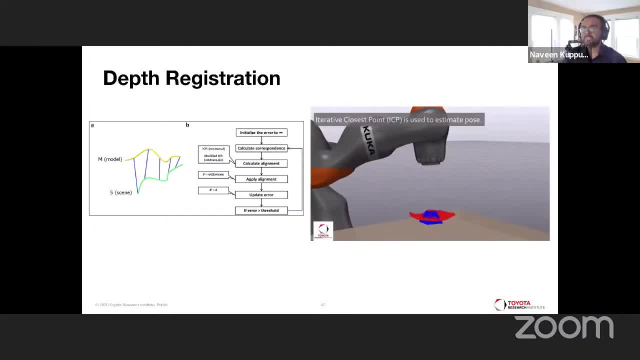 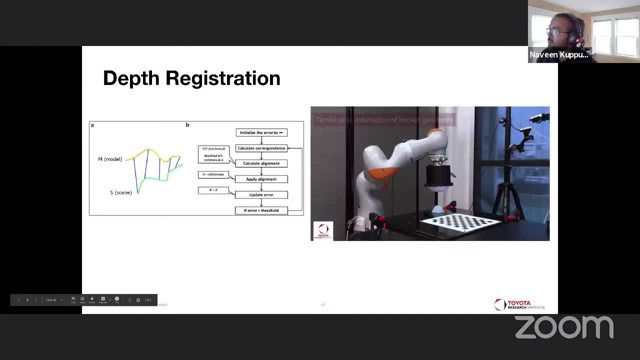 instance of the soft bubble sensor. This was the bigger format which was at the end of the arm. That image you see here is the ICP fit of trying to figure out what is the pose of this known simple geometry, which is that of a. 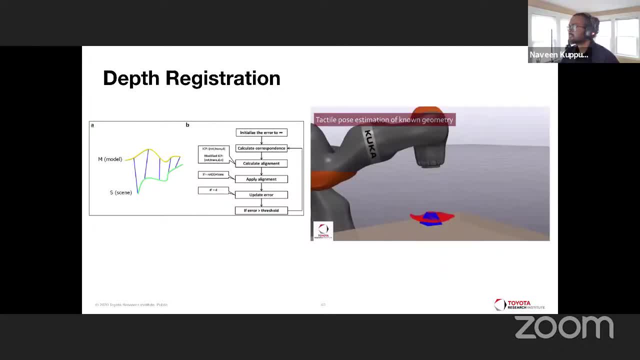 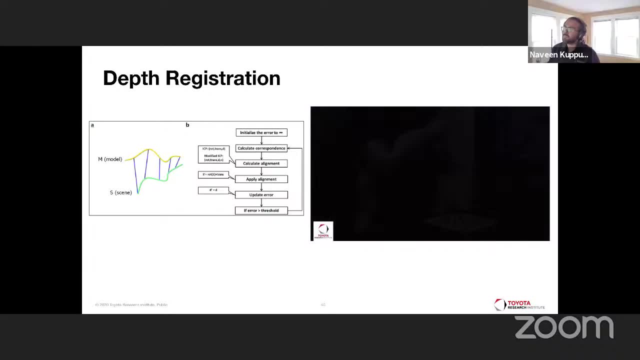 tetrahedral. what is this called? Wait, I suddenly forgot. the name of the shape Doesn't matter. You touch the shape, you have a known model of the shape. we, incidentally, 3D printed shapes so that we know exactly what is the shape. 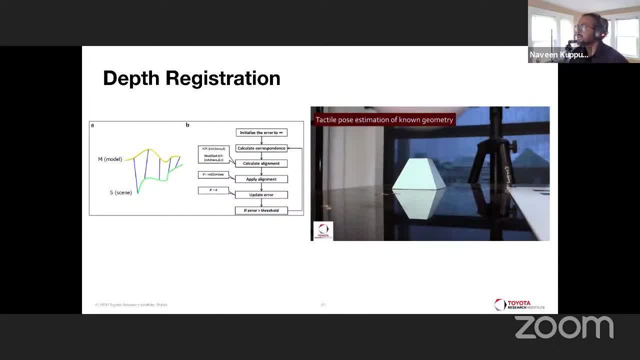 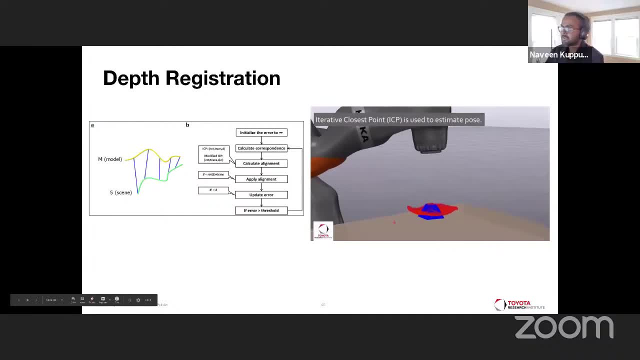 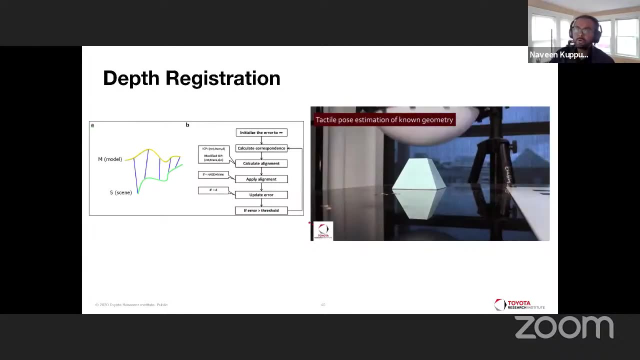 that you're trying to make contact with And from this contact you have this point cloud obtained from your sensor itself. in red and blue is the fit of the sensor, of, fit of the pose inside the sensor measurement. And the interesting point is your, all your measurements of, or all your? 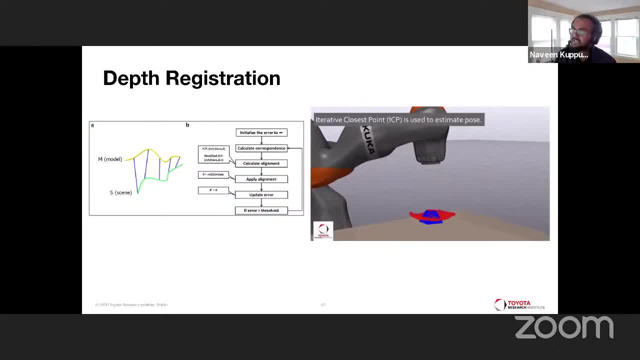 computations of pose estimates through the depth registration technique would effectively be computations of the pose in the camera frame of the instrument. And that's what we're going to do, And that's what we're going to do, And that's what we're going to do, And that's what we're going to. 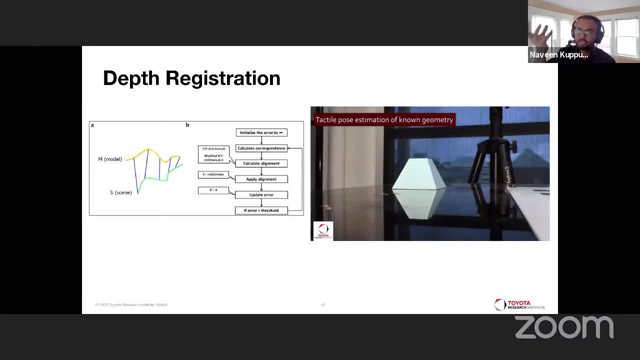 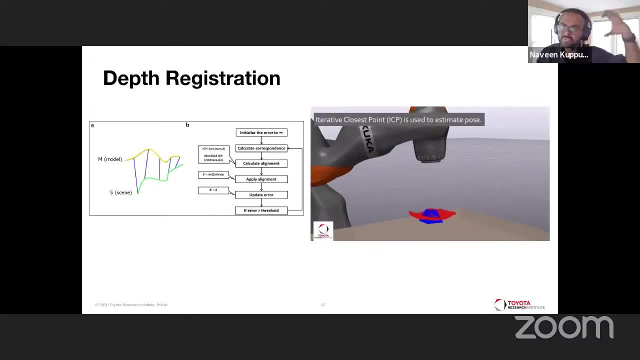 be using to look for beweging of the embedded camera. In other words, you're computing everything between your local gripper frame, which is why I would call this an in hand pose estimation problem, as opposed to a global pose estimation problem from an external camera or so on. Now, what makes this? 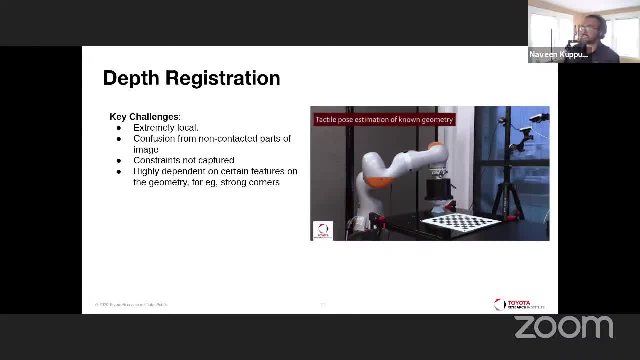 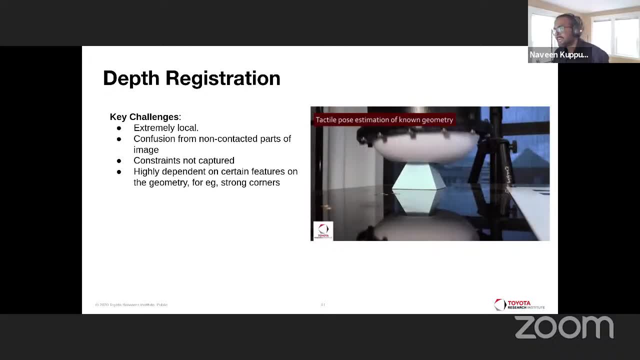 Now, what makes this problem hard? that was a nice neat demo. you see that I'm showing the result of. That was a nice neat demo. you see that I'm showing the result of performing that. well, it turns out it's actually a pretty annoyingly hard problem because there's several effects which make this. 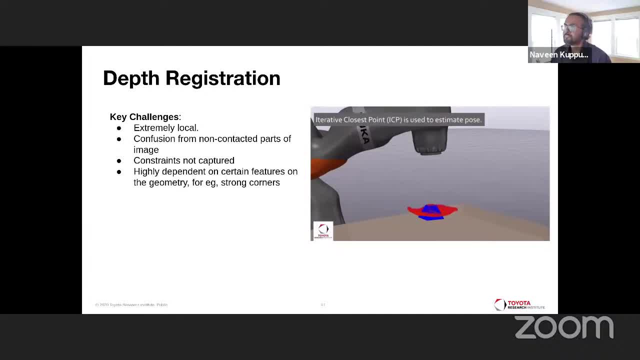 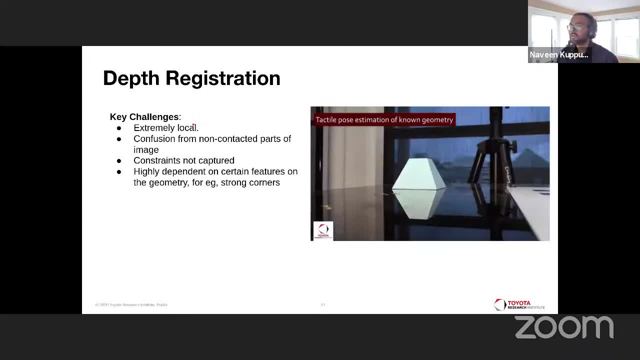 out of that's an in hand position estimation or an in duration information problem falls more like a really tricky One. you have dealt with in your own lecture. This is a really local problem, So you need a really good guess somehow. Second, you may often have confusion from non-contacted. 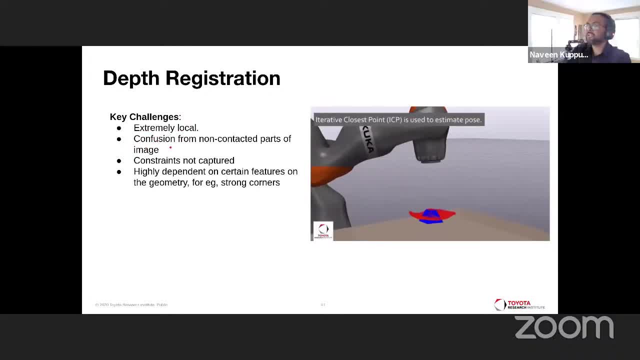 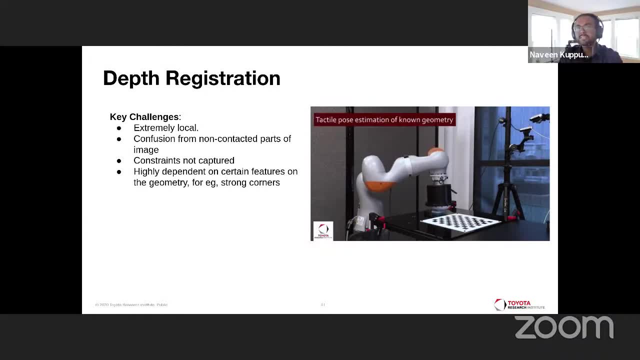 parts of an image, because here's another little distinction between a tactile sensor and something like a camera-based sensor. A camera can quite often treat pixels as independent. You can treat parts to the scene which are not looking at an object as being completely independent to the. 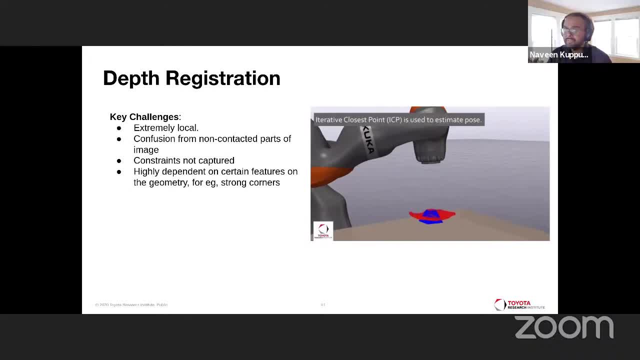 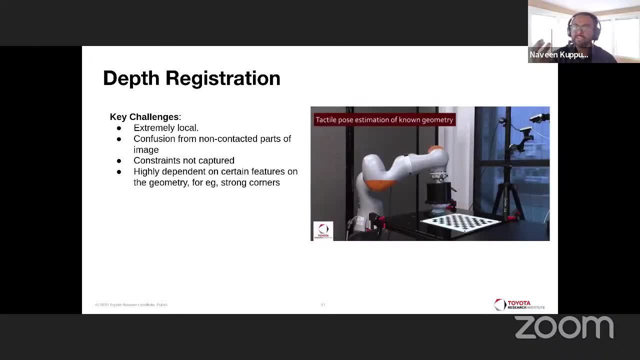 actual object, Whereas tactile sensors can deform everywhere. So if you're simply sensing deformations, you're looking at every part of your image changing a bit, but actually what you want to pay attention to is only the part in contact with your sensor. So that makes it a little bit. 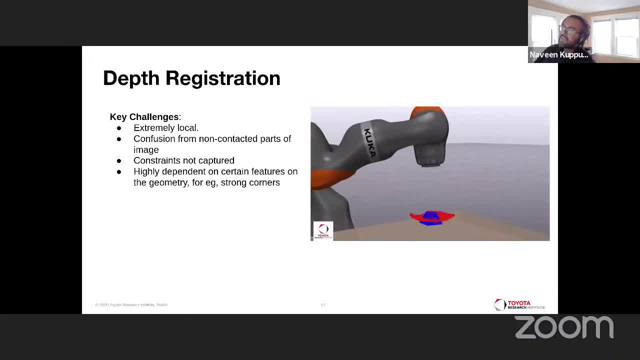 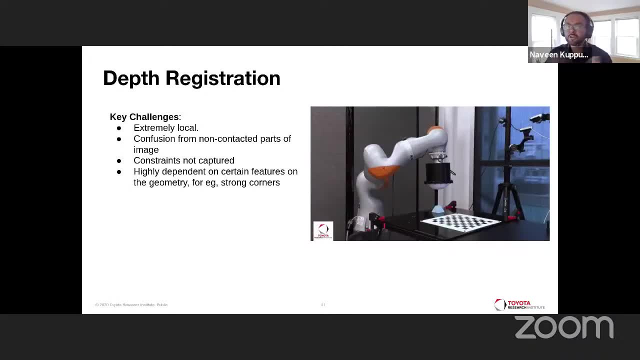 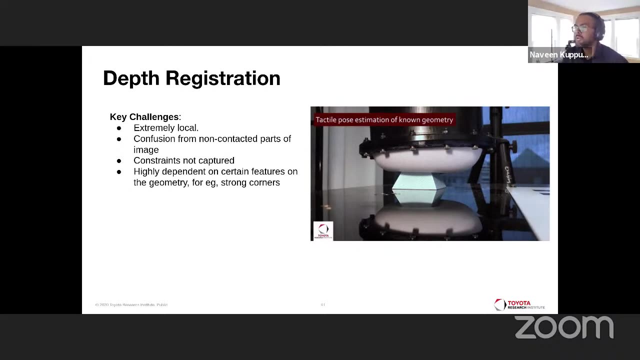 more tricky Constraints are not captured in a vanilla ICP formulation. So what are the constraints I mentioned? The object pose cannot be inside your sensor. The object pose cannot be away from your sensor because the contact has happened at the sensor surface. That is one hard fact that you know. And lastly, if you were to use 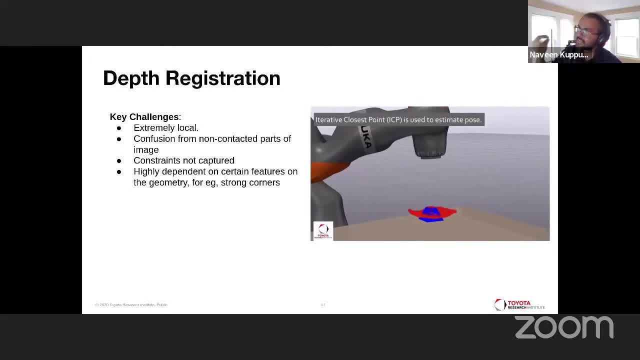 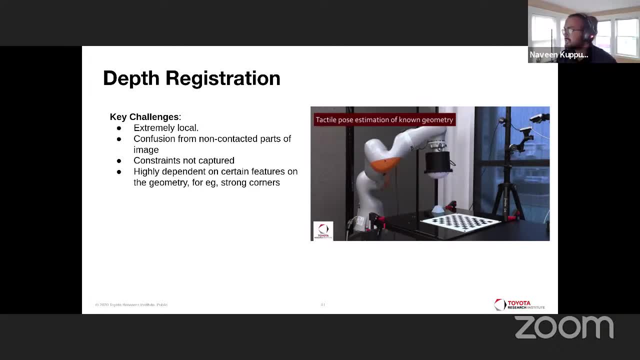 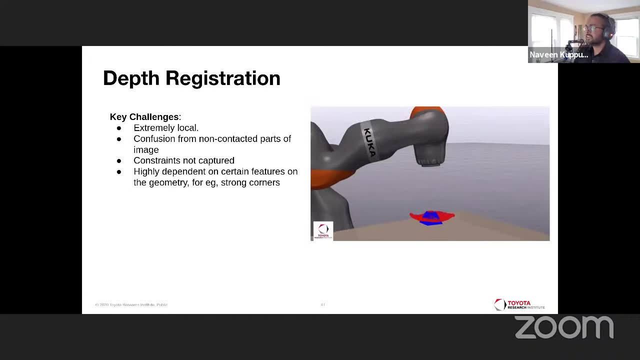 these kind of straight, direct depth registration methods like ICP, you tend to be highly dependent on features, on the geometry itself, like corner features and so on, And that- oh, now I got the shape. It's called a pyramidal frustrum. So with these pyramidal frustrums you often have these. 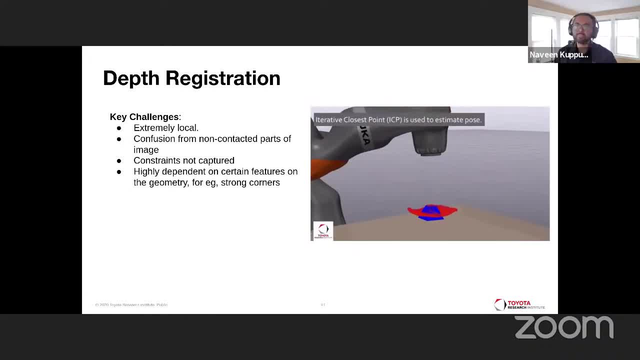 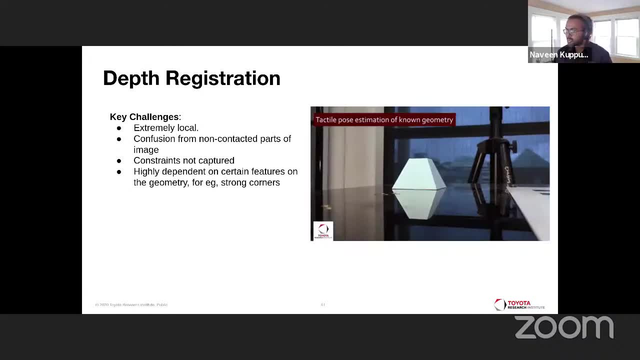 nice, convenient features like corners. So this was a cherry-picked example intentionally to show you how ICP can work. If I were to pick a shape with all kinds of weird topological features, perhaps ICP may not converge smoothly. So let's try to break this down and think about how we can improve. 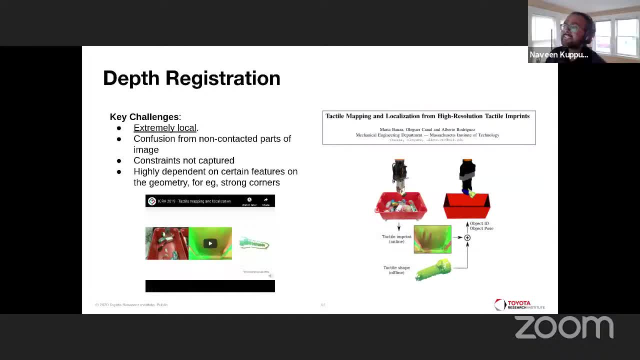 our pose estimation. First, let's tackle the question of being extremely local. Now, this is one example from literature out there. This is from Alberto's lab, where they used a pretty straightforward way to guess what is the initial condition. So let's say: you have, this is a very close estimate which we want to then infer the pose estimate. 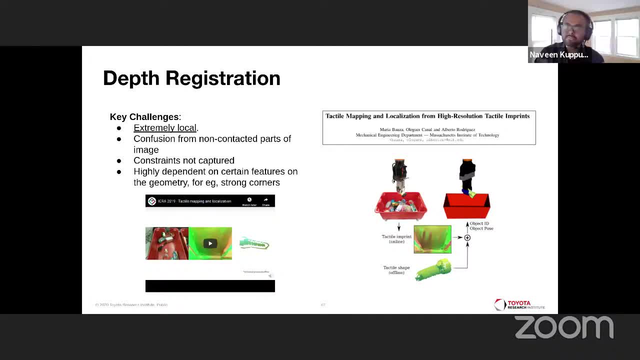 So, in other words, if you are very local, perhaps we need a guess which is close enough. And what's the technique we all love these days? Let's throw a deep network at it. So, and it turns out it's quite possible using a network. In this particular instance, what they did was to obtain a whole set. 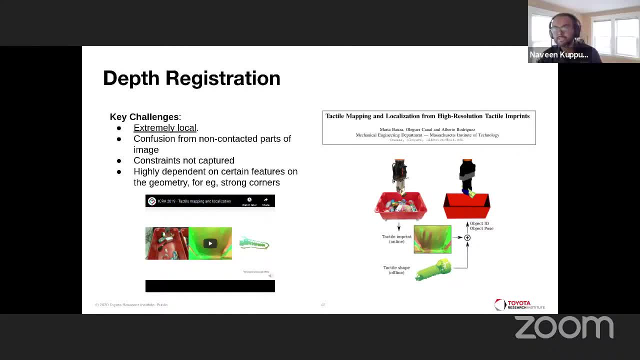 of tactile imprints, quite similar to the classification example I spoke of before, And from these tactile imprints, what they did was they asked the question of what is the initial condition of this. we would like to know is an initial guess, for what is the closest tactile imprint to the imprint I 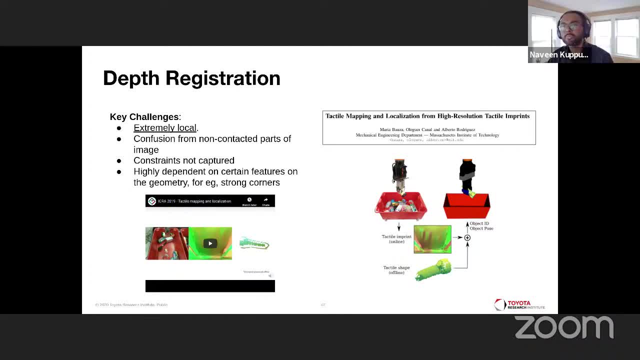 have right now, which is something like an image matching problem. I'm giving you one image and asking you to find the image in my corpus which closest matches this image, And from that you immediately have an initialization of the pose of this object which you can then use to initialize. 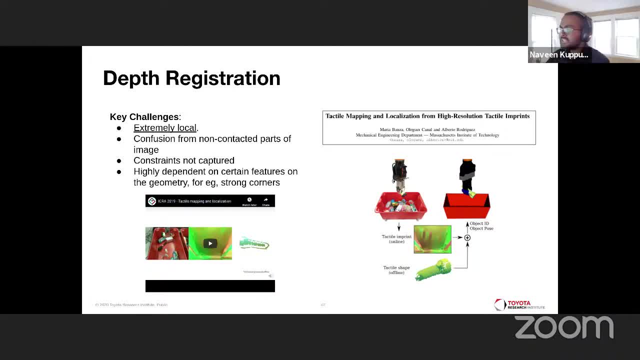 some ICP style technique. So this I would suggest let's watch the video briefly while I continue speaking. But you essentially have these kind of tactile imprints from holding these objects. This is the Gel Slim tactile sensor- And from these tactile imprints. 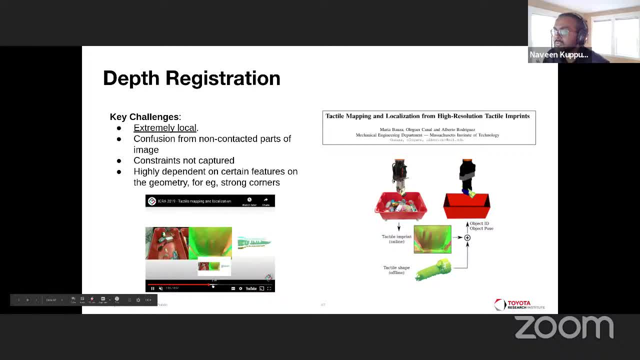 we are able to then pre-initialize and then perform some kind of pose estimation which is a bit more robust to the initialization error. The other way of getting over this initialization error is also if you use the vision-based technique to actually go in and grasp an object. perhaps your initial pose before you made contact is a good enough guess. 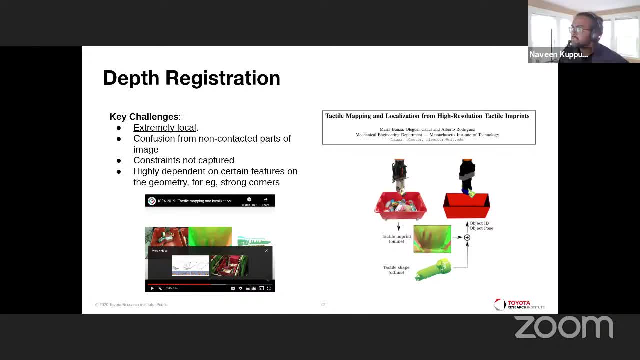 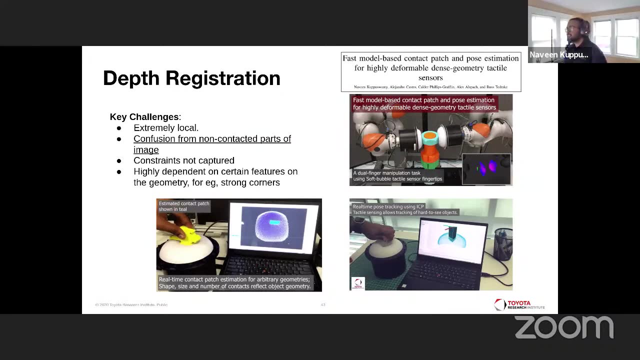 for where contact actually happened. So that would be the other way of inferring this. But that is assuming a camera was looking at your scene before you made contact. So let's pick out item number two, confusion from non-contacted parts of this image. So 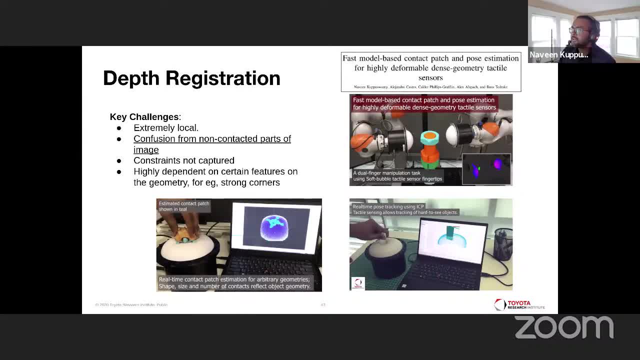 in some sensors, for instance the TRI soft bubbles, you have deformation which happens all over. So what is this particular soft bubble sensor? It's a time-of-flight sensor embedded behind this little balloon. It's a stretched, elastic membrane. It's an air-filled chamber. 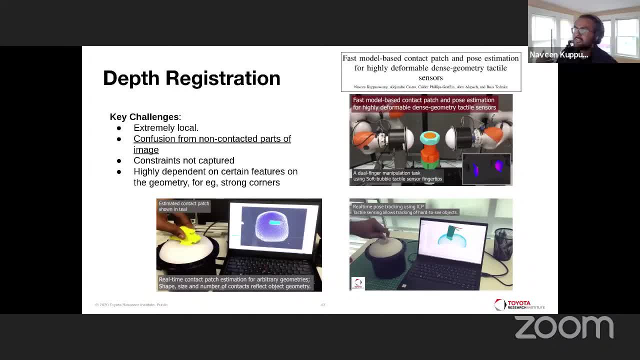 So it deforms exactly like what you expect a balloon would deform. It's in fact a latex membrane And as you're pushing into this latex membrane, you have these depth measurements. So the whole membrane therefore deforms when contact happens And therefore it's important to try and resolve. 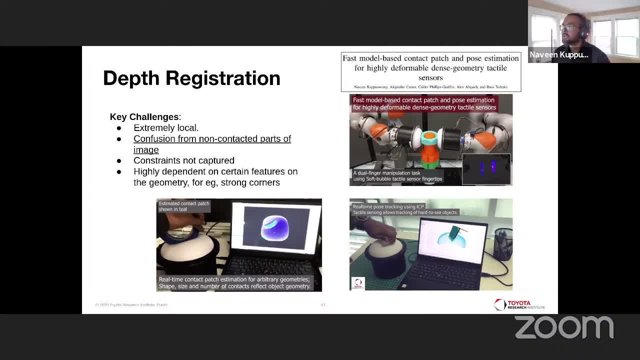 this confusion between the non-contacted and the contacted part of this image. Now, how this was solved in our work was something I'll briefly talk about in greater detail later, But for now suffice to say there's a lot of number crunching which goes on, which try to understand how a 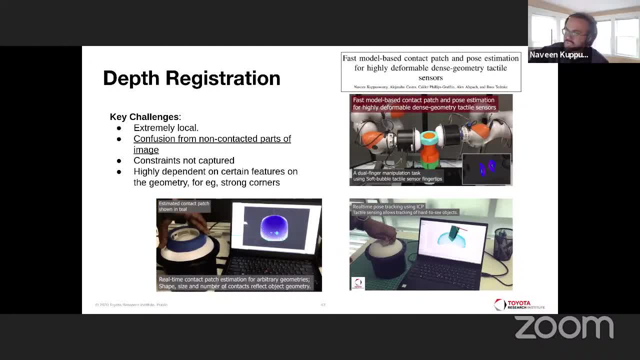 membrane deforms when contact happens And through this prior model of understanding how deformation happens on this membrane, you can then ask an inverse question, which is: if I gave you a bunch of measurements, what would be the most likely subset of measurements which resulted in that? 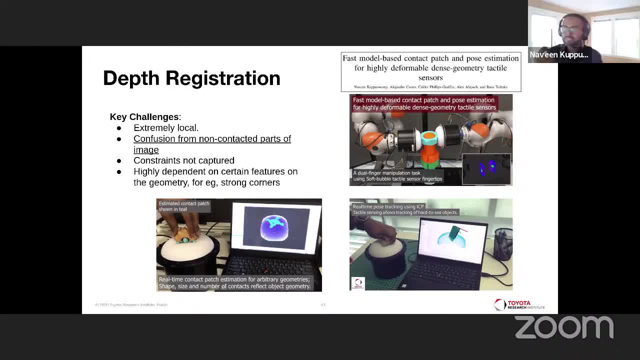 deformation on this object surface, Which is why it's an inverse problem. The forward problem would be if I gave you an object and I gave you this membrane, tell me how this membrane deforms. And now we are asking the opposite. I gave you a bunch of measurements. What would be the possible? 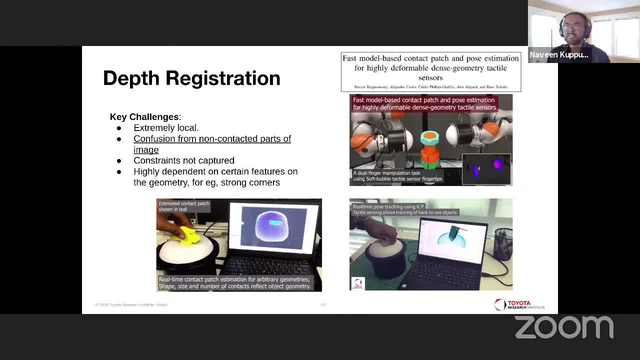 set of deformations which resulted in this membrane deforming, And that gives us a concise set which we call the contact patch, which is a part of the tactile sensor's surface which is in direct contact with this external object. So from this contact patch, 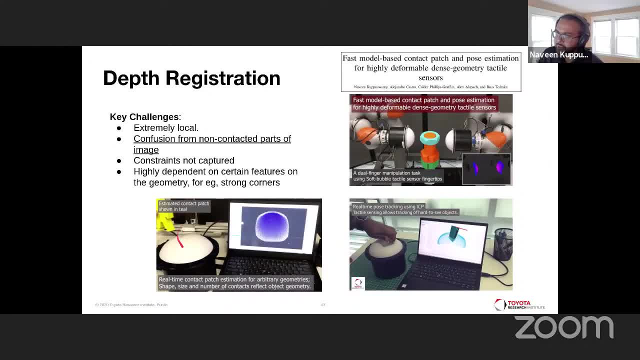 what you can do is so you're seeing in this particular video here, live tracking of the contact patch as I'm pushing in different objects into the surface of the sensor And you'll notice there are some features which are missed and occasionally there are holes. 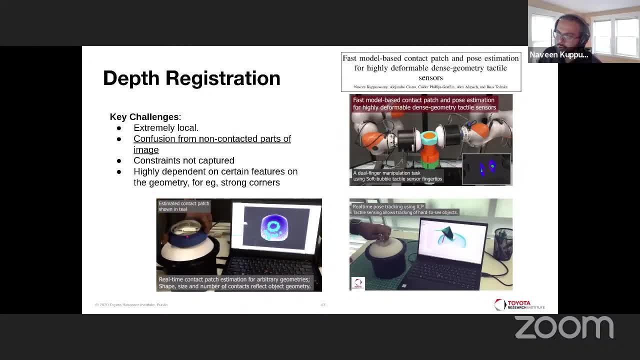 and other issues, but for the most part it is able to quite nicely capture the shape of this object. For instance, it's able to discriminate that the inner surface of this tape wasn't really part of the patch. Same was for the gap between the feet and so on. And if I were to only use that part of 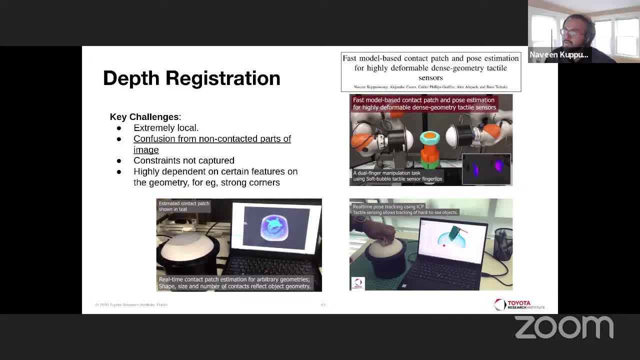 the scene for doing pose estimation. that would be a lot less than the space between the feet, And so I have a much more culled set of points. Now, an equivalent in a camera-based world would be to use some kind of masking. 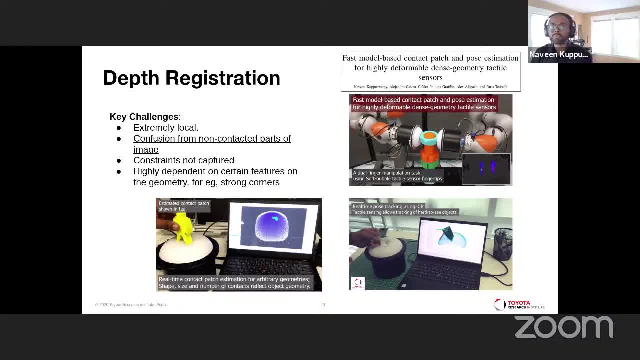 And I know that you have gone through the mask RCNN problem, So perhaps the closest analogy for performing this is to simply take an image mask, use the depth values coming in purely from the mask and then using that to perform your registration, And it turns out that leads to some level of robustness. 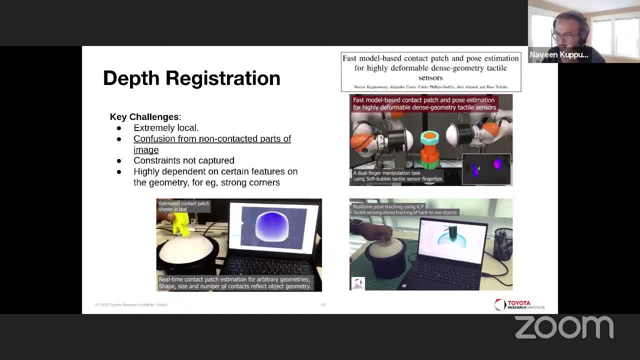 from this confusion with the non-contacted parts of the image. It doesn't quite solve the problem yet, but we now have two possible solutions to this tricky challenge. Any questions at this point? Just have to give you a time check. I know you have so much more material. 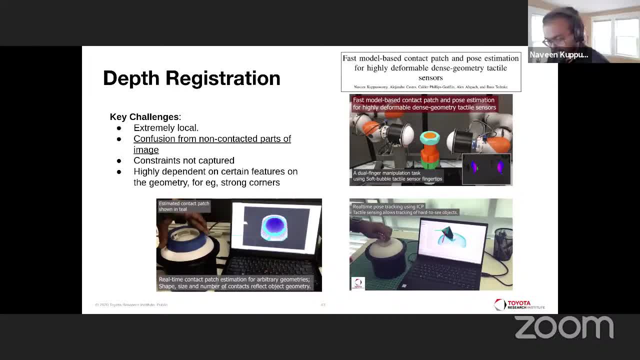 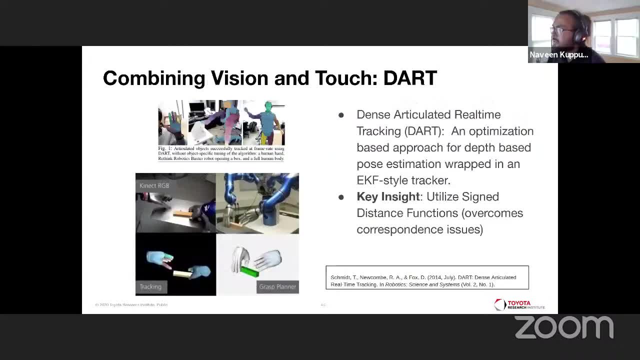 but we only have a few minutes left, So just make sure you're watching the time. Okay, I did slip my mind, So let's jump ahead Now. this part I don't quite need to get into great detail because it has been covered in your previous lecture. 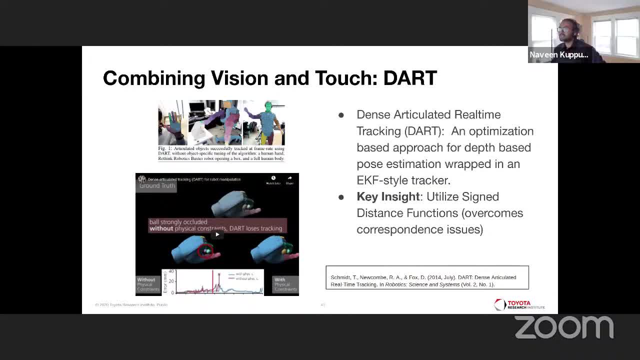 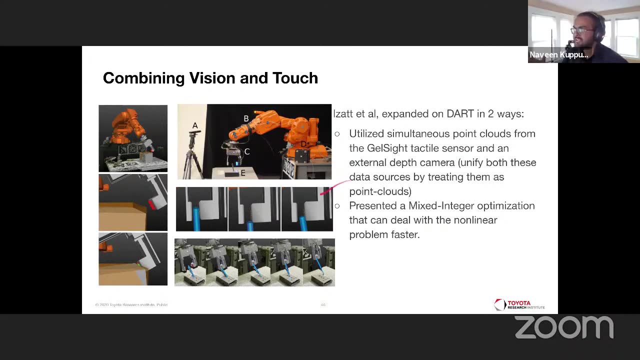 which is, of course, performing some kind of DART-based tracking. Now, the key insight here was to utilize the so-called sign distance function to overcome correspondence issues. Now I really want to focus on one little trick to enhance what we have seen in DART. 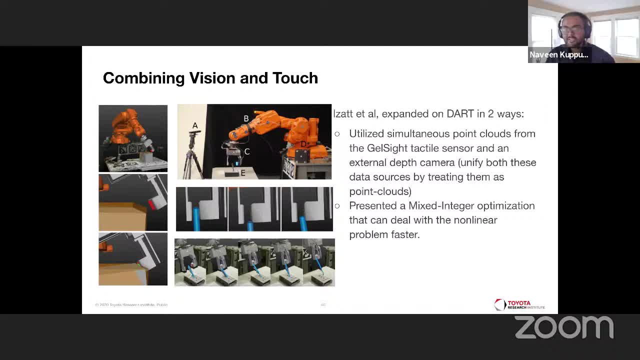 So take the gel-side tactile sensor and see that the depth image is essentially something you can represent as a set of points in space, Because if you know the kinematics of your robot and if you know the gripper position at this point in time, 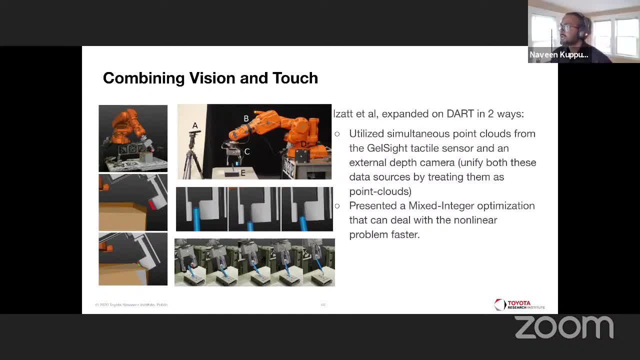 you also directly have a measurement of a set of points in space, And this is exactly what Greg did in his work, which is he utilized simultaneous point clouds And there were some mathematical issues he dealt with in speeding up this problem, but we don't need to get into those details. 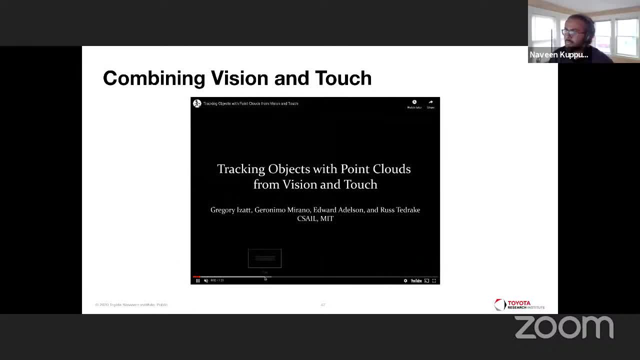 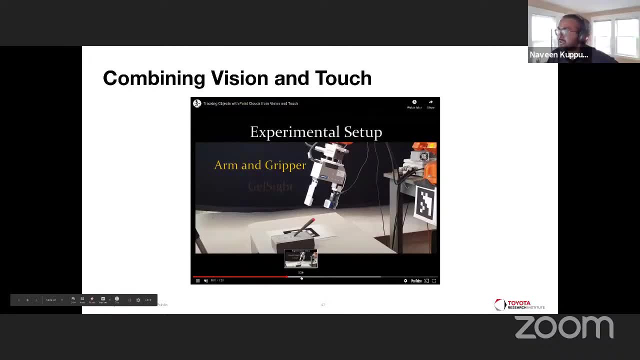 But essentially it comes down to combining depth images from your tactile sensor with depth images coming from an external perception system like a depth camera. looking at the scene will effectively lead us to do a DART-style optimization, which makes us more robust. 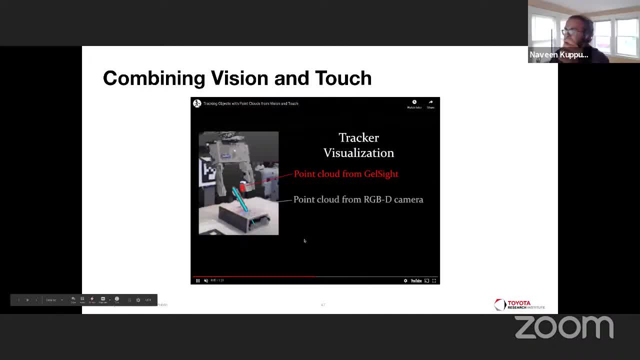 So that is literally what this problem is doing in this task of figuring out the pose of this pen-like object, a screwdriver- and inserting it into this hole. So I don't want to get into greater detail. I am running out of time, which I didn't realize. 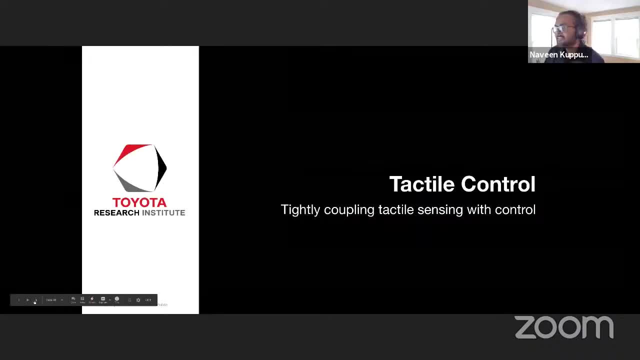 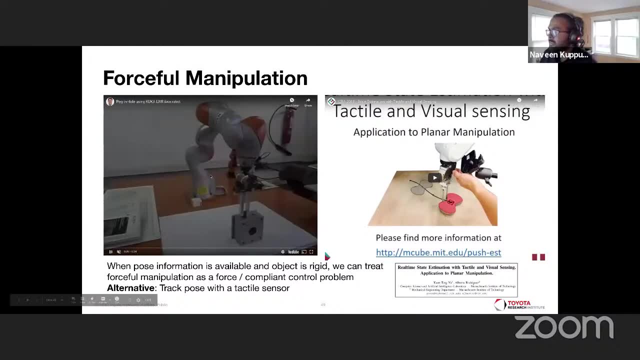 So let's now jump into the next part, which is let's jump into a few tactile control examples. Hopefully I can go through them Now. the first subset of examples: again, I don't need to repeat because you have already covered it. 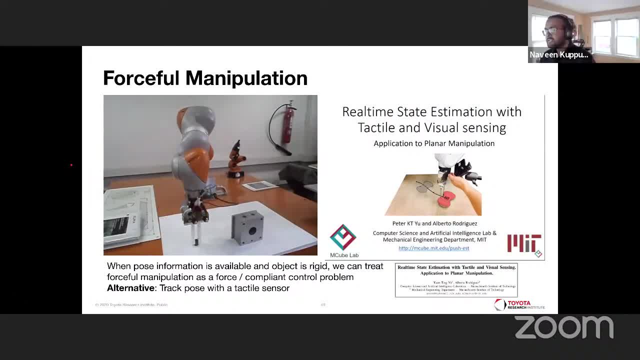 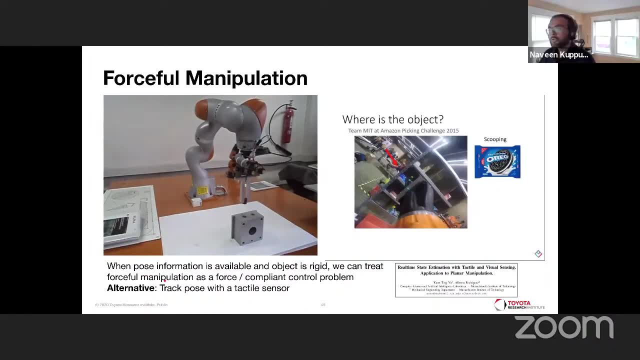 in a way in your previous class, When pose information is available and the object itself is rigid, you can treat it as a forceful manipulation problem, which is a force or compliance control problem. So this comes into some of the nomenclature. 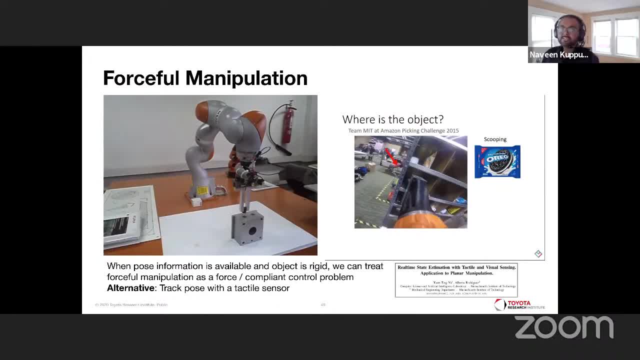 A lot of people tend to think of a force-talk sensor as a very simplistic tactile sensor. So if you were to perform some kind of force control or impedance control strategy, it's still for me a kind of tactile control. Now, if you did not have the pose information. 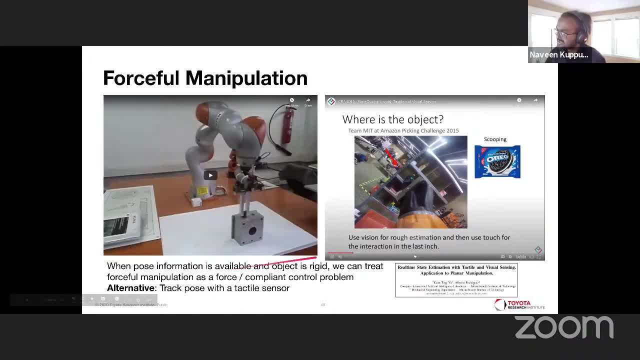 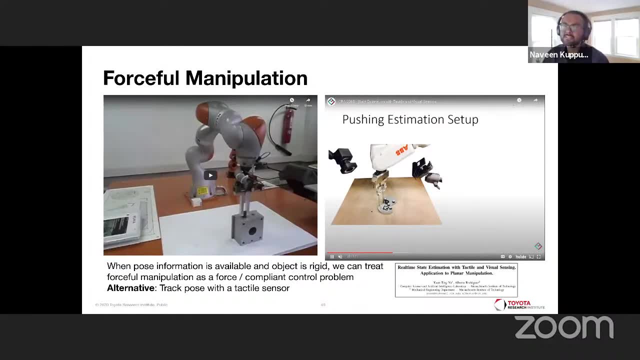 of this object a priori, you could enhance by doing some kind of tactile pose estimation. In this particular paper they combine an FT sensor with the camera instead of a dense tactile sensor with the camera track the shape of this object And in this case they are performing. 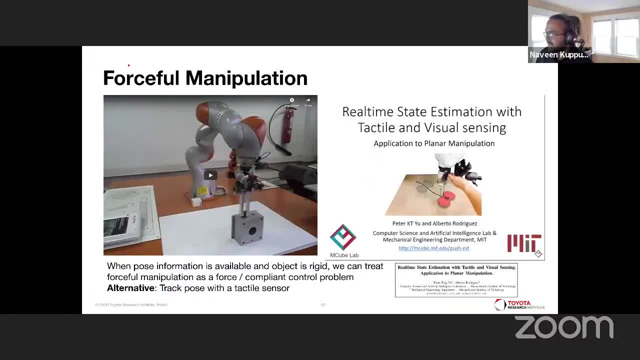 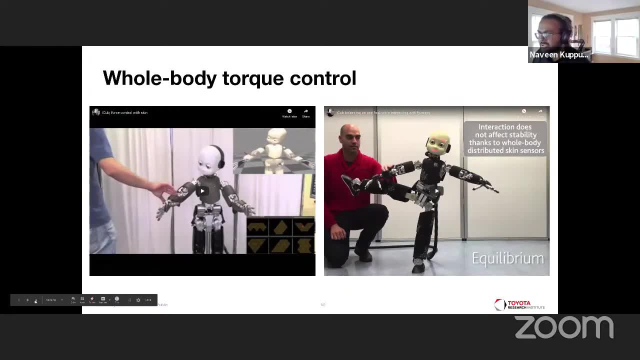 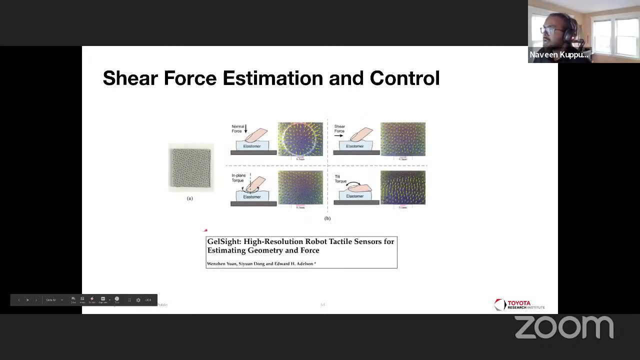 a task of planar pushing. But let's go really into the next example, Which is where I hope to have a little bit more of time. We can skip this for this particular instance, but the slides are available for you, Okay. 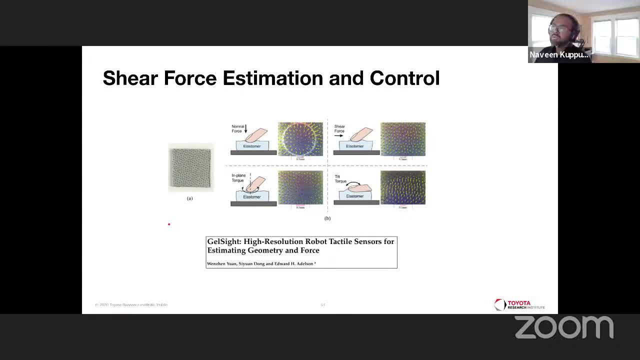 Now a lot of tactile sensors out there are now capable of tracking shear forces, And the technique they often employ is some form of markers on the sensor surface which moves due to external contact. You're now looking at three different forms of external contact and how they influence. 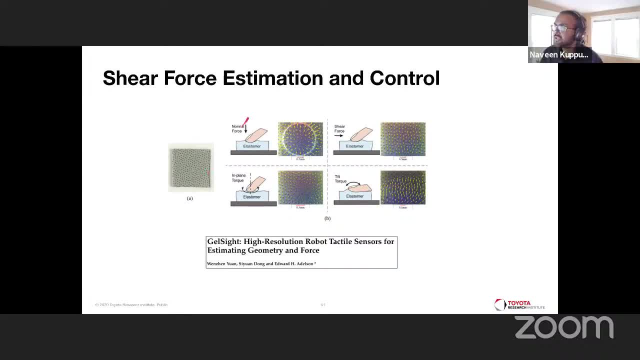 how these little markers, dots, are moving, For instance, in a normal direction, in an in-plane direction and in a shear and tilt direction. So this is from this work, from Gelsight. Now, how can we track the motion of individual parts? 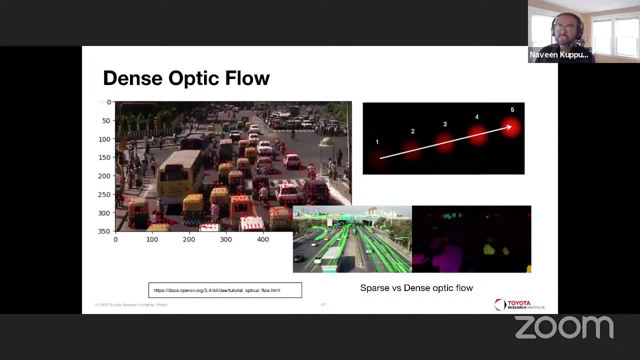 of the scene. Well, it turns out again in computer vision literature. this is a well-known problem which is known as optic flow, And optic flow, which I will not get into details right now, is simply trying to understand for a given pixel, which way is. 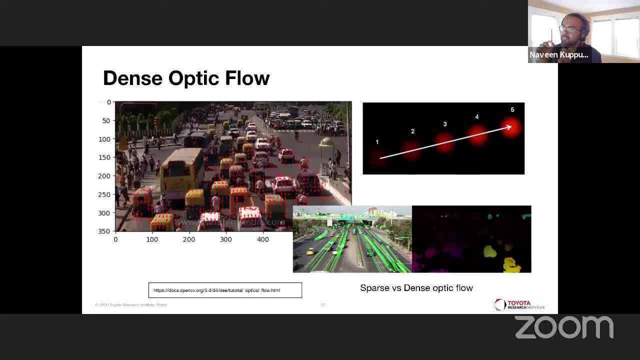 it most likely that particular pixel is moving, if I gave you a new image. So between two images, we are looking at each pixel and trying to guess which way that pixel has moved, And the power of optic flow methods is in a dynamic scene like tracking a road. 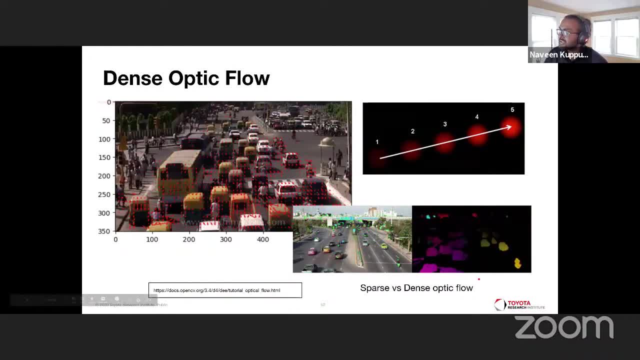 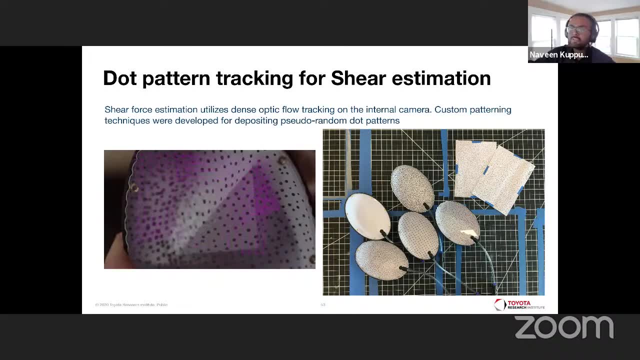 you can actually tell what parts of the scene have changed and in which way the change is happening. Now, in a tactile sensor like, for instance, the TRI software, you can actually tell what parts of the scene have changed and what parts of the scene have changed. 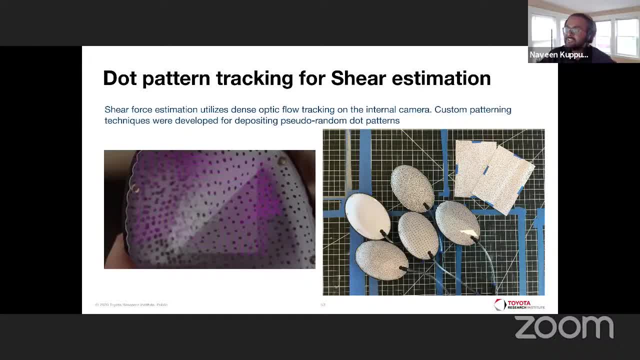 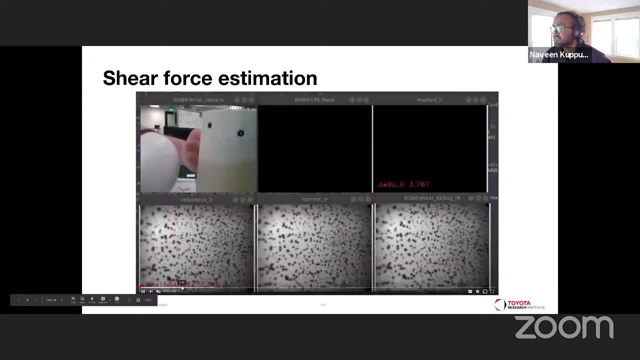 And in a soft bubble. the same principle applies. We have dots embedded on the structure. In this case they are printed on the surface And we can track the motion of these kind of dots. So this little video here is showing the tracking of these dots on this object. 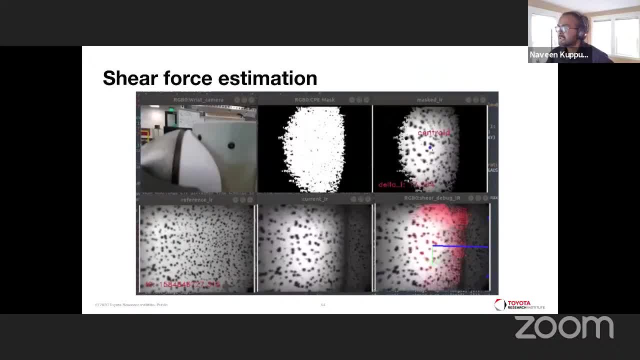 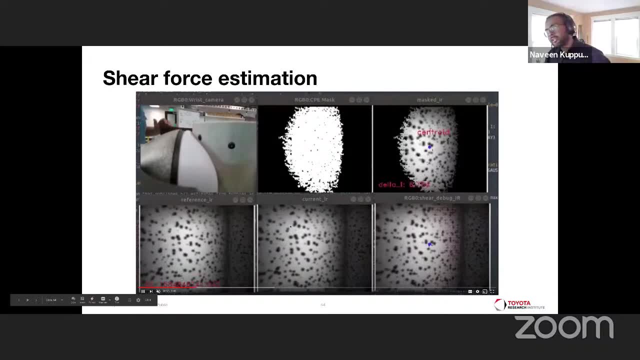 as we are going in and touching On the bottom part of the scene, you're looking at the different parts of the image, the IR images here. This is what's known as a reference image and a current image, And the distance, the optic flow is. 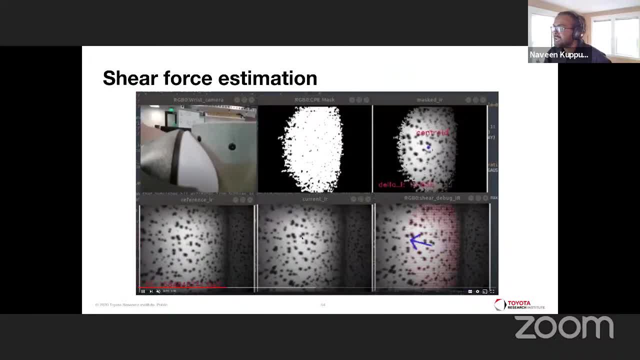 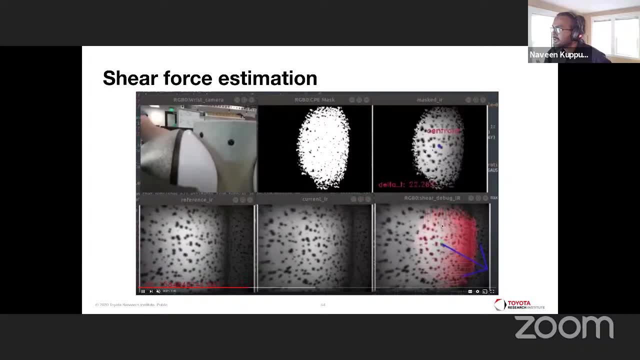 the problem of tracking each pixel in these two images how they have moved. And it turns out that simply by looking at the way each of these pixels are moving, you have quite a good guess of the shear forces happening as the person is pulling and pushing on this object. 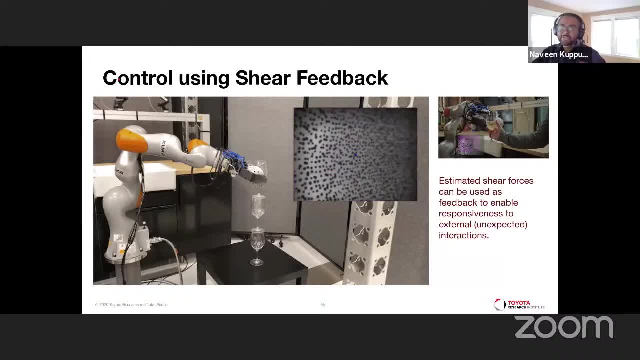 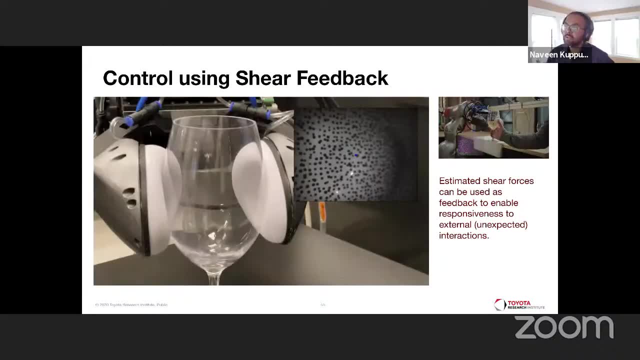 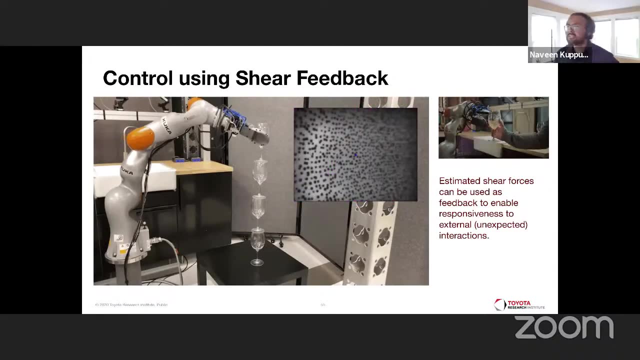 Now, what can you do with this information? You can do a pretty powerful form of control without really thinking and reasoning too hard, In this particular instance, which is a blind object stacking, and I intentionally picked these transparent objects just to illustrate the point. 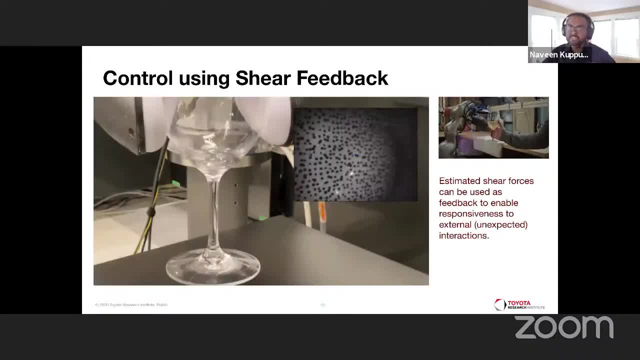 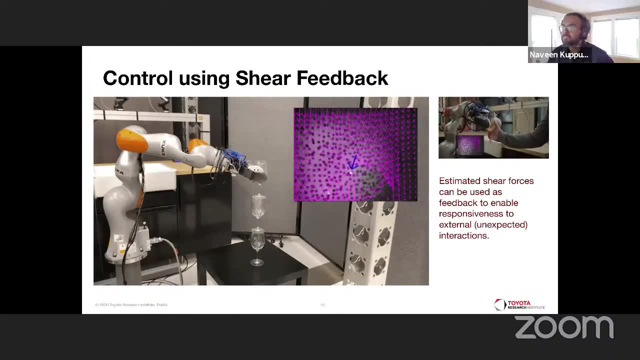 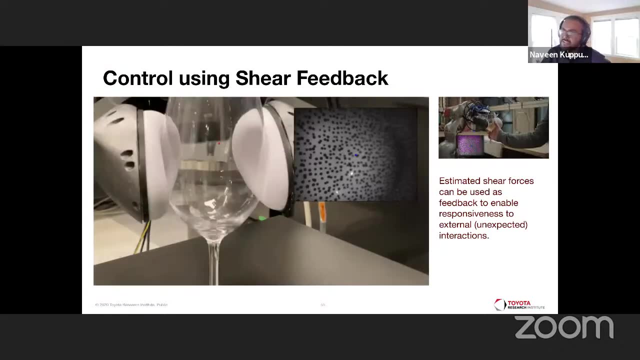 the robot is simply commanded to move downwards until sufficient shear is detected, and at which point it lets go, And it turns out with these kind of objects with flat surfaces and flat bottoms. it would just keep doing this indefinitely and leading to stacking. What was the controller which actually led to this action? 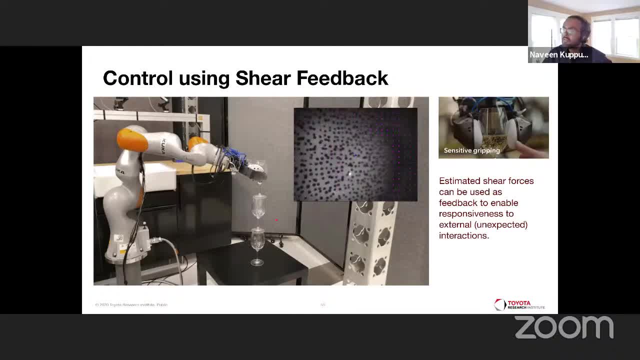 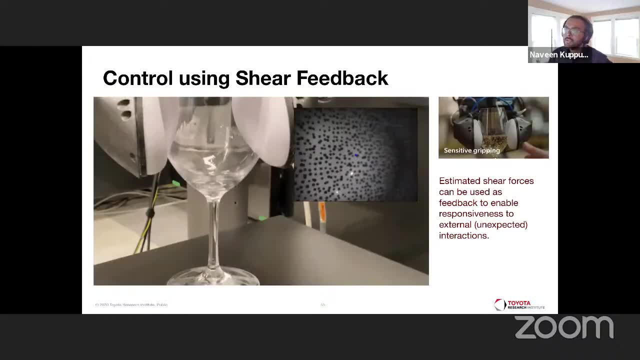 The controller was very simple. It said: keep moving until force threshold is reached, which is to say that sufficient shear has been detected. Now you could do this kind of an action also with the force talk sensor. That is not to say that. 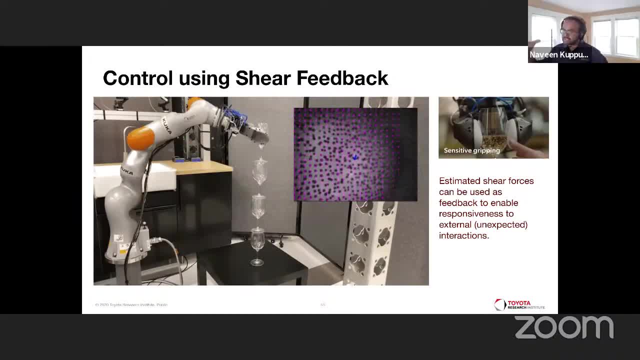 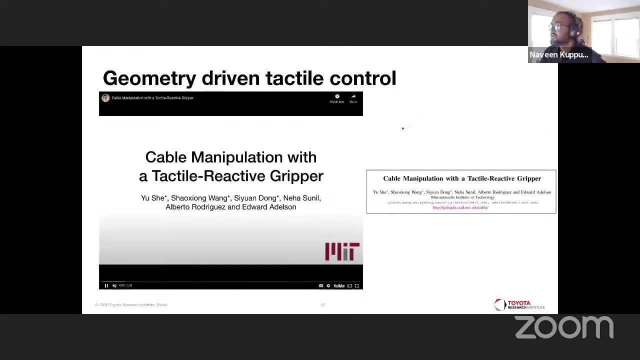 But in this kind of soft sensors you do have a lot more advantages in grabbing an object. So we are close on time, so I'm really going to try and run through. I unfortunately have to skip this example, But let's actually go into the outlook question. 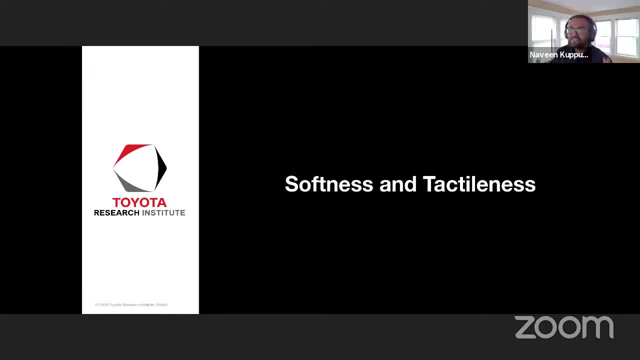 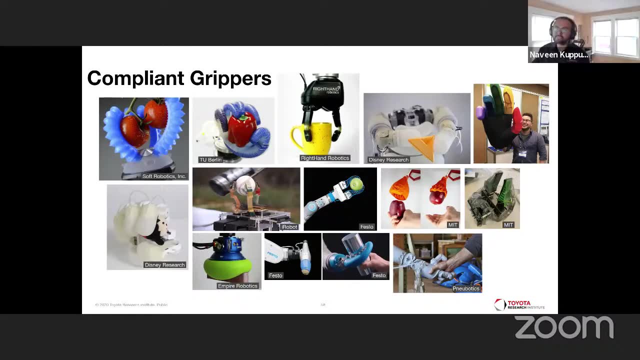 So there were two parts, One One: let's combine softness with tactileness, And that is indeed one of my take-home messages, which is: we have a huge history of compliant grippers out there, But why not combine both these stories of a compliant gripper? 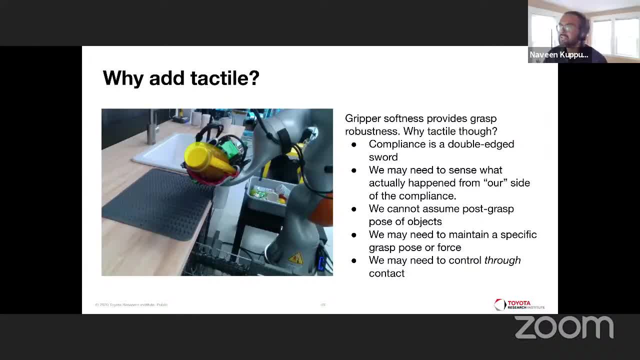 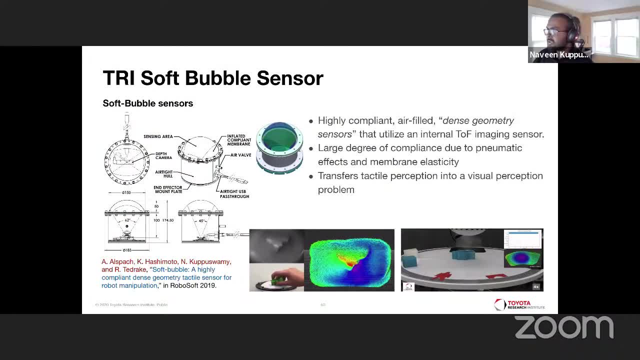 with a tactile sensor so you actually know what's happening in between your grasp and in between places, And there's several reasons why we would like to know that. which is kind of similar to our earlier story And again going back, the soft bubble sensor which 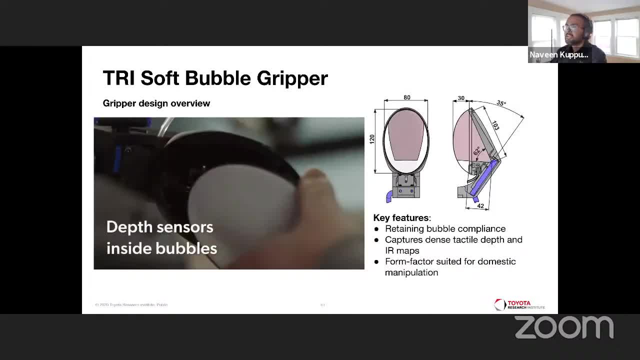 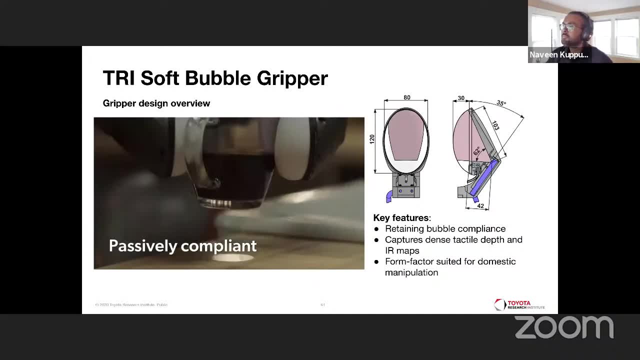 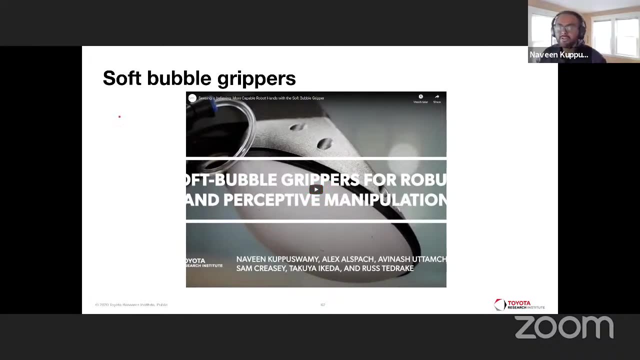 contains a membrane and this kind of depth sensor embedded leads us to perform these kind of tracking problems. So in this case this is a gripper form of the same sensor And I'm just going to leave this video out there for you will look at it again in the last slide. 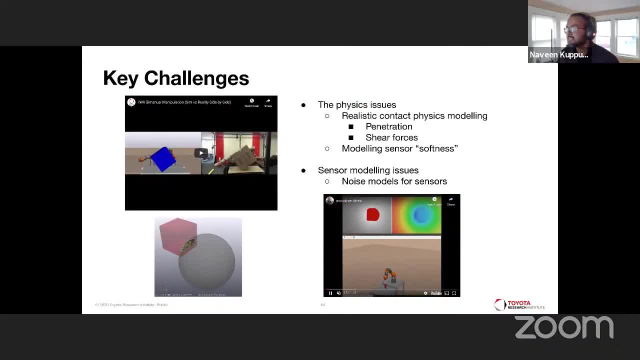 But let me preempt your question on simulation and just answer this part very quickly. How can we simulate a tactile sensor, Turns out, We have the vocabulary, but putting in the pieces together is very unique and dependent on the kind of sensor. In the example on the bottom right here: 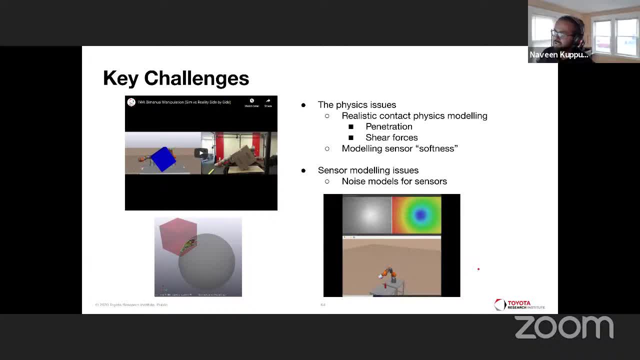 you're seeing a Drake-style simulation simulating the tactile perception of making contact with an object, And what it is is nothing but a depth camera inside a surface which is allowed to penetrate and touch this external surface. So simulating the depth part is quite straightforward. 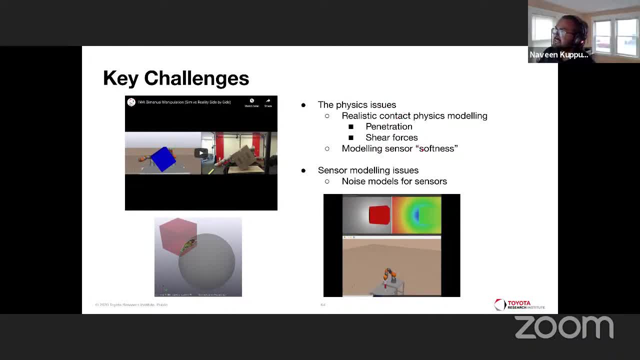 What is the hard part of this problem? Simulating the realistic contact physics, And we have. I know Russ has covered some of these questions earlier in this lecture, So essentially my answer to can you simulate a sensor is: can you get the contact physics right for your instance? 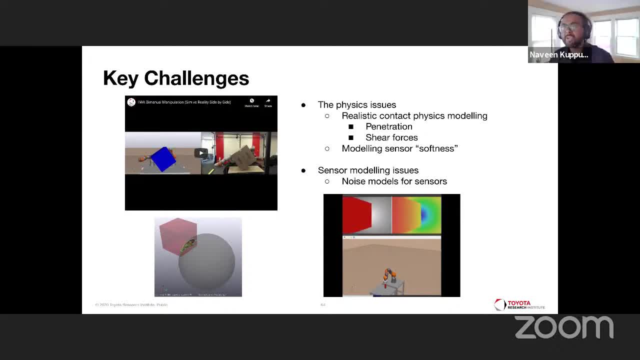 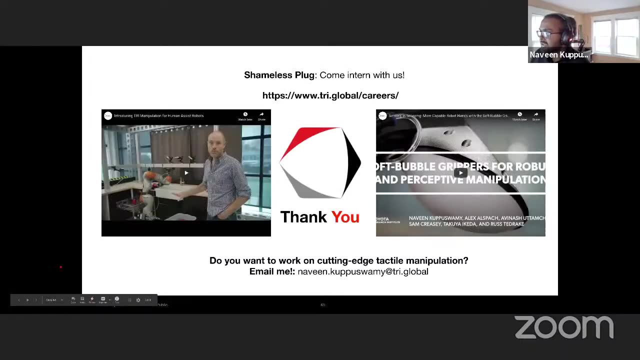 of tactile sensor And can you appropriately capture the noise model? If you can do these things, any tactile sensor is simulatable, And that is one of my key take home messages. So, since we are out of time and I just do want to have one or two quick questions towards the end, 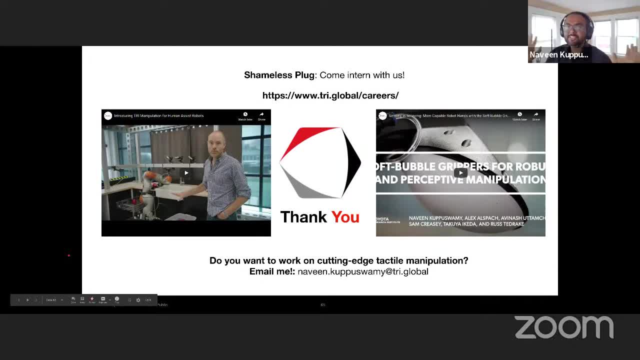 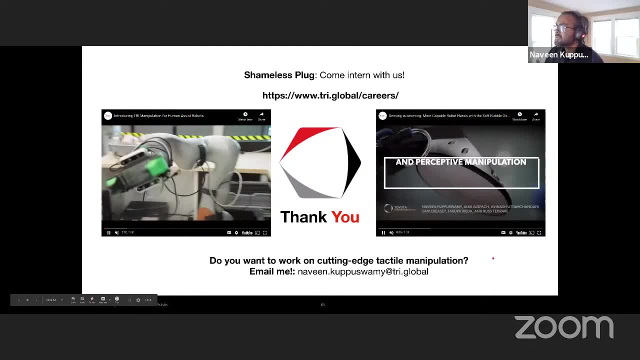 I want to ask you: OK, So shamelessly, throw a plug. we have internship positions open. There's a lot of material out there if you're interested in understanding what TRI has been up to. And while we are discussing that, I'll leave our video on the soft bubble grippers. 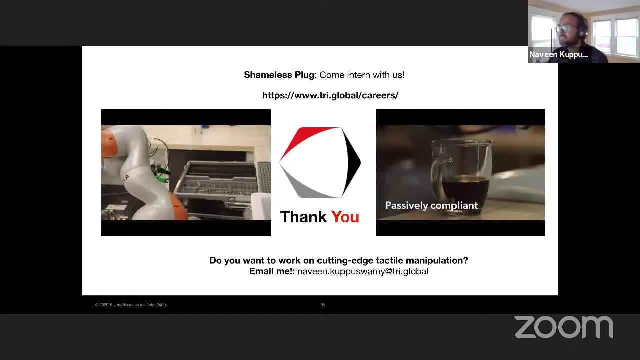 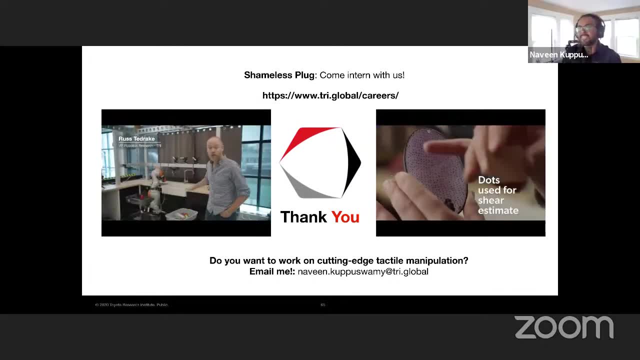 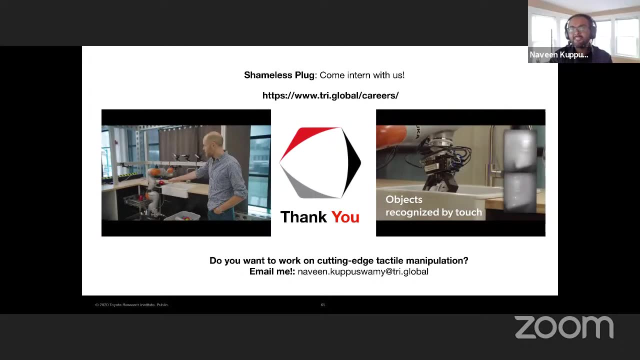 And do email me if you're interested in working on problems on tactile perception. But unfortunately that's it for today. Any other questions? Thank you so much. Thank you, Naveen. Thank you, I have a question, Or I was going to ask. so most of the sensors you talked about? 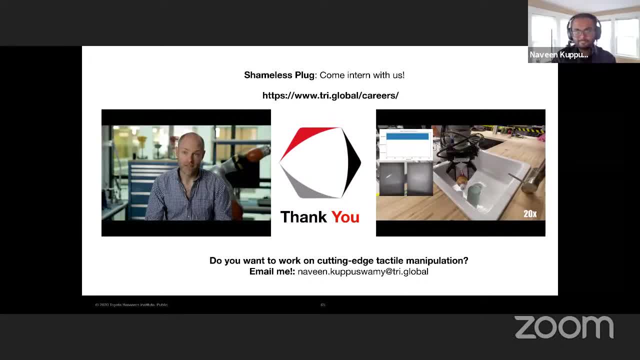 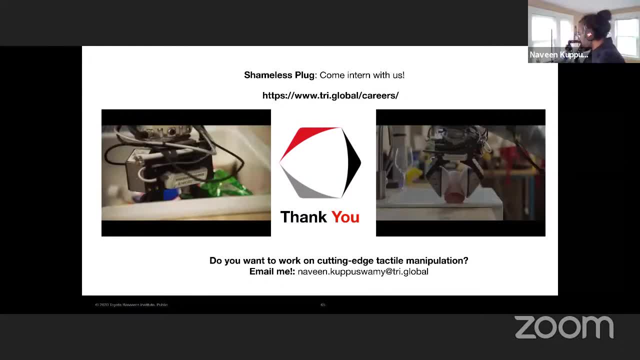 were vision-based? Do you find that the camera frame rate is ever a limitation for problems you want to work on? Where I imagine for tactile you could do things at a much higher frame rate or a much higher sensing rate, There might be some sort of 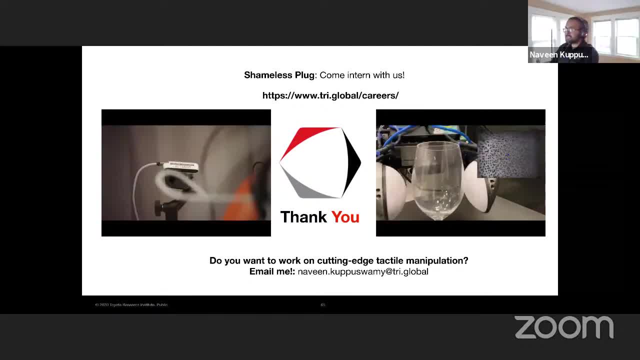 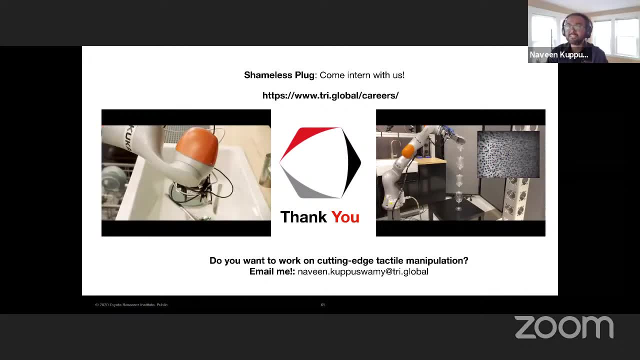 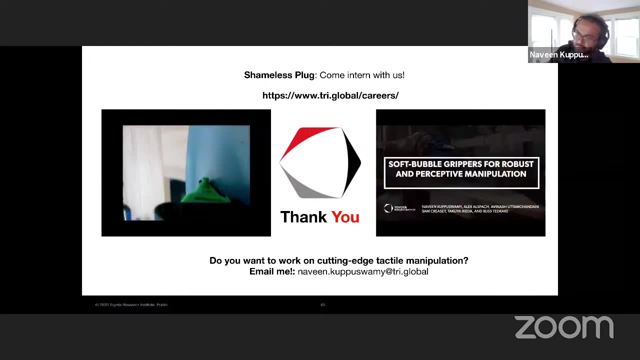 There are two answers to the question. Just like any other camera-based perception, if you want to do things faster, you can always try and look for a custom sensor which does things a lot faster, with a lot fewer pixels, for instance. So it may entirely depend on the nature of your problem. 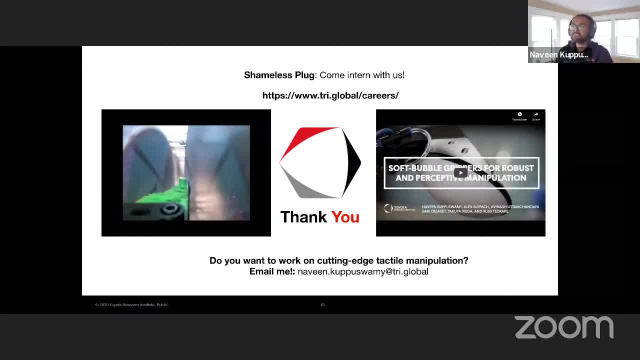 You could try and find yourself a custom imaging sensor which is not quite at the resolution you need for a whole scene, but at a much lower resolution can sample a lot faster. You also have some tactile sensory work out there where they embed even driven cameras or dynamic vision sensors. 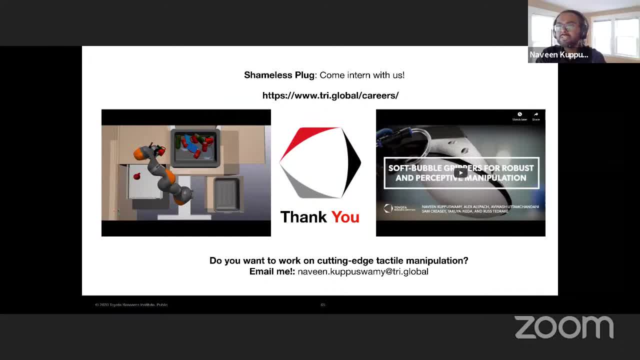 into the scene. If any of you are familiar with these kind of sensors, people have tried to embed them into these kind of sensors too, And that captures a lot of phenomenon. But I'd also like to emphasize: putting a camera inside sensors is not the be-all and end-all. 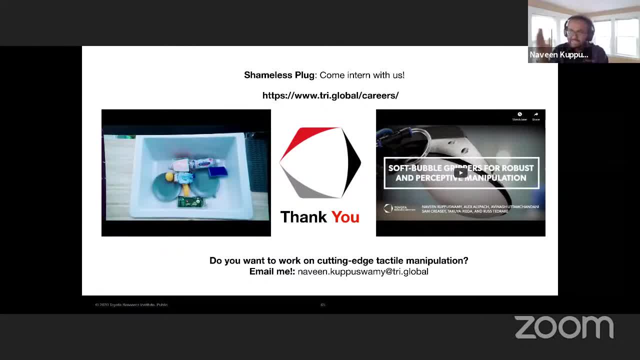 It's a very good solution for certain kinds of perception. Perhaps you want to work really fast. You don't need a camera inside the sensor, You simply want to sense something much faster, which is the vibrations which could be sensed through acoustic techniques which could be sensed. 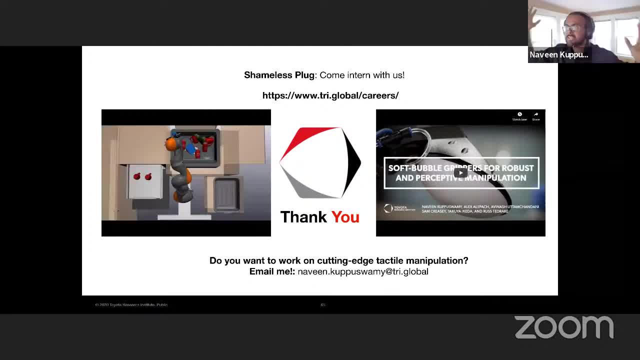 through accelerometers and so on. So a simple example is: stick a microphone in your sensor. You're going to sense things really fast, for instance impulses or the sensation of dragging your finger over the surface. Cool, Thank you, You're welcome. 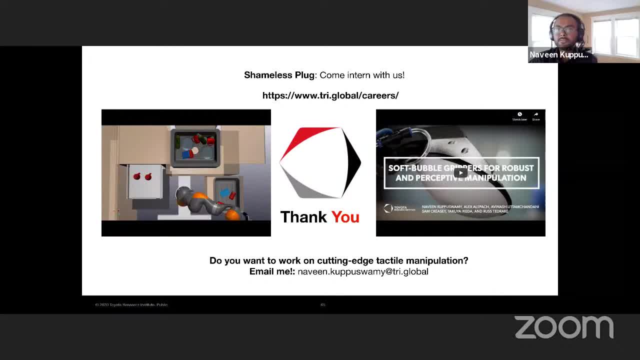 It's super interesting, right? One of the common things that I've heard you say and I've heard other people say is that if you're trying to wait for the onset or detect the onset of slip, if something's going to slip out of your hands, 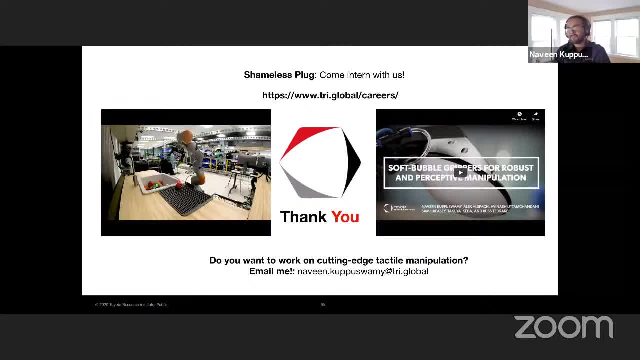 it's so hard to detect it And actually react to it in a time frame that would be useful. all right, I think that's a really acute place where the bandwidth question comes in And it's a closed loop question, really right. 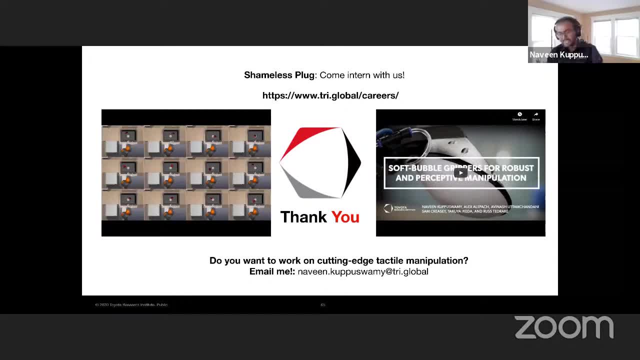 Even if you could sense it, could you react fast enough, Right, In fact, with a paddle gripper, what can you do? You can just jam harder and hope that your normal forces are sufficient to prevent slippage happening, Right? 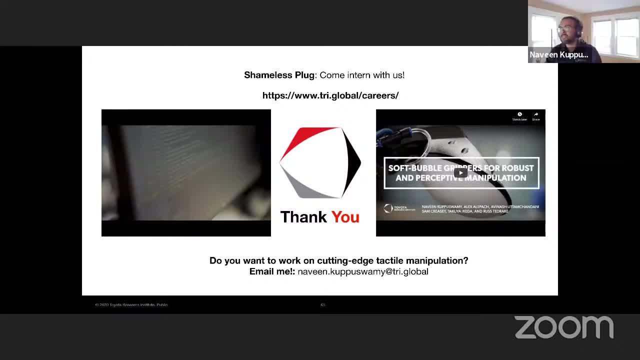 Yeah, That's even in that simple example. closing the loop to jam harder is really tricky Because a lot of times slip is a phenomenon which happens so fast And at best you can only tell that slippage happened. And coping with it fast is a tricky challenge. 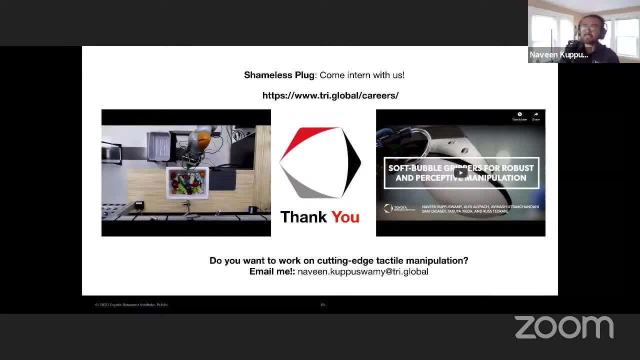 So there are some times when you could intentionally control slip- For instance, letting an object rotate between your fingers- And that might be a feasible way to utilize slip sensing rather than just coping with slip and trying to grab it and hope that you haven't completely. 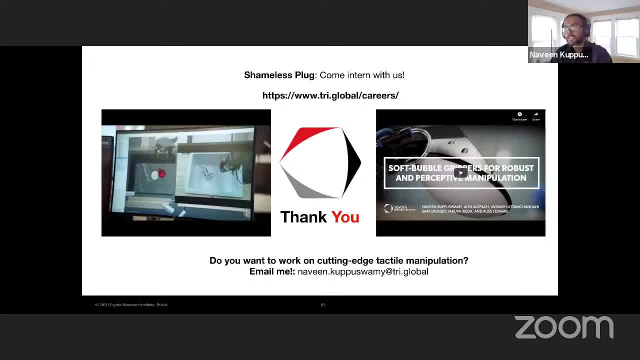 let go of the object. Are there any other questions? I'm just going to flip through your faces. So you showed some examples of using force feedback for control. Do you ever think about using tactile localization and estimating the pose of the object in a control framework? 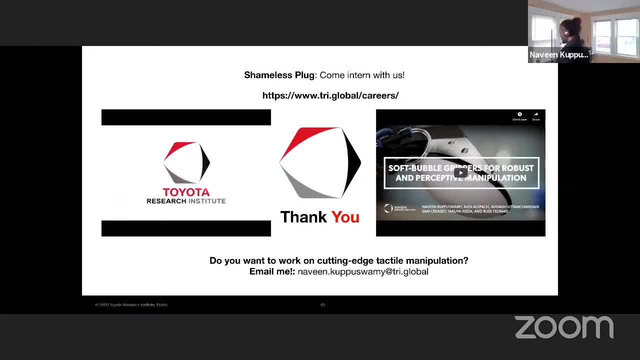 Or do you mainly do more reactive things, like with forces? So this is a good question. I think it's a good question. I think it's a good question, A really good question. There are two ways in which you want to think about it. 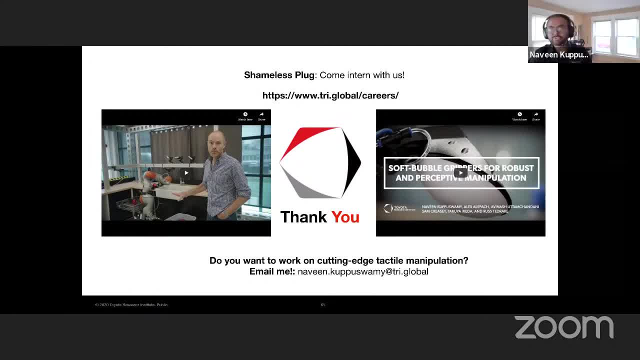 If you expect the pose will change and you want to cope for the pose change as you're manipulating an object, so when it is in contact, you would be actually trying to write a feedback controller using tactile pose. Now more often than not, especially 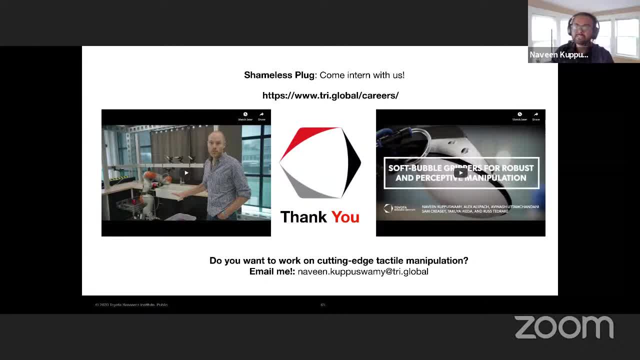 in these parallel gripper examples where you're picking and placing in a complex scene, the pose change is a resultant of an unexpected contact, So it's more like It's more like you actually want to cope with something unexpected happening rather than actively control. 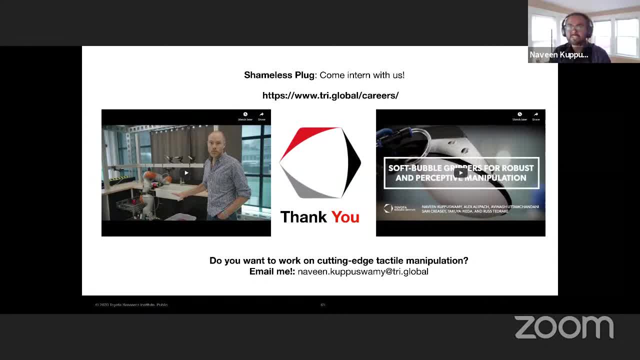 Now an active control example might be closer to what I just said with the slippage. Maybe you want to have control slip and keep looking at the object while you're letting it slip or slide between your fingers. Now again, my gut feeling about this problem. 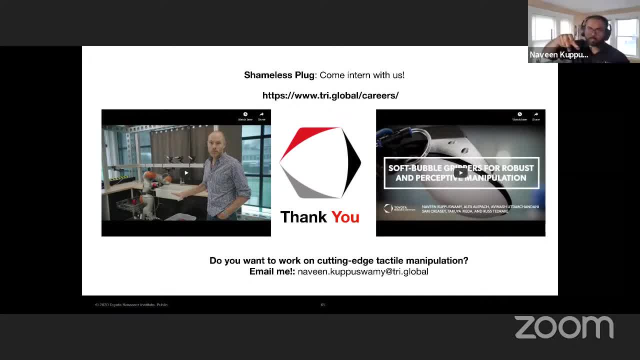 is perhaps trying to use a tactile sensor to control pose continuously may be the wrong kind of problem, But it doesn't mean it's a problem. It's not. It's the wrong problem for a behavioral level switching. You could, for instance, use the pose. 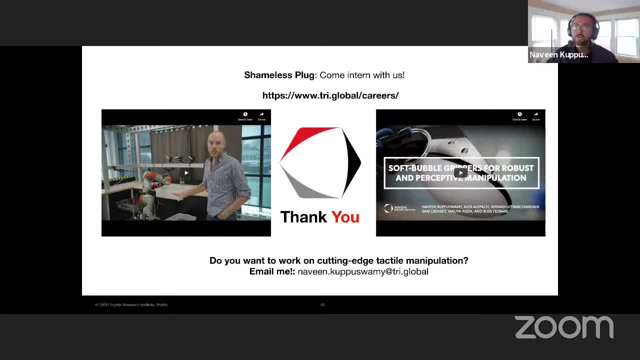 and perhaps change your robot's trajectory mid-flight on what you're performing. So I'd like to just slightly draw a distinction between behavioral level control and actually writing a feedback stabilized controller using the pose. So my non-answer is: it's really hard. 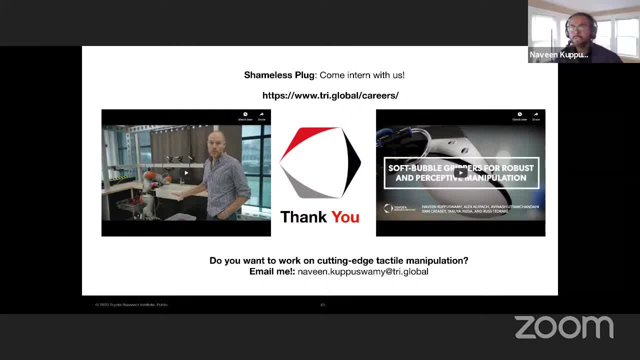 I would rather use the tactile sensor to cope with an unknown state or do behavioral switching, Thank you, Thank you, You're welcome. So I mean Tony who just asked, that is from Alberto's group, And so I guess, thinking about Nikhil's work, for instance, 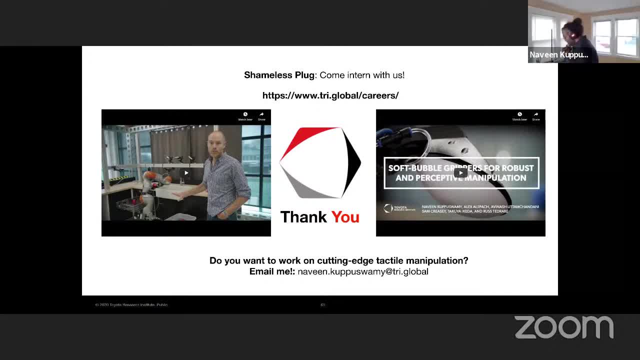 of the non-prehensile- I guess I haven't talked about it in lecture yet, but of moving the MIT around and then having a sorry, his is prehensile in that case- but causing, like the in-hand, reorientations using world contact. 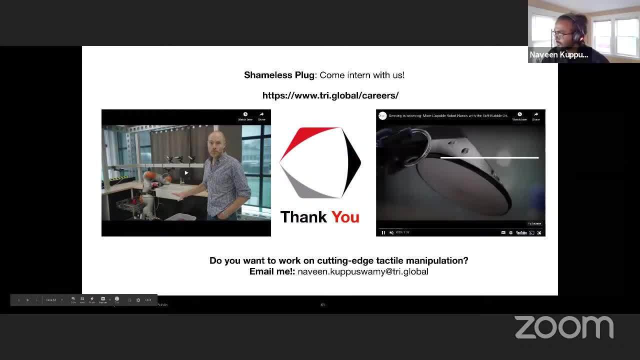 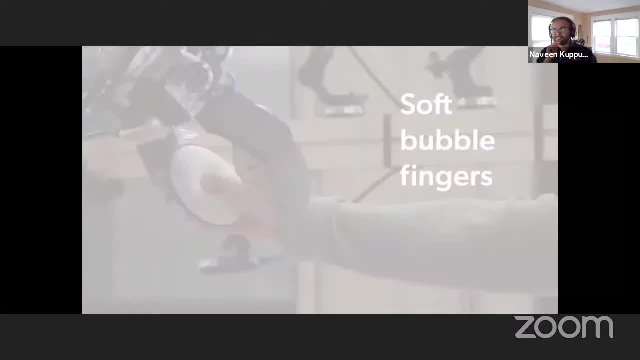 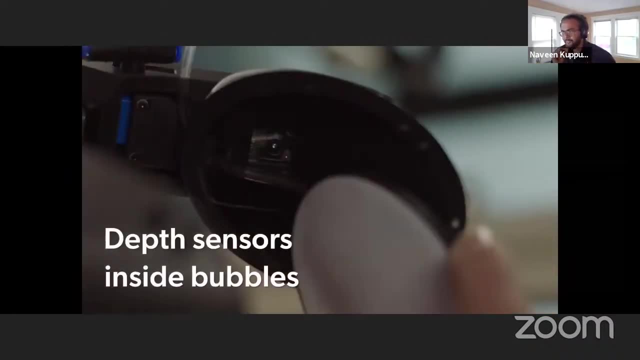 That seems like one case And we have. you have an example of reorienting a mug by making intentional contact with the world and tracking that in-hand reorientation with the pose estimate, tactile pose estimation right. Yes, So there are definitely cases where you could do it. 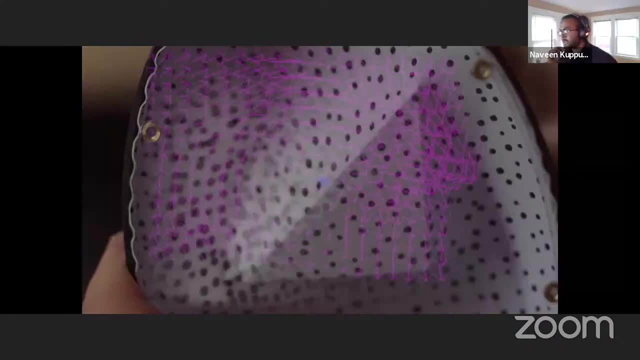 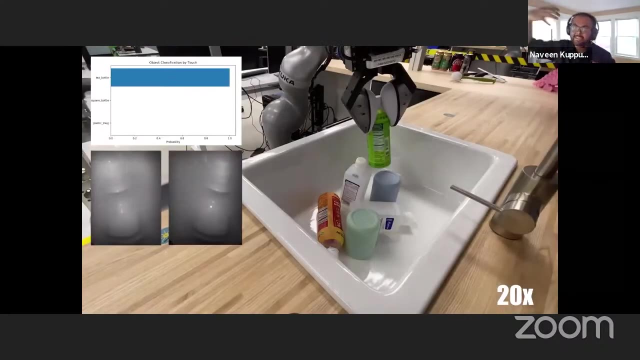 and would want to do it right. Yes, The only caveat I want to add Is your actual hardware behind the tactile sensor is a lot more complex. It's the entire gripper and the entire robot itself which is performing the control. 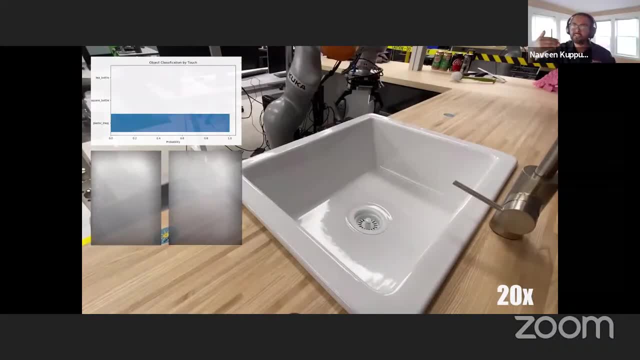 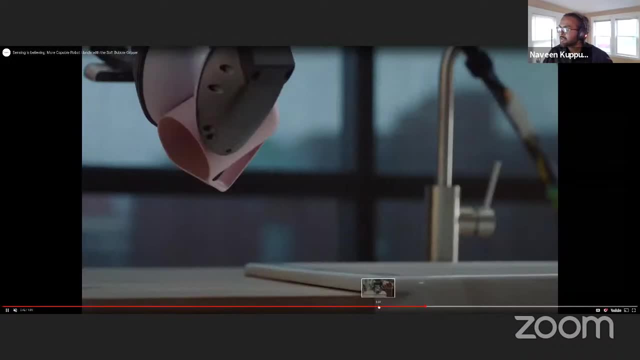 So if this entire chain is capable of reacting fast enough, that is the speed of reaction which you want to send. So this particular instance is exactly what Russ mentioned. So let me go back to this example. We are trying to flip this object, in this case. 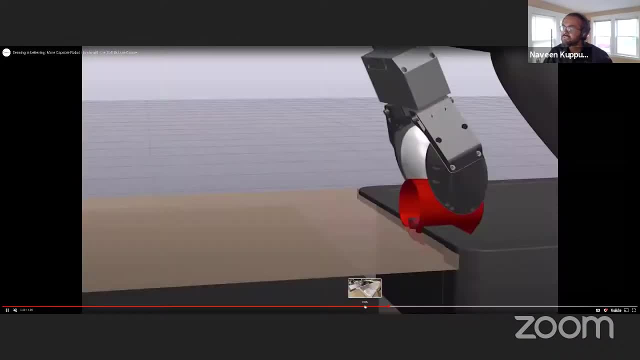 this mug by making intentional contact with the edge of this world. In this particular instance, the pose estimate is used to understand if it can indeed flip, And you can then come up with a plan which can then cause this flip to happen, perhaps. 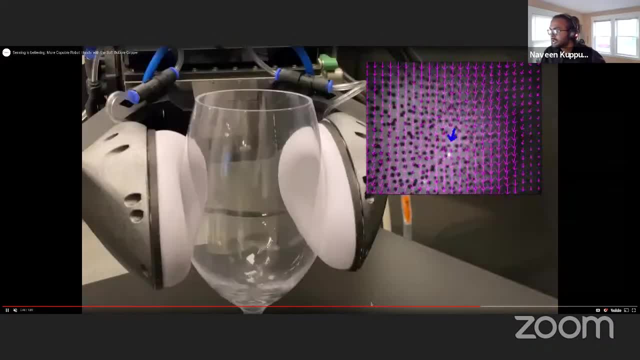 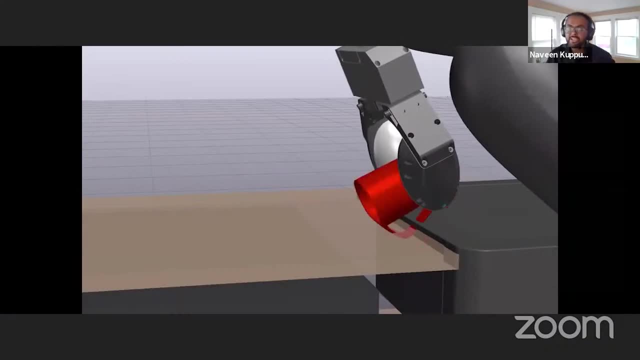 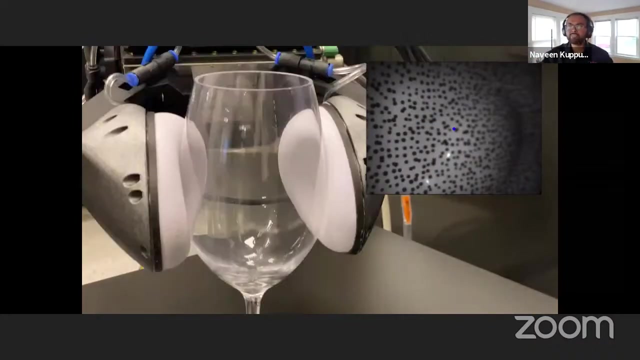 through Nichols work or so on. Now it is my feeling that you could write this as a pose feedback problem and try and speed up this pose estimation problem. The obvious trick I would throw at this is downsample and therefore let your pose estimator run way faster than normal. 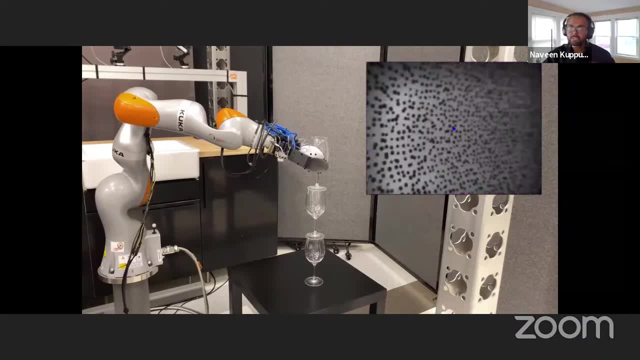 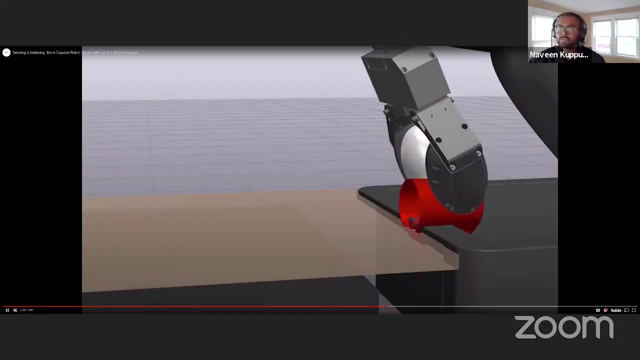 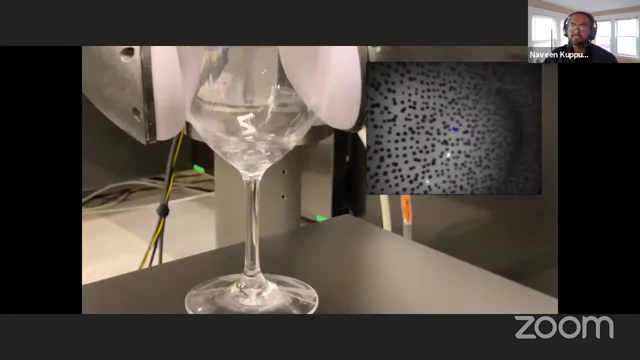 But still you would be limited to the peak frequency of the camera in your pose estimates And I think slowing it down, slowing the task itself down, is one obvious way in which we can actually write a feedback controller which uses pose. In this particular instance it's more a behavioral level. 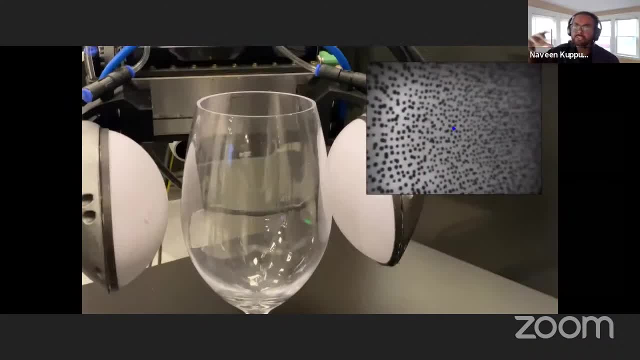 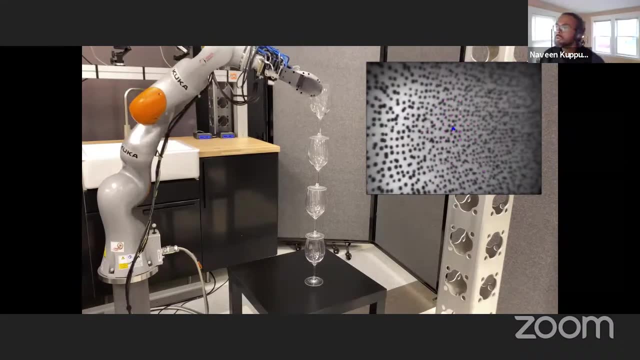 flipping. What I did was to query the pose, perform this action and, based on the pose in hand, slightly change the trajectory in which I was placing the object down on the surface. So again, my answer is I'm not sure. 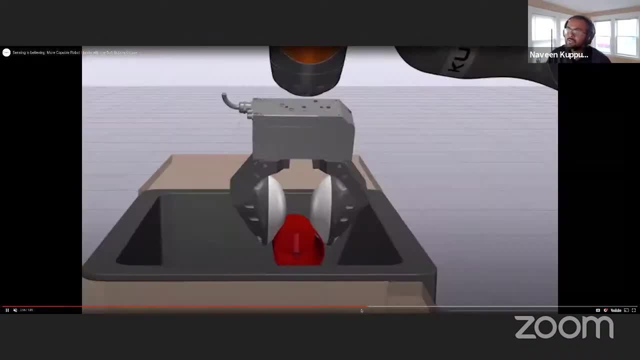 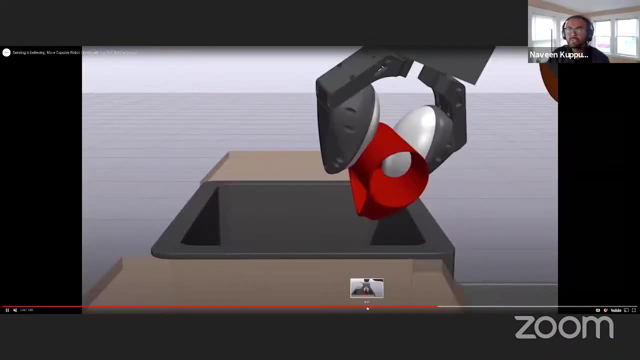 The answer is there are tricks in play where we can write a feedback controller with pose, And all those tricks require basically trying your best to speed up the sensory information. The control part is, of course, limited by your control bandwidth in this particular problem. 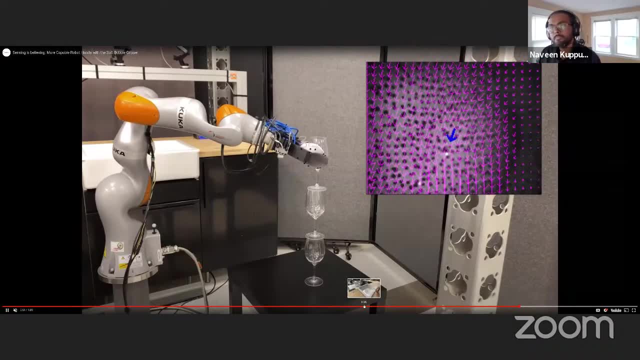 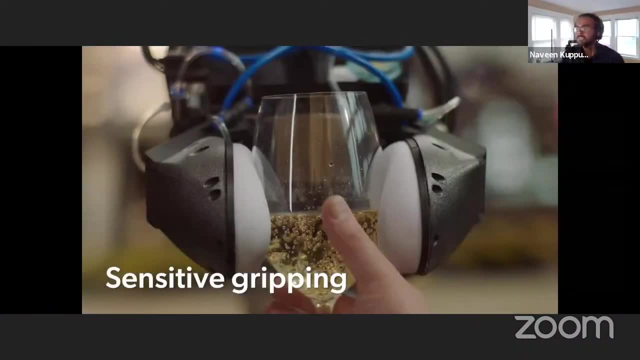 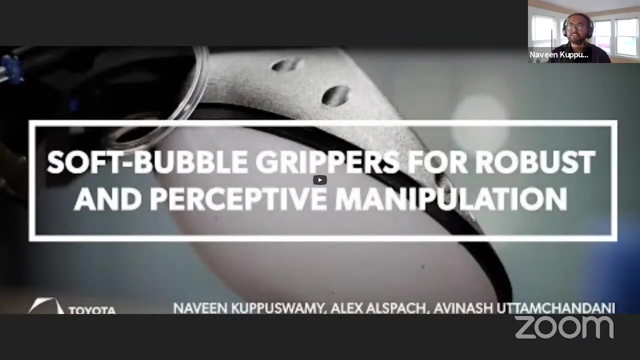 But it's doable. It's not impossible. I do like to think more about forces than pure pose, simply because force is something I often like to imagine. You can't directly obtain from a camera. You can infer it. You can know something about the world. 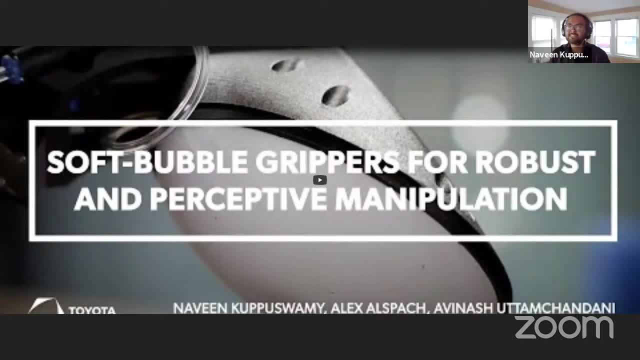 and use your pixels to guess force happen, whereas a tactile sensor sees force, And that's a huge distinction why I like to think about force-based problems rather than purely geometric-based problems. I guess, on a related note, what do you think about force-torque sensors, which is just 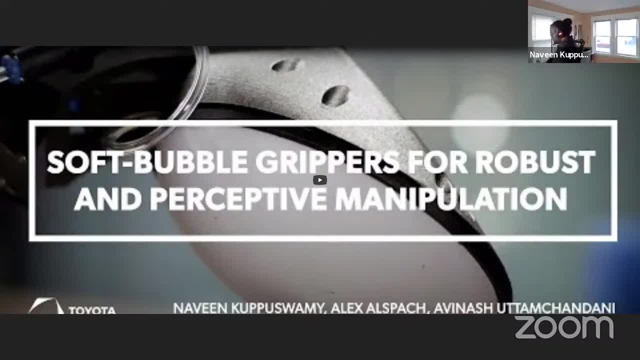 like one data point related to the force and the torque versus distributed. I think that's a great question.